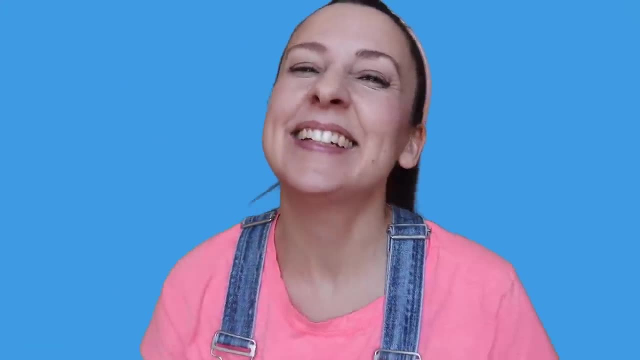 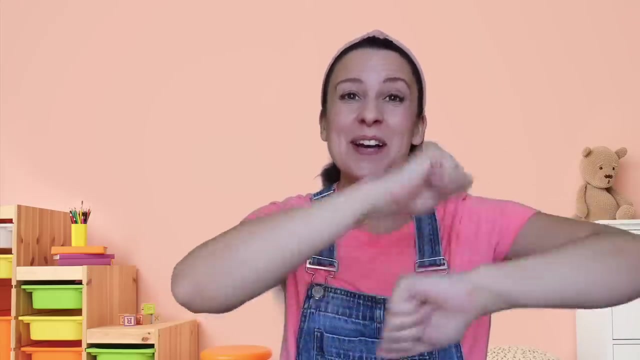 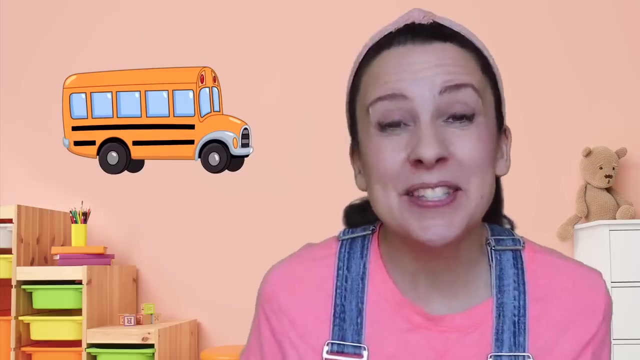 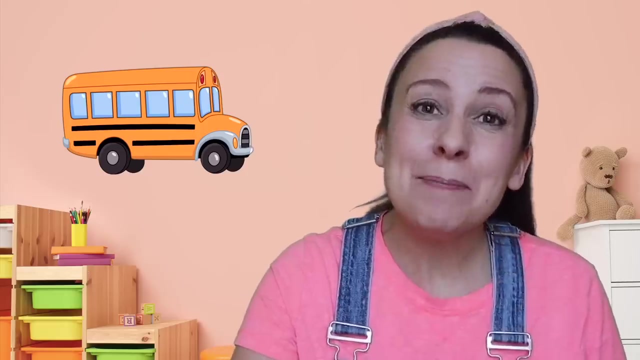 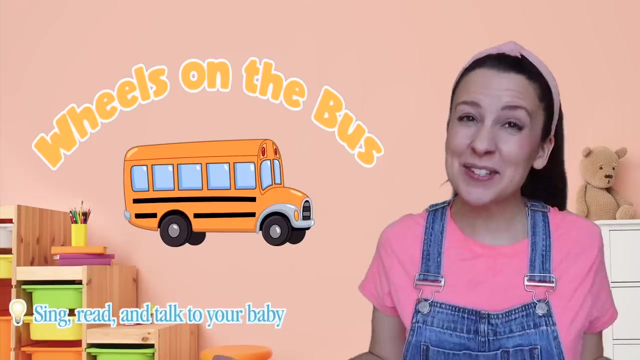 Da-da, Da-da, Good job, Can you do this? Do this and a bus will come out. A bus, Good job. Can you say beep-beep, Say beep-beep, and maybe the bus will beep. Beep-beep, Beep-beep, The bus beeped. Let's sing the wheels on the bus. 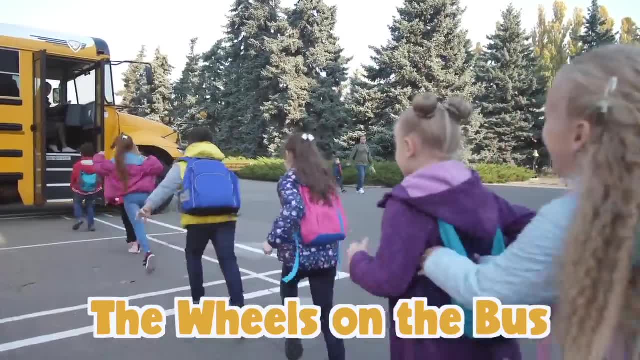 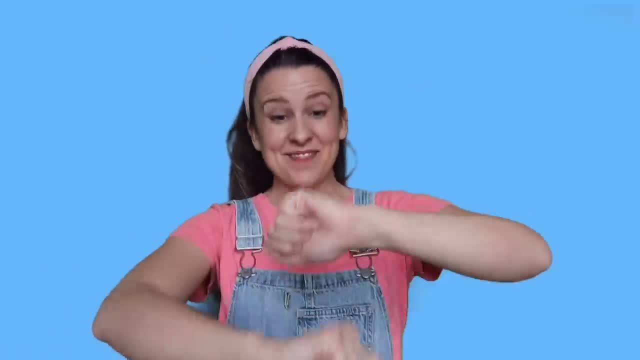 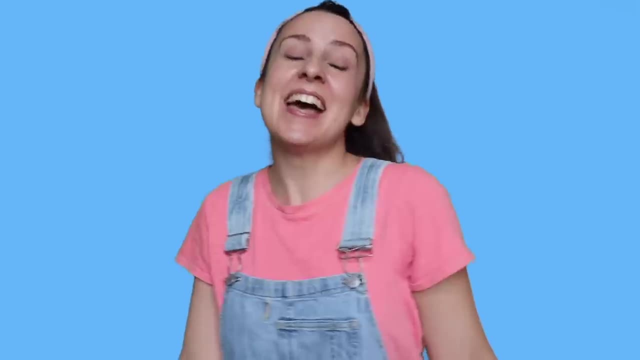 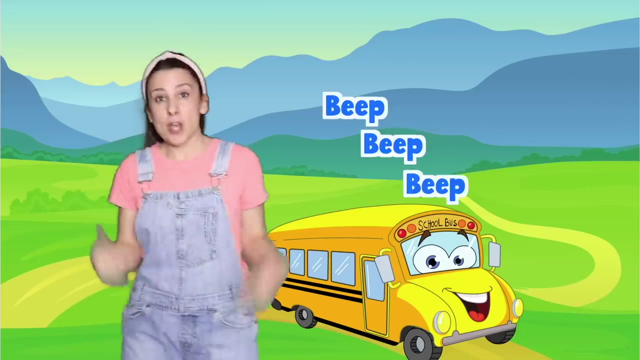 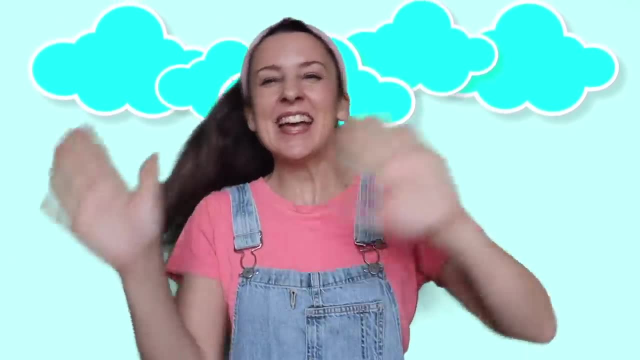 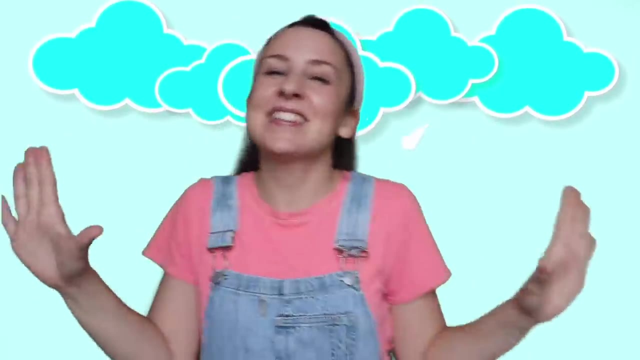 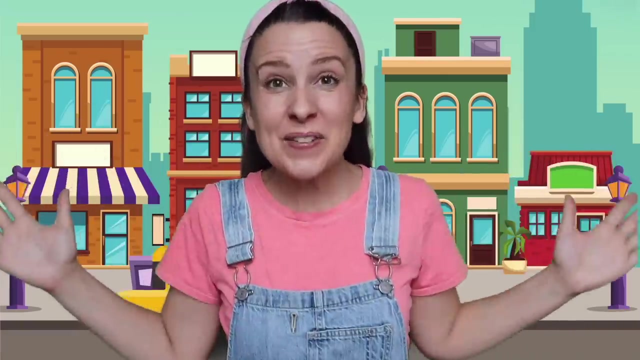 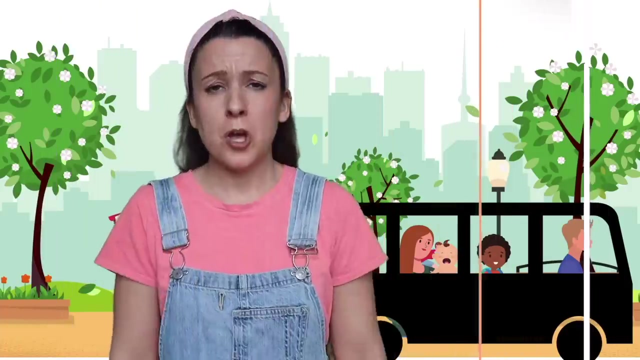 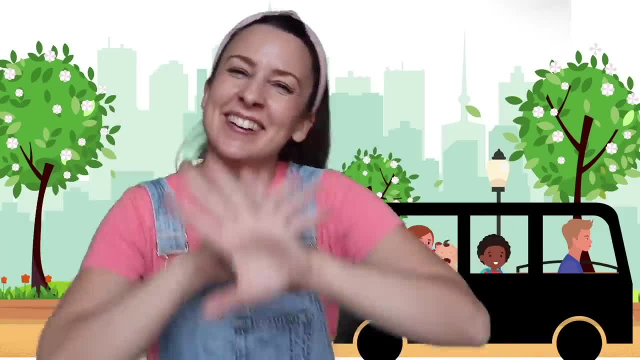 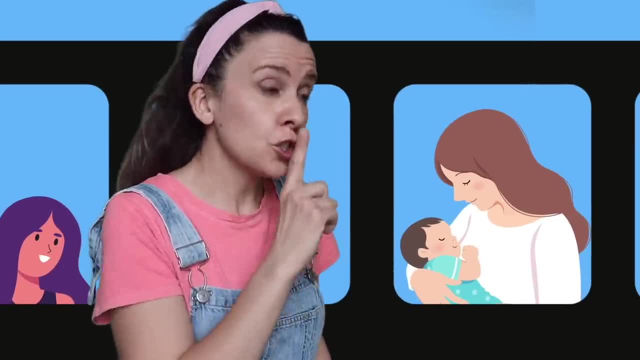 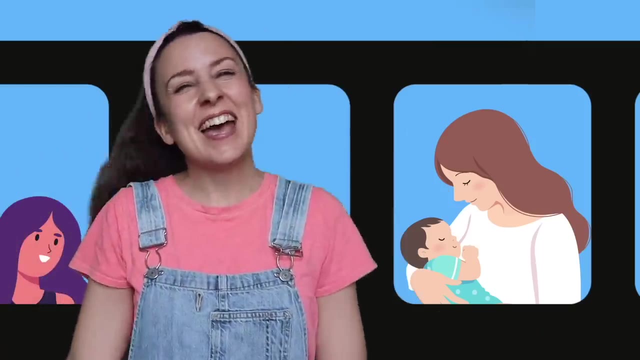 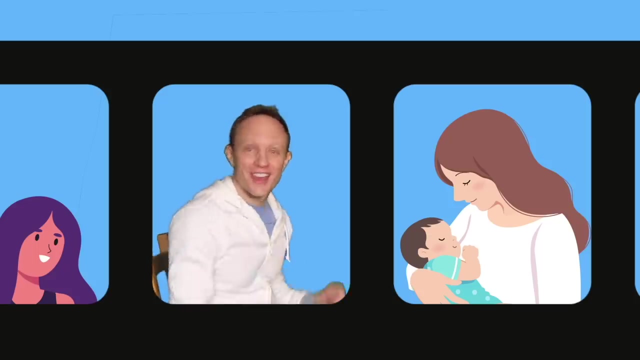 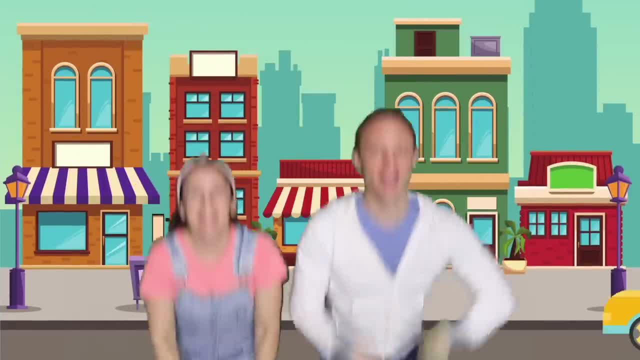 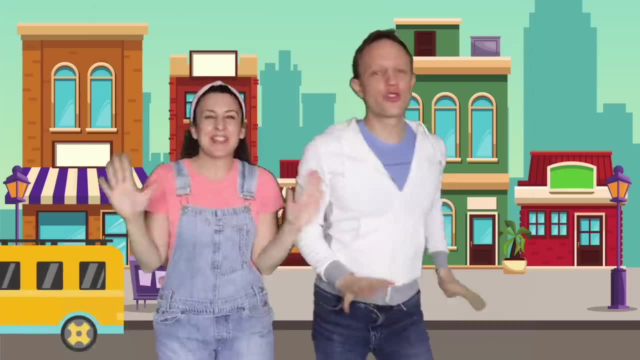 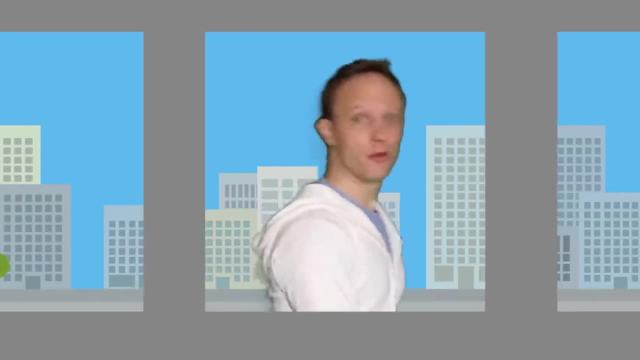 The people on the bus go up and down, Up and down, Up and down. The people on the bus go up and down All through the town. The driver on the bus says move on back, Move on back, Move on back. The driver on the bus says move on back. All through the town. 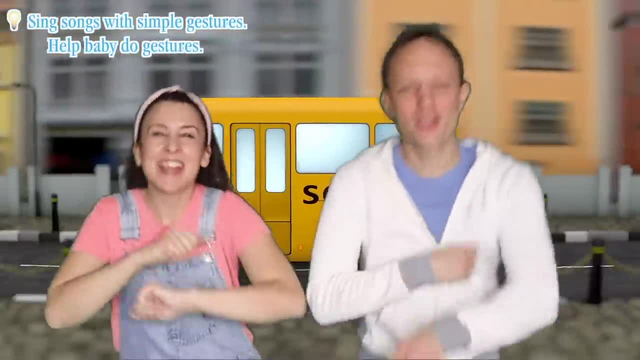 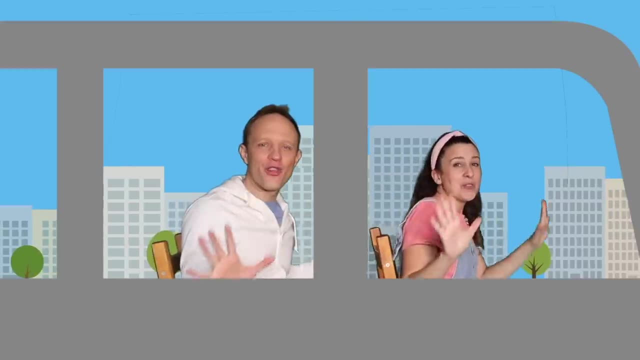 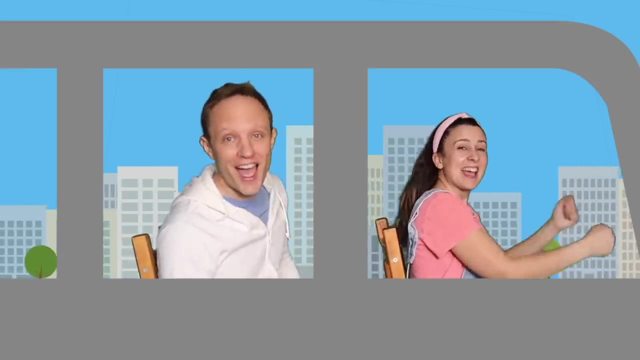 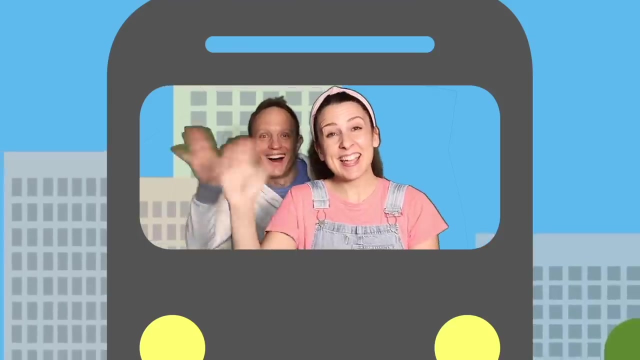 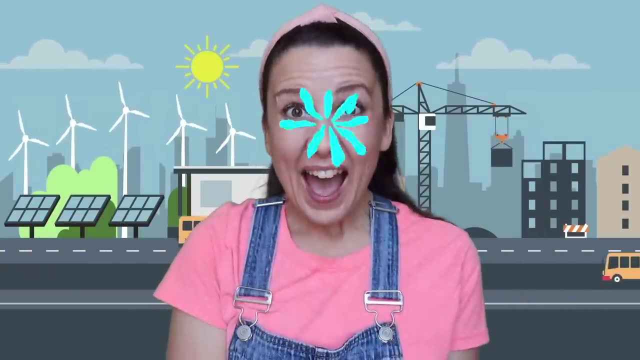 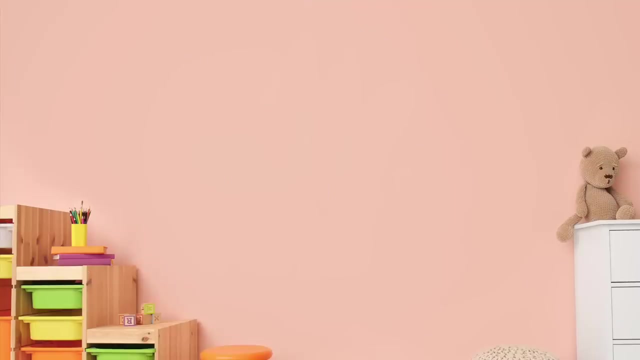 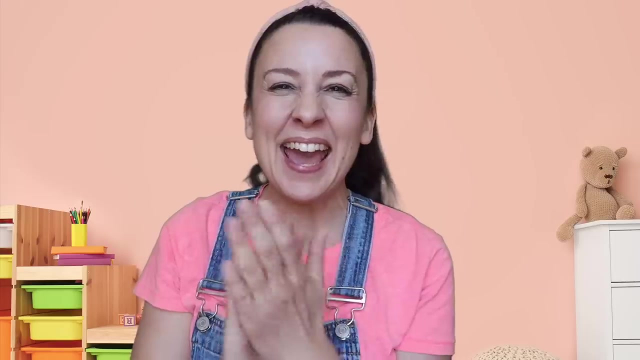 The wheels on the bus go round and round, Round and round, Round and round. The wheels on the bus go round and round, All through the town, All through the town, All through the town, Peek-a-boo, Peek-a-boo, Peek-a-boo, Peek-a-boo, Peek-a-boo, Yay. 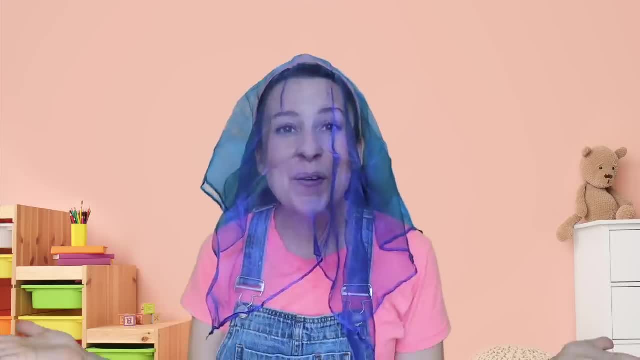 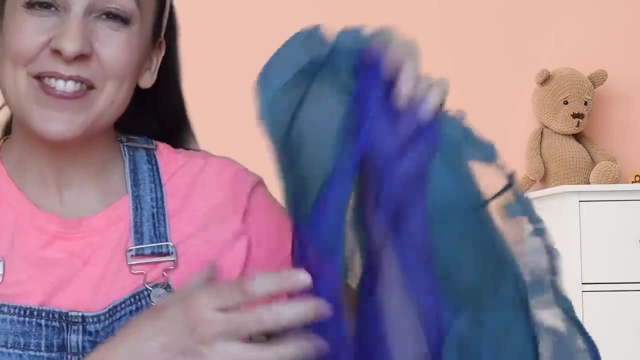 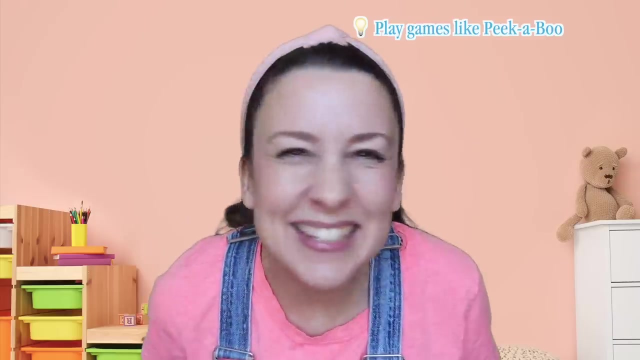 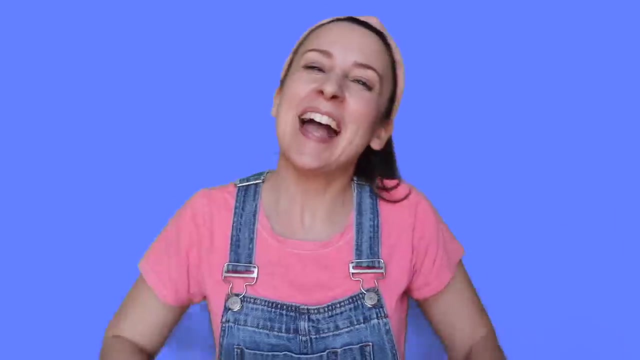 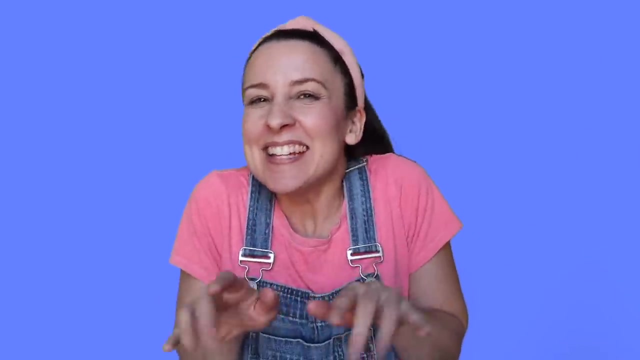 Where did I go? Peek-a-boo, I was under the scarf, Blue scarf. Where is Rachel? Where is Rachel? Peek-a-boo, I see you, Peek-a-boo, Peek-a-boo, I see you, I see you. I see your button nose. I see your tiny toes. Peek-a-boo, Peek-a-boo. 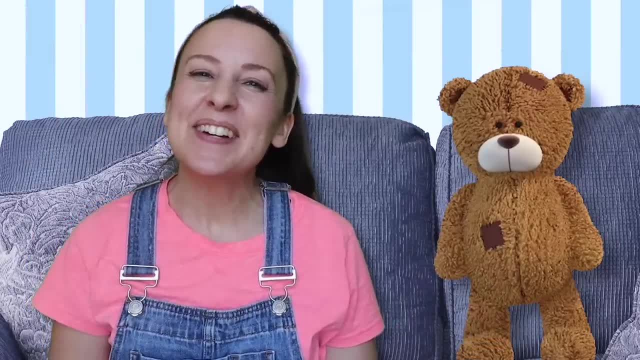 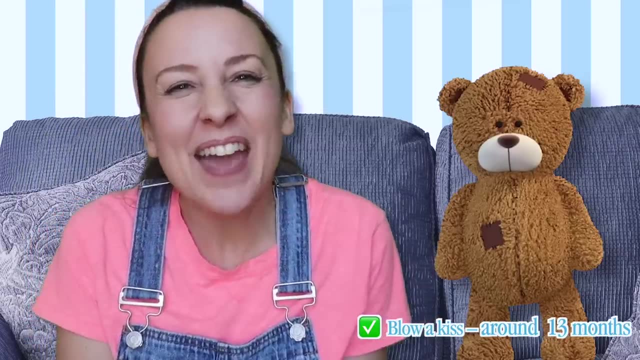 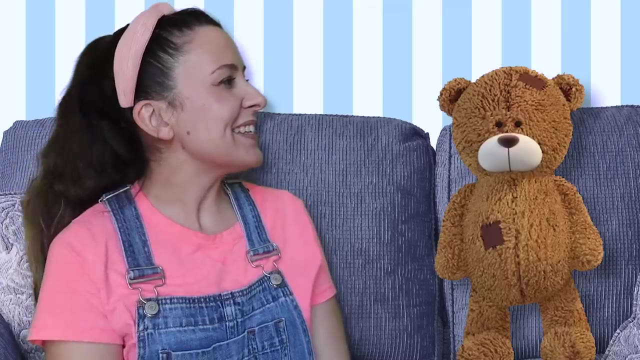 Can you blow a kiss? Blow a kiss. Maybe if we blow a kiss to the teddy bear, he'll give us a kiss back. Let's try it. Blow a kiss to the teddy bear and see what happens. Blow a kiss to the teddy bear. 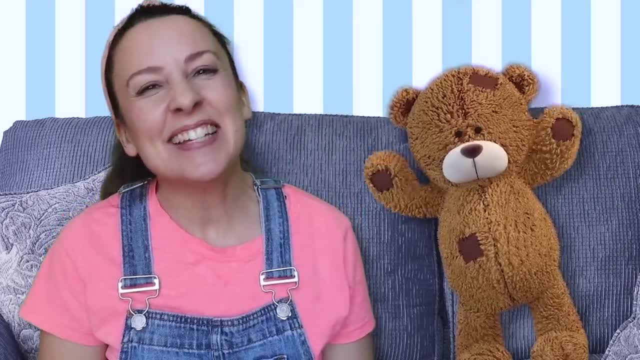 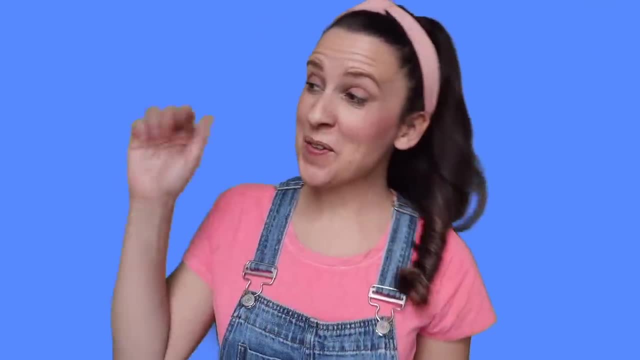 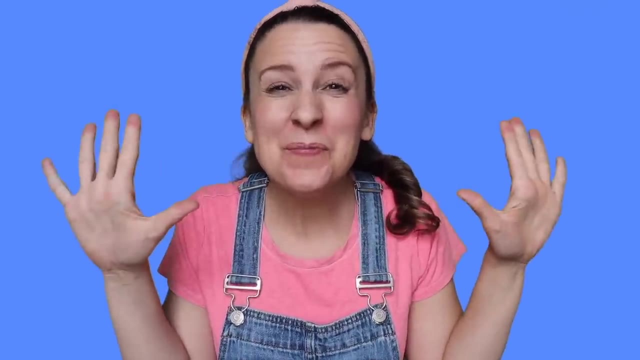 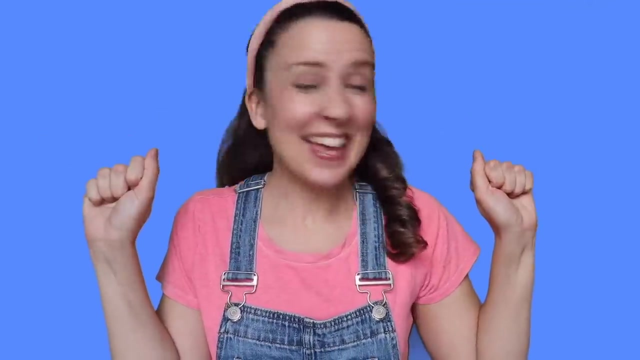 He gave us a kiss. He gave us a kiss back. Good job blowing a kiss. Can you get out your two hands, One, two, Open, shut them, Open, shut them. Give a little clap, clap, clap, Open, shut them, Open, shut them. Put them in your lap, lap, lap. 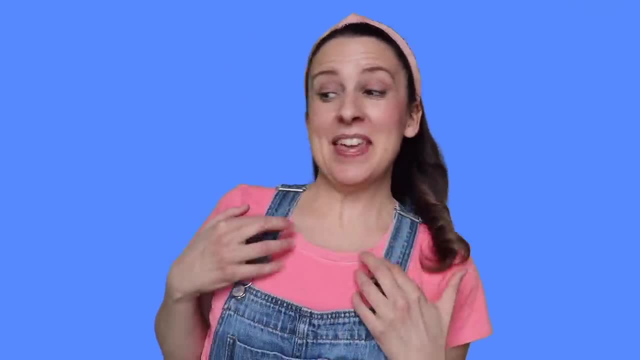 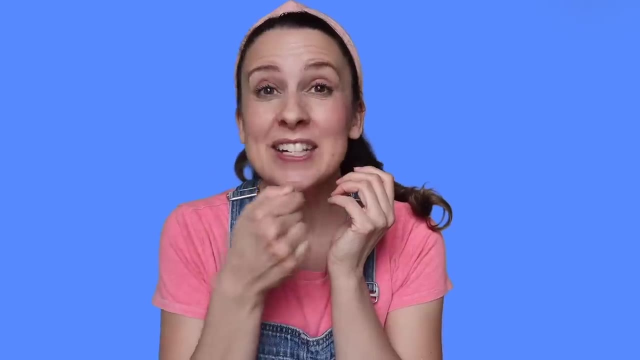 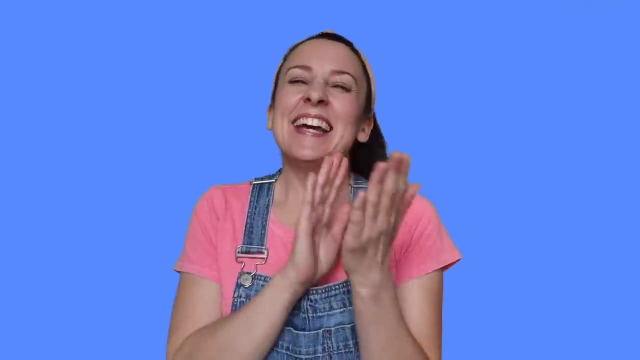 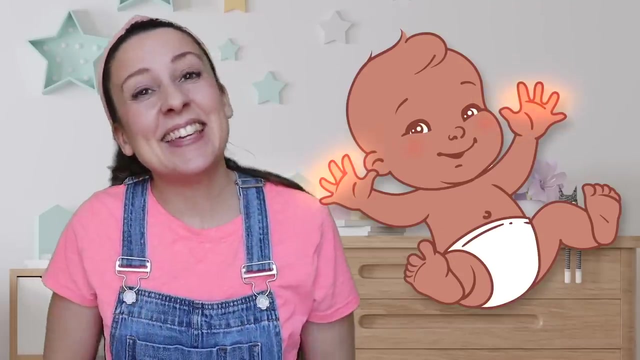 Creep them, crawl them, Creep them, crawl them Right up to your chin, chin, chin. Open wide your little mouth, But do not let them in. Great job, That was so much fun. These are baby's fingers, These are baby's toes, This is baby's belly button. Round and round it goes. 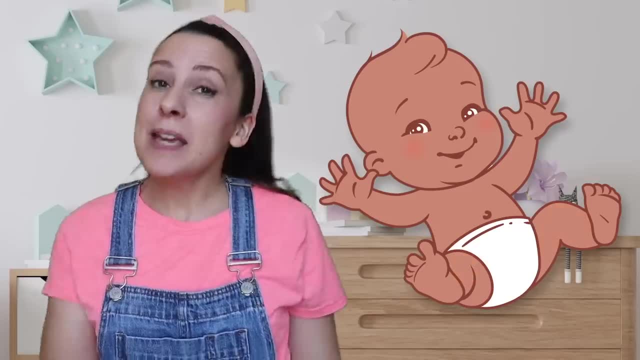 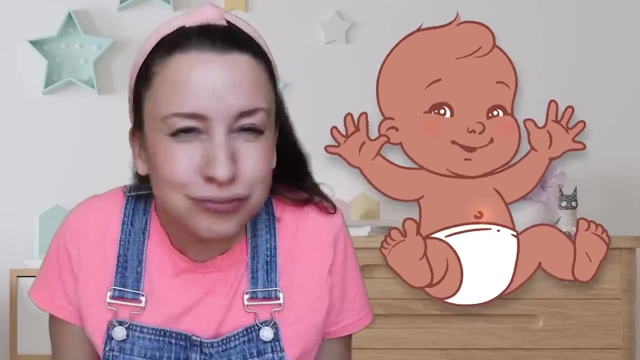 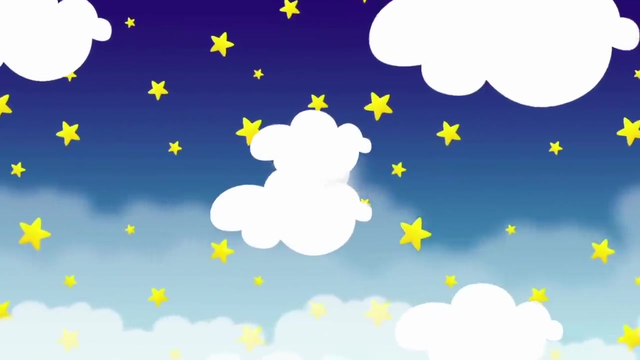 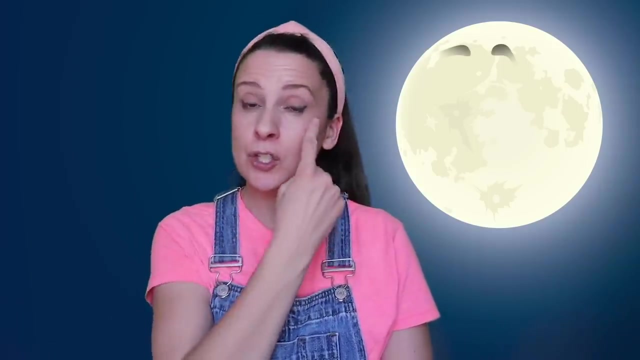 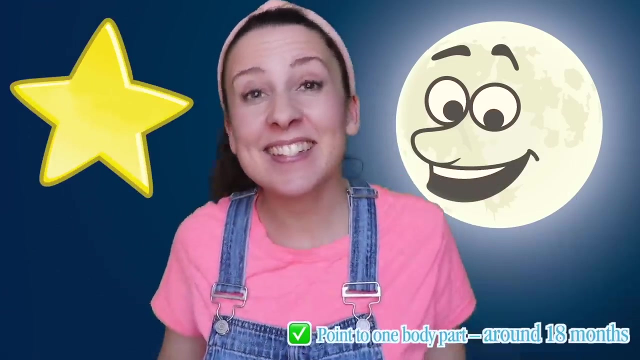 These are baby's knees And this is baby's nose And this is baby's belly button, where mommy blows So silly. The moon is round as round can be Two eyes, a nose and a mouth like me. Where are your eyes? 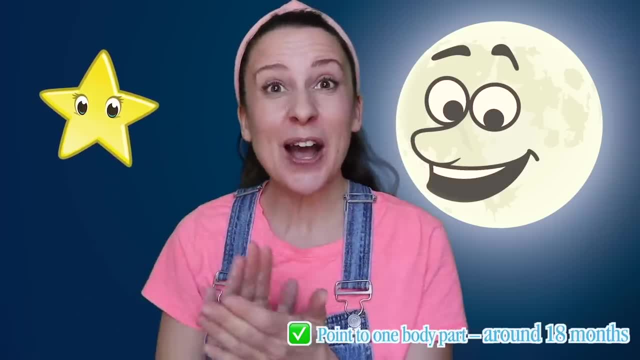 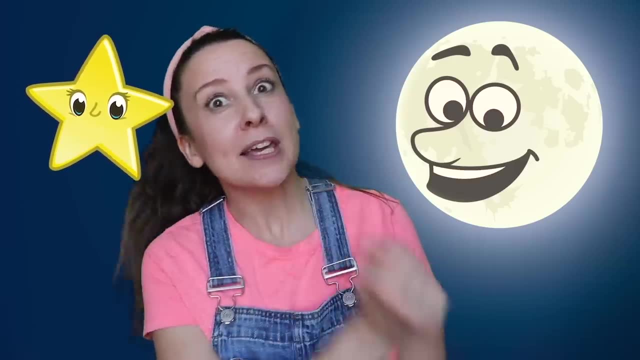 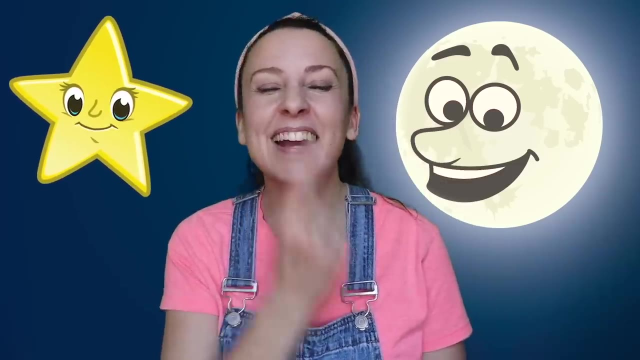 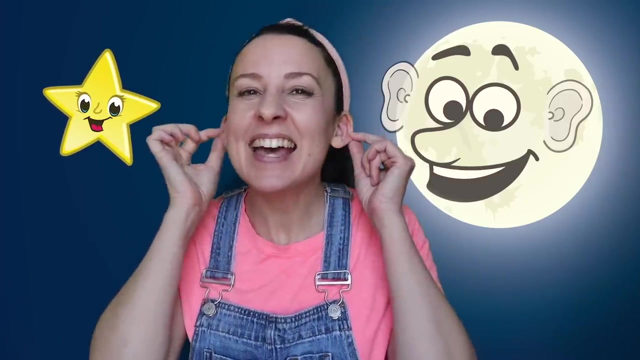 There they are, Good job. Where's your nose Boop? There, it is Beep Boink. We found our noses. Where is your mouth? Right here, Good job, Mouth. Where are your ears? Yeah, these are your ears, Ears- Good job. 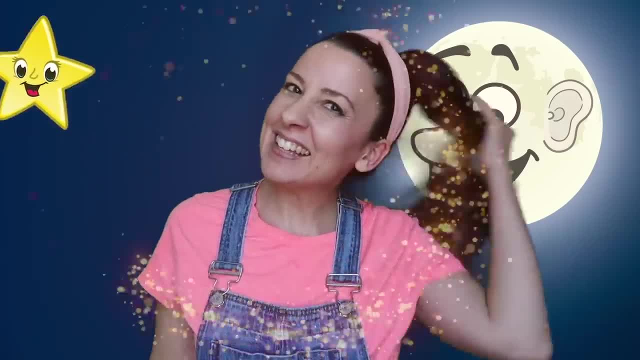 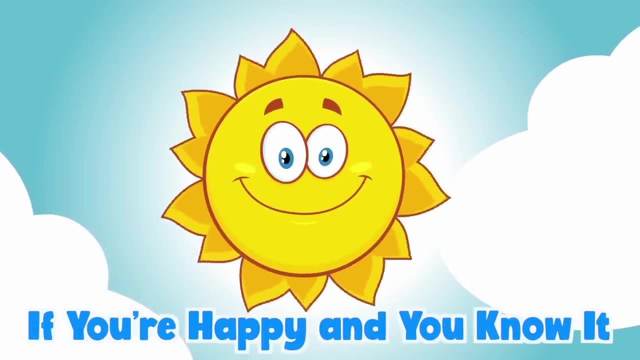 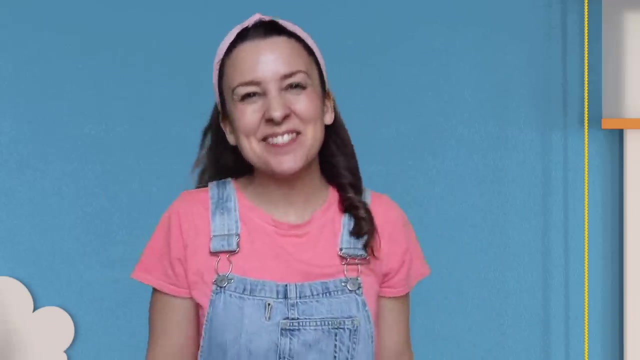 Where's you hair? Hummm, Yeah, this is our hair Hair. If you're happy and you know it, clap your hands. If you're happy and you know it, clap your hands. If you're happy and you know it and you really want to show it. 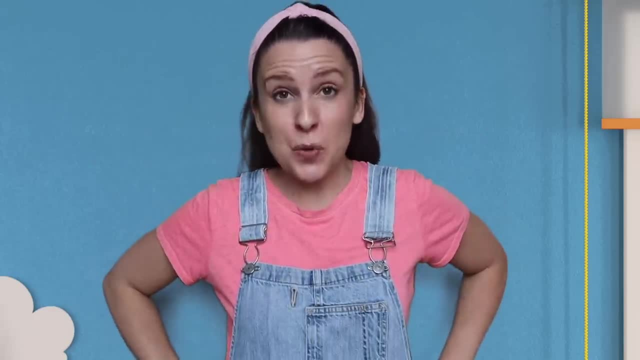 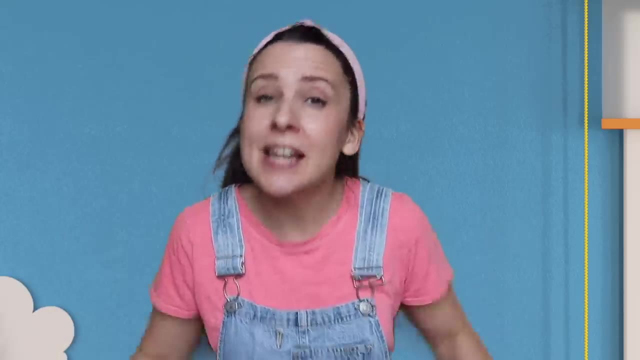 If you're happy and you know it, clap your hands and you know it, stomp your feet. If you're happy and you know it, stomp your feet. If you're happy and you know it and you really wanna show it. 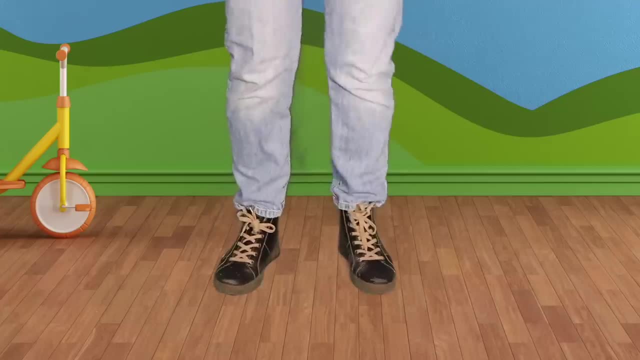 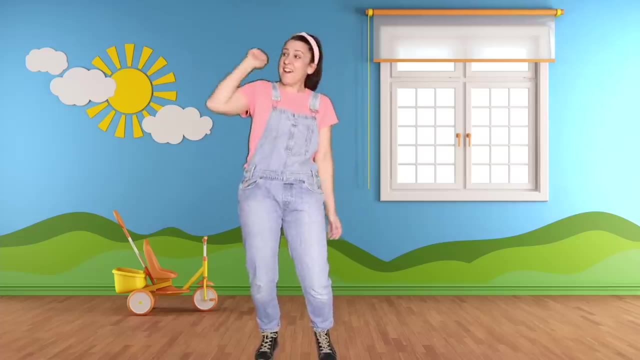 If you're happy and you know it, stomp your feet. If you're happy and you know it, shout hooray hooray. If you're happy and you know it, shout hooray hooray. If you're happy and you know it. 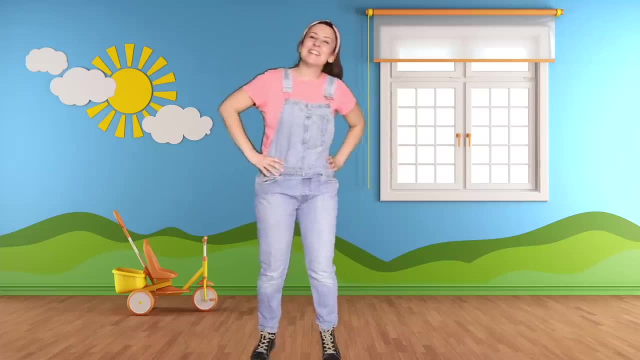 and you really wanna show it. If you're happy and you know it, shout hooray, hooray. If you're happy and you know it, do all three hooray. If you're happy and you know it, do all three hooray. 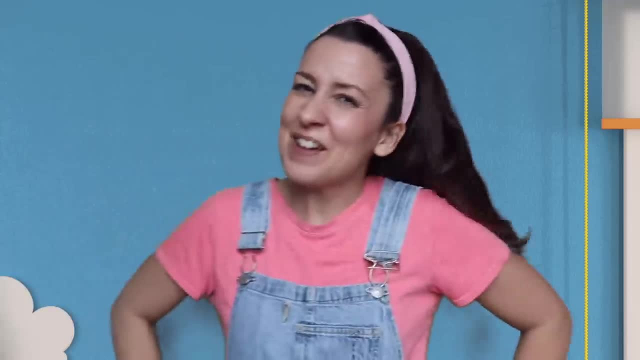 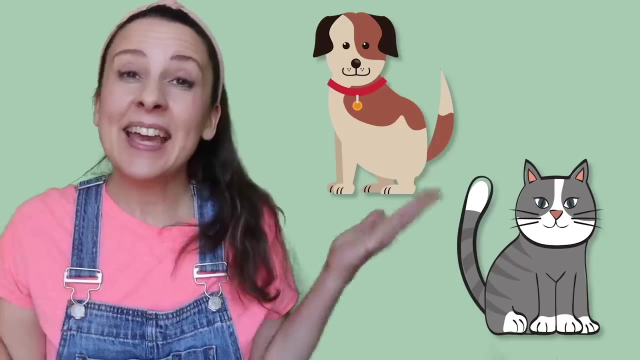 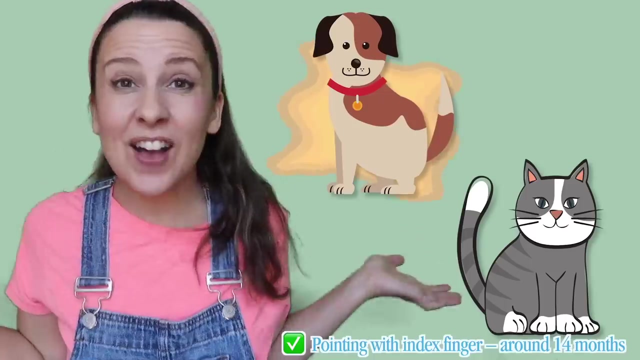 If you're happy and you know it, and you really wanna show it. If you're happy and you know it, do all three hooray. Can you point to the dog? Good job. What does a dog say? Woof, woof, woof, woof. 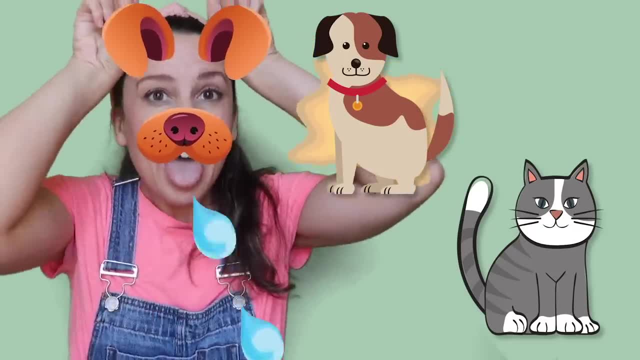 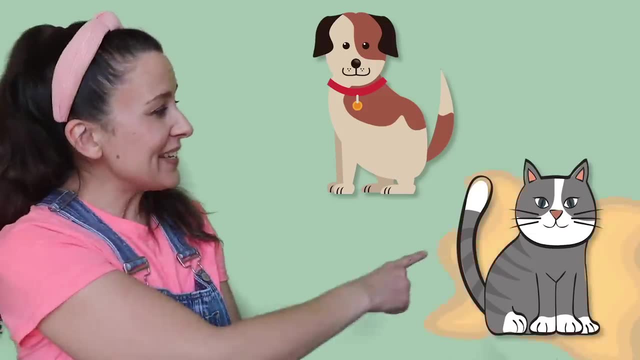 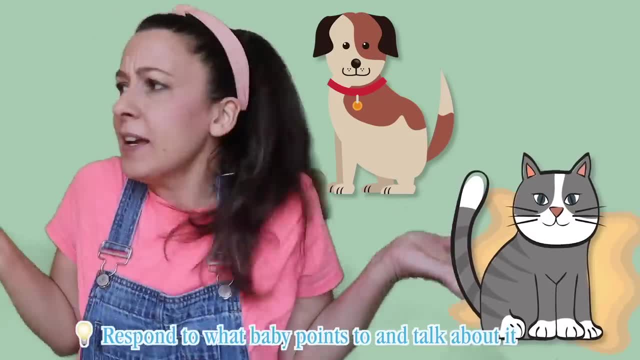 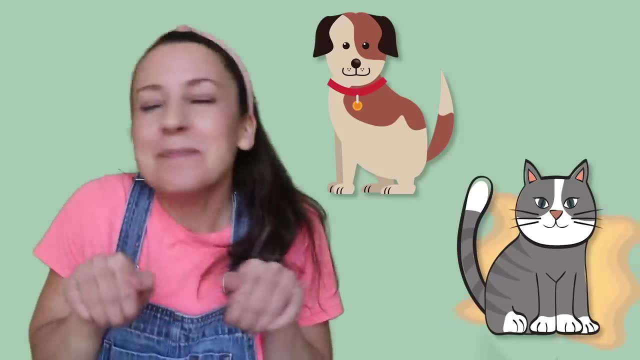 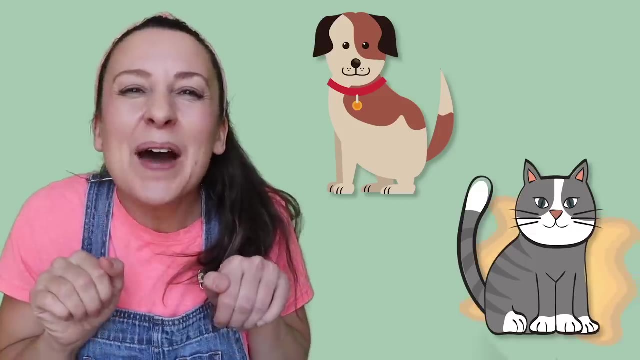 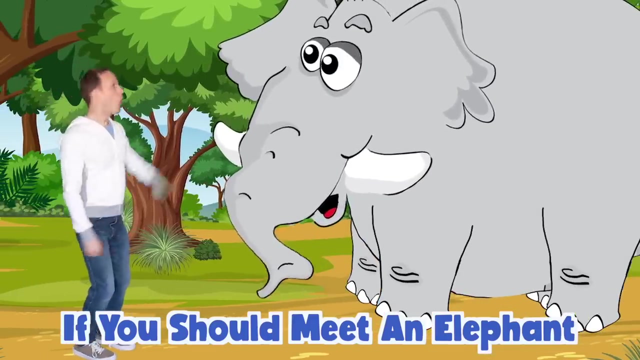 Pointing to the cat. What does a cat say? Yeah, meow, Let's pretend to be cats. Meow, meow, meow, Meow, meow, meow. Good job If you should meet an elephant upon a summer's day. 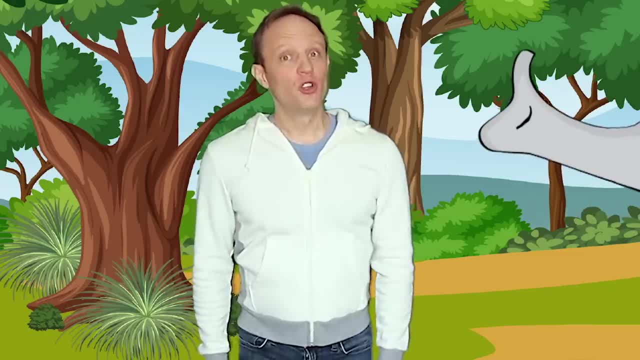 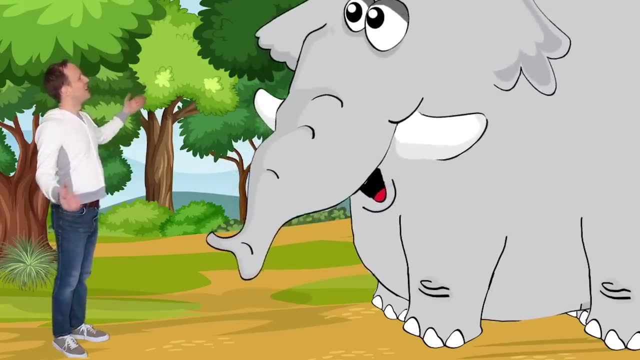 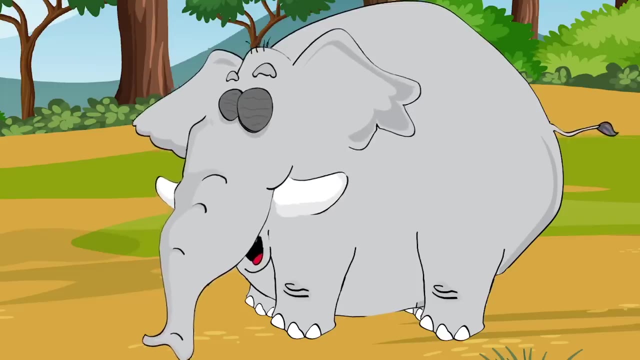 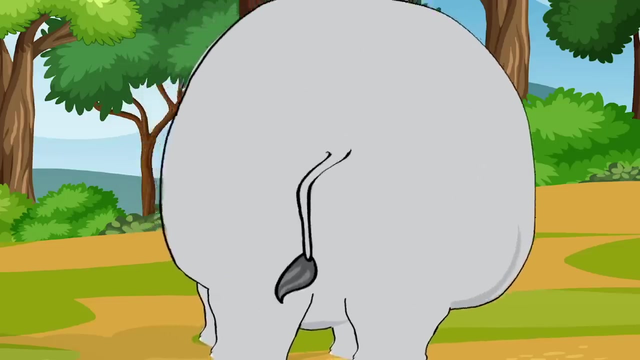 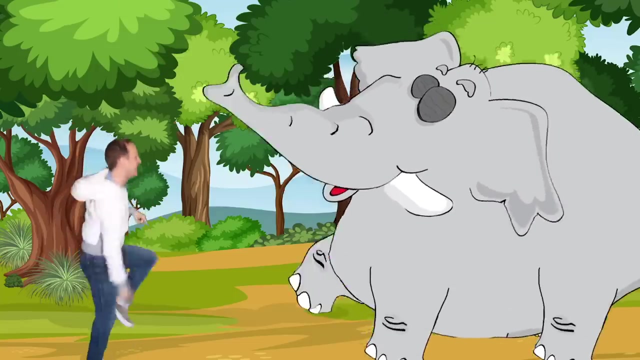 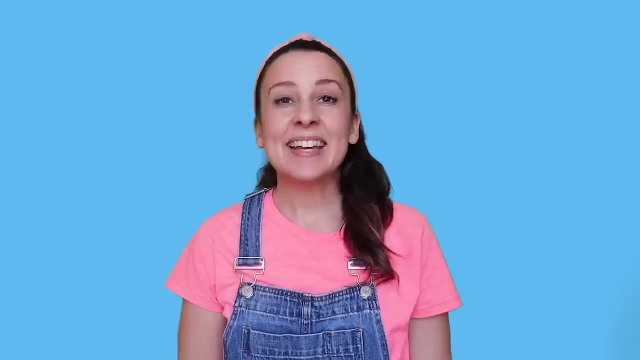 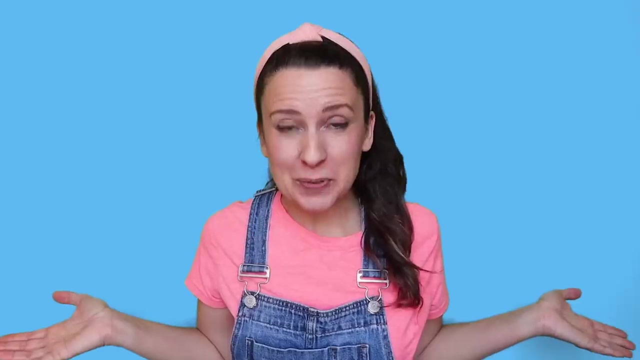 what would you do and what would you say? Say good morning elephant. How do you do? lovely morning elephant. May I dance with you? Tra, la, la, la, la. Can you say go, Go, say go, And some cars will. 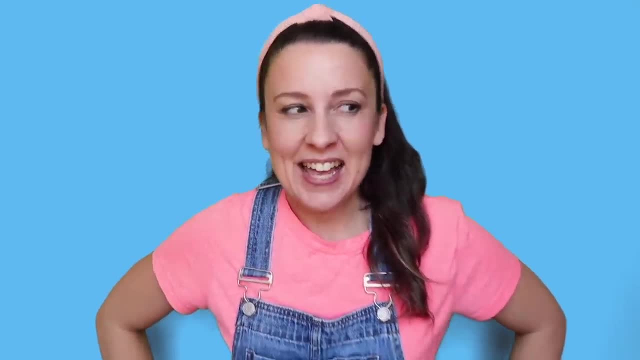 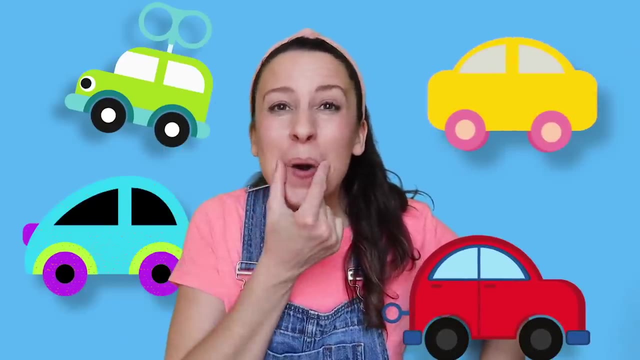 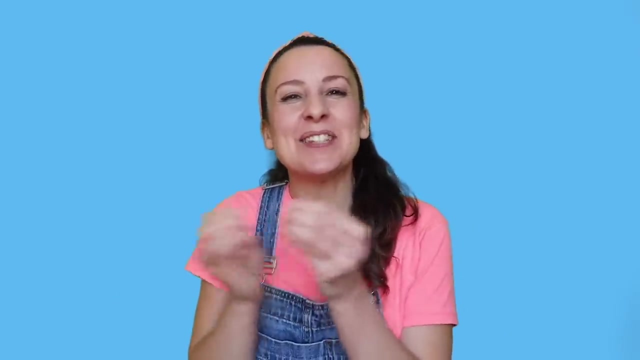 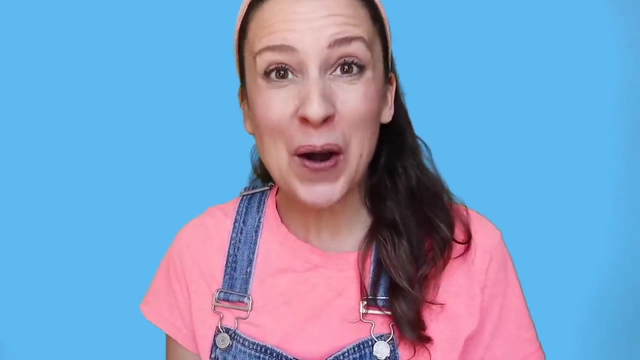 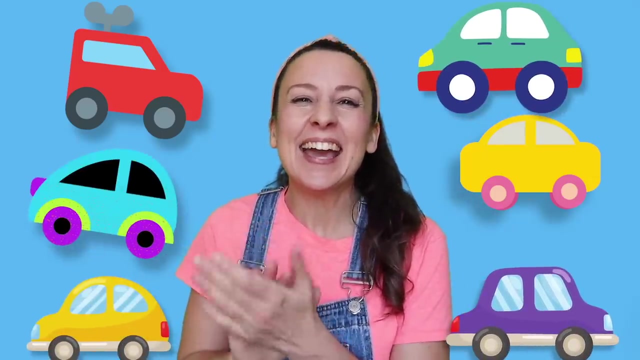 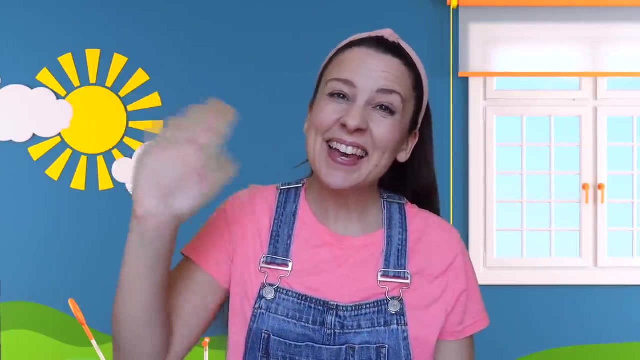 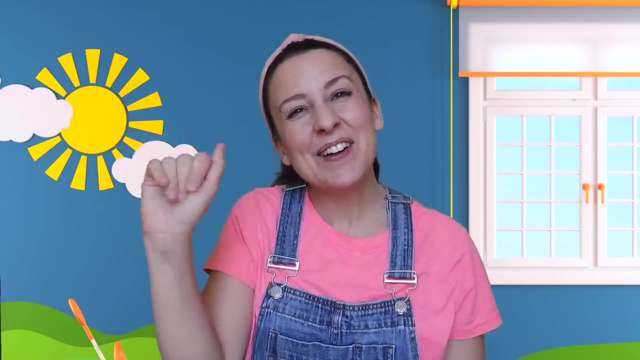 come out, Ready set go, Wow, Wow Cars. Let's do more, Let's do more. Ready set go. More cars, More cars. Yay, Can you wave? This is waving Wave. hello, Hi, Hello, We're. 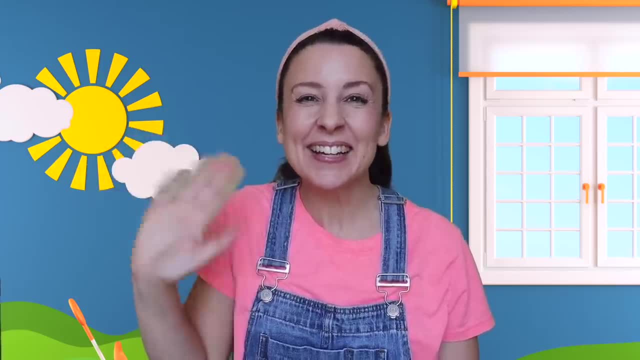 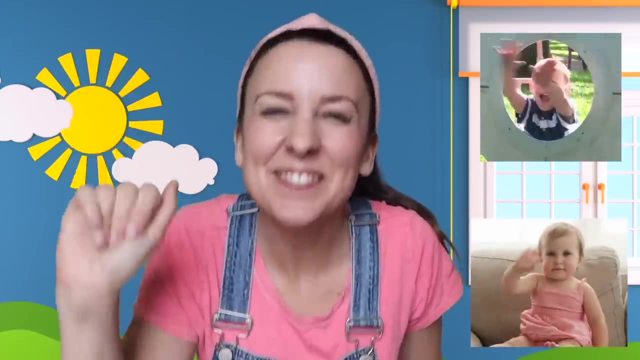 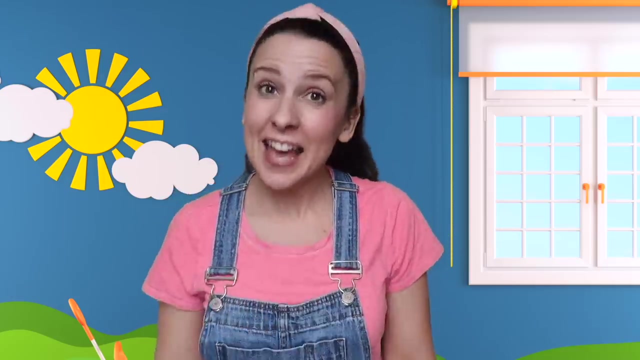 waving, Waving, We're waving, We're waving, We're waving, waving, waving, We're waving, We're waving, We're waving. Now we stop. Did you stop? Good job, Let's try clapping We're. 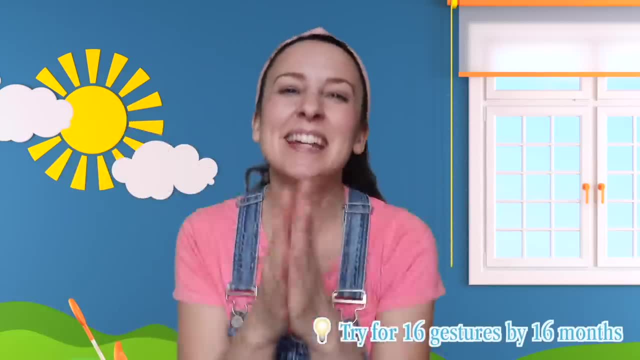 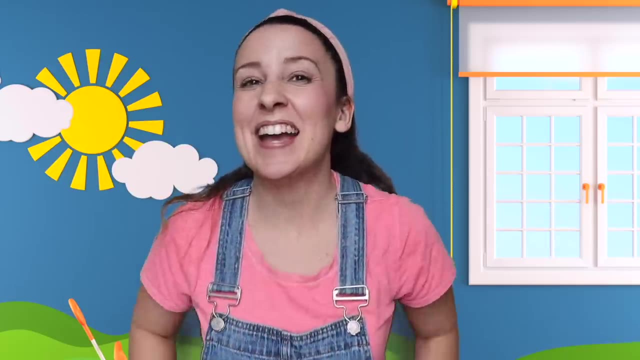 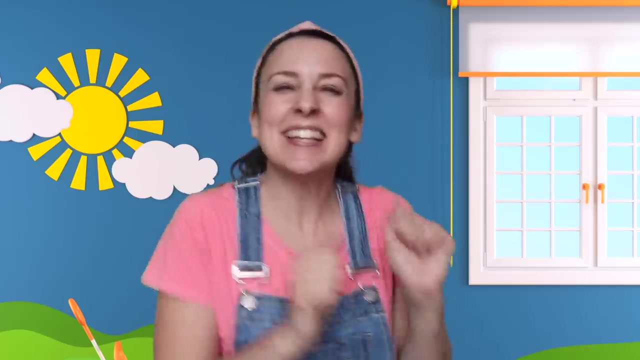 clapping, We're clapping, We're clapping, clapping, clapping, We're clapping, We're clapping, We're clapping. Now we stop. Let's try twisting, We're twisting, We're twisting, We're twisting, twisting, twisting. 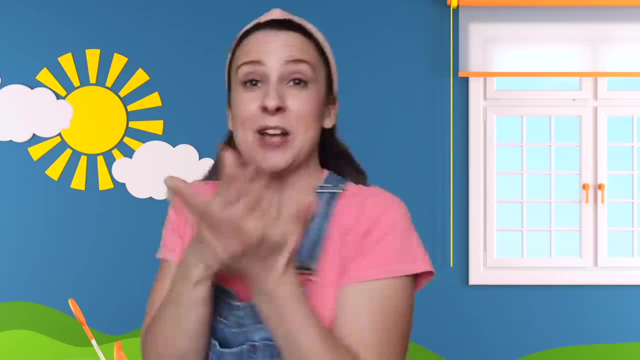 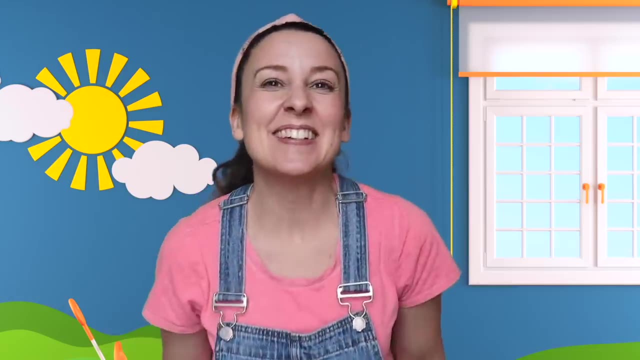 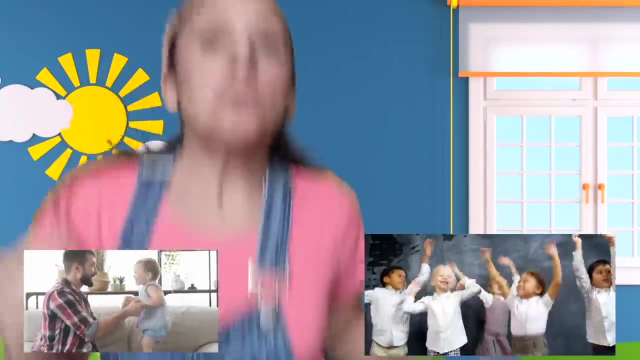 We're twisting, We're twisting, We're twisting, Now we stop. Good job, Hmm, Should we try jumping? Let's do it. We're jumping, We're jumping, We're jumping, jumping, jumping, We're jumping, We're jumping, We're jumping, Now we stop. That was so much fun, Great job. 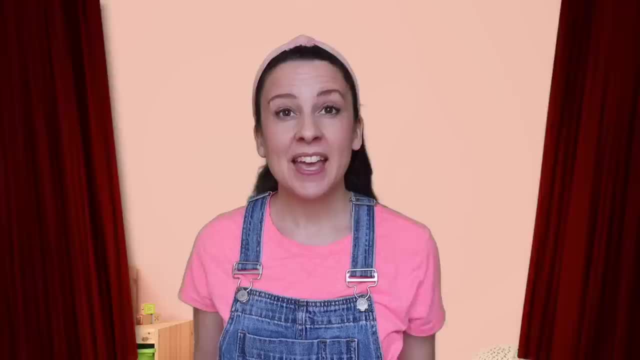 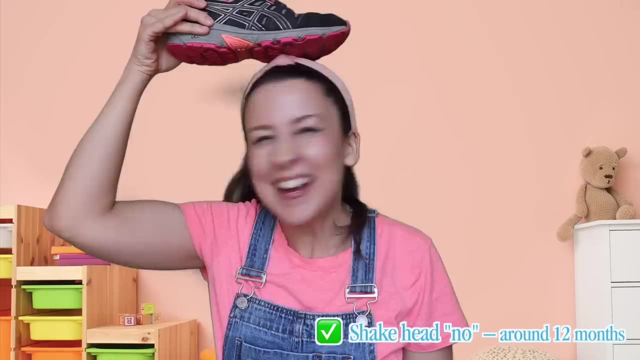 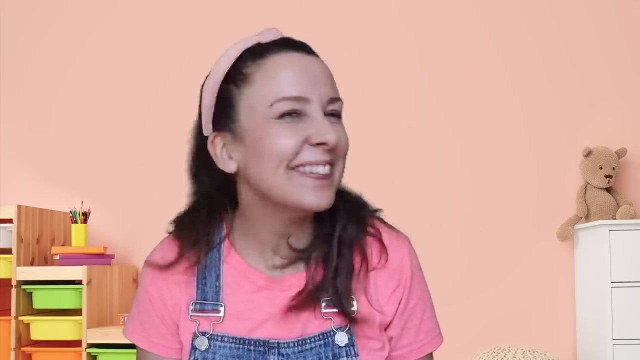 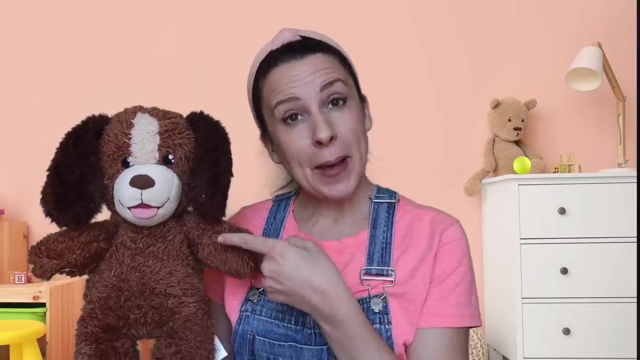 Does a shoe go on my head? No, No, no, no. Can you shake your head? no, No, No, A shoe doesn't. Oh, oh, Oh, oh, Oh. Does puppy want the ball? Yes, Does puppy want the ball? 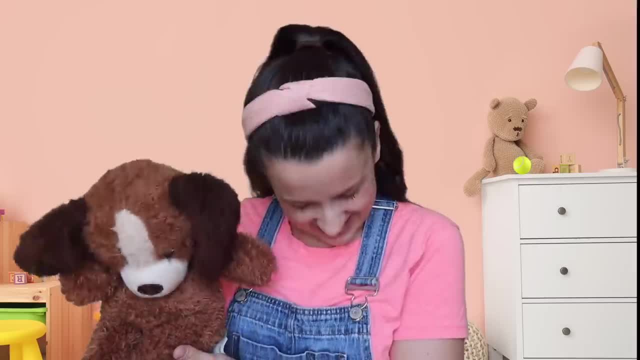 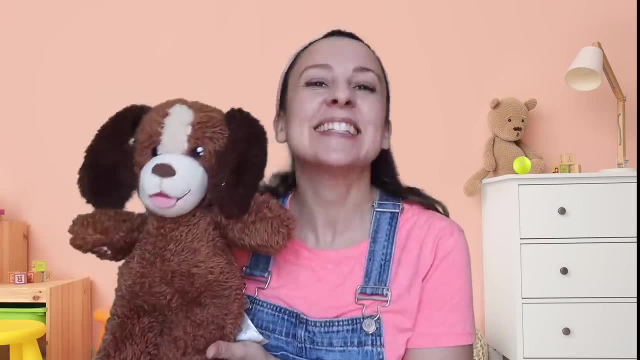 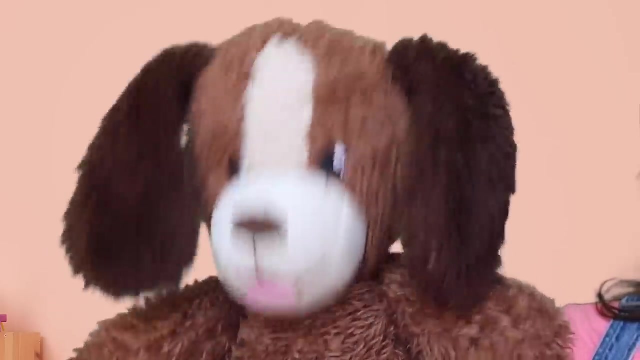 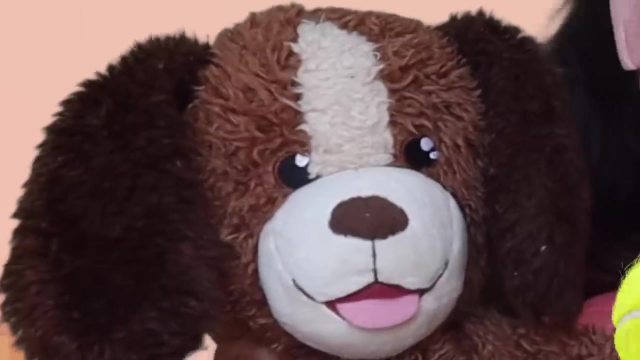 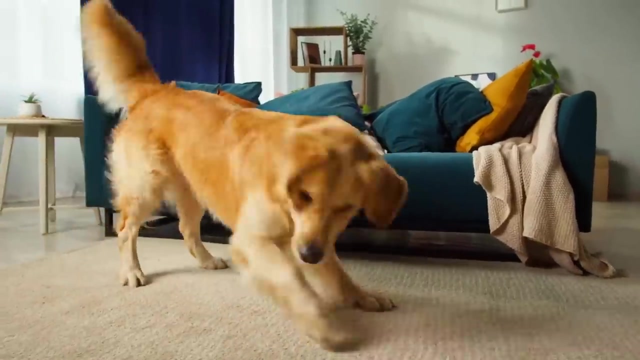 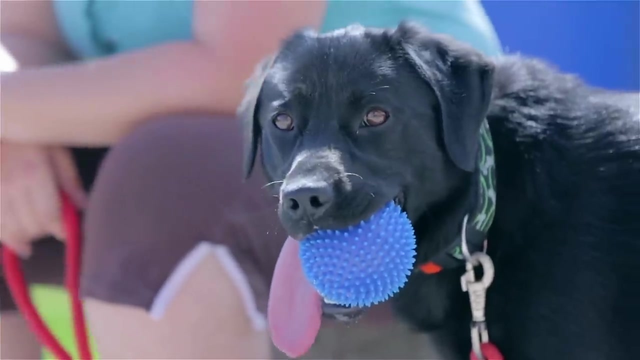 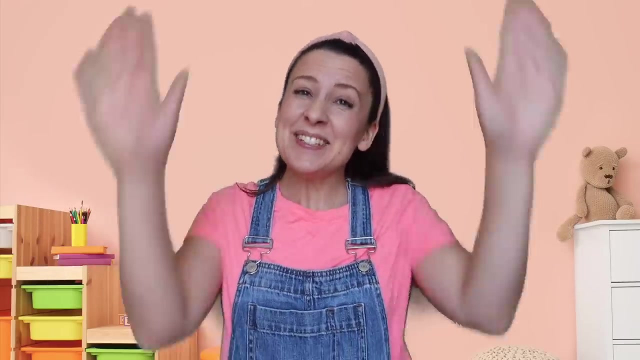 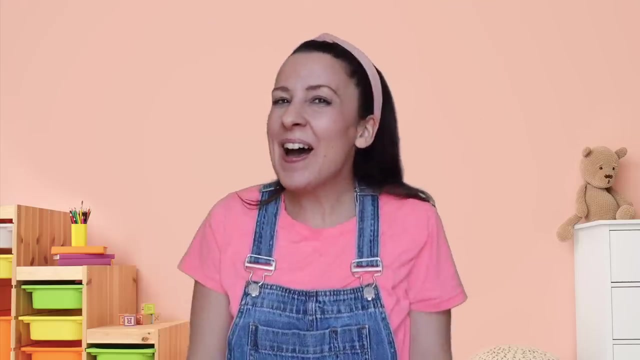 Yes, Yes, Can you nod? yes, Puppy wants the ball. Yes, Yes, yes, yes, Yes, I want the ball. Yes, Yes, How big is baby? So big? Can you put your arms up? Arms up, Arms up. How big is baby. 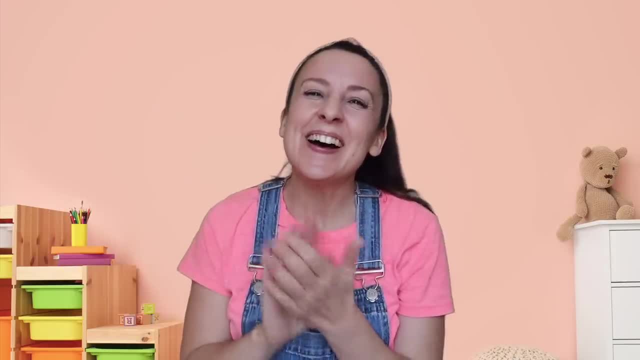 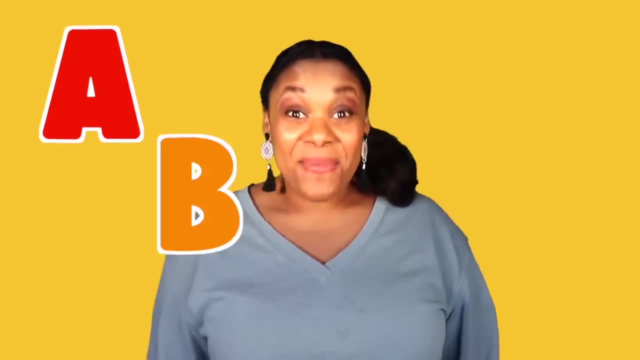 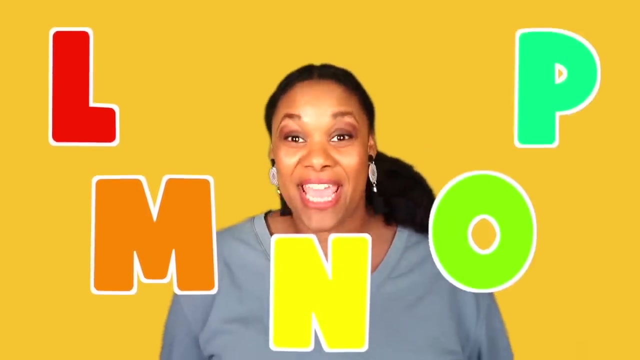 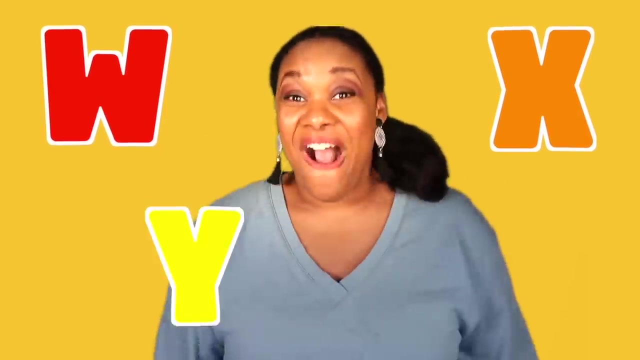 So big Good job. A, B, C, D, E, F, G, H, I, J, K, L, M, N, O, P, Q, R, S, T, U, V, W, X, Y and Z. 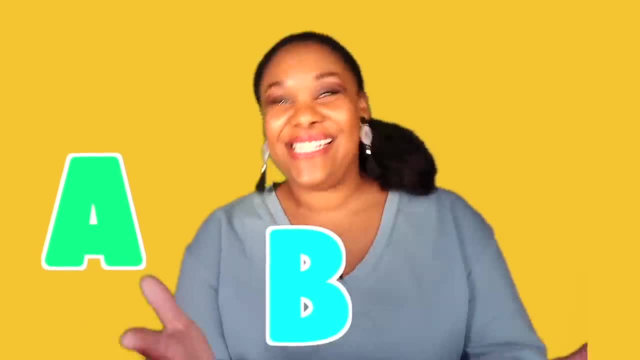 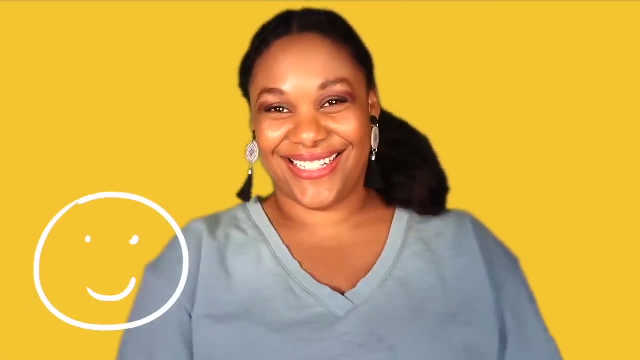 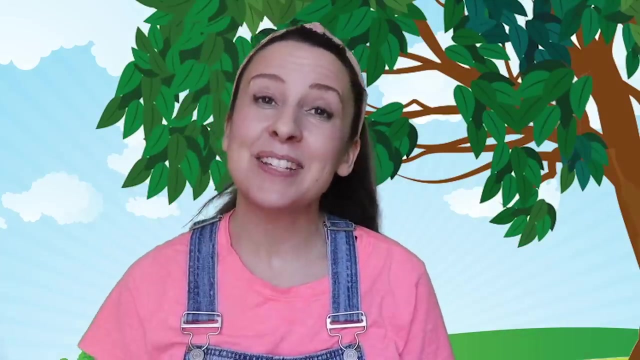 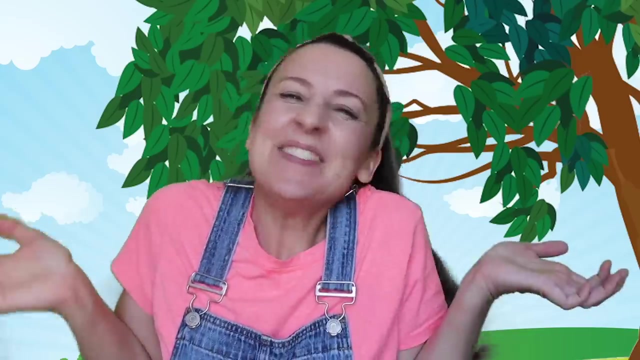 Now I know my ABCs. Next time won't you sing with me Hm. Where is the bird? Hm. Can you say: I don't know, I don't know. Can you do that? I don't know, I don't know, I don't know. Let's call him to come out. Say bird. 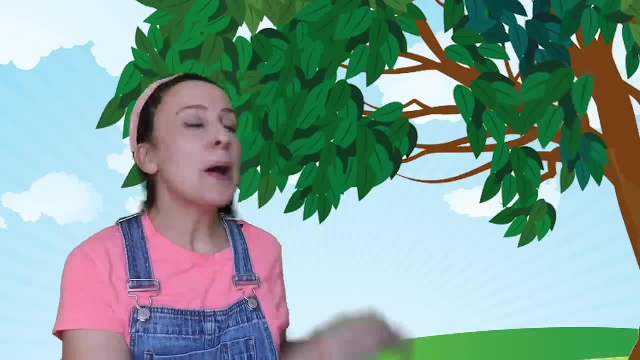 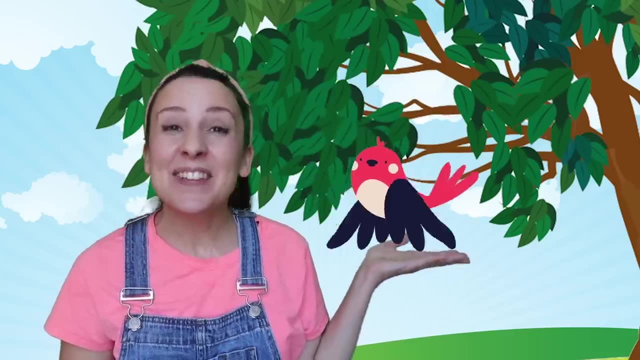 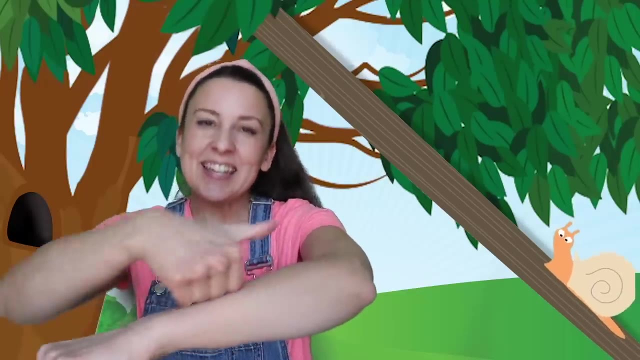 with me. Biiird, Where are you Bird? Oh, the bird was out. A bird was out, Cardнибудь. The bird was in the tree. Now he came out. He was in the tree. Slowly, slowly, very slowly creeps the garden snail. 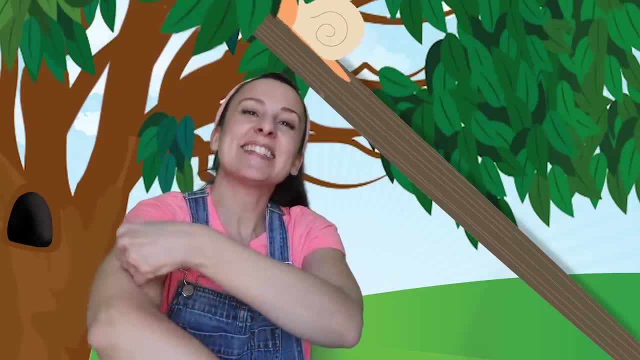 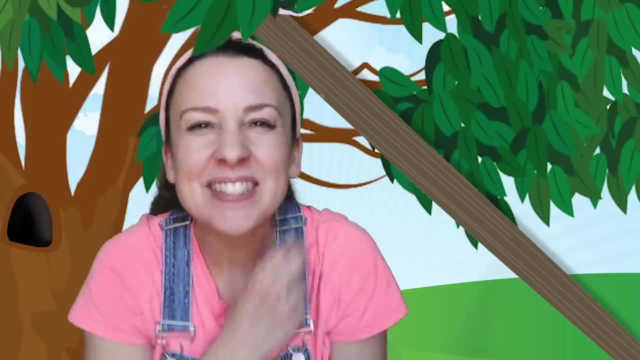 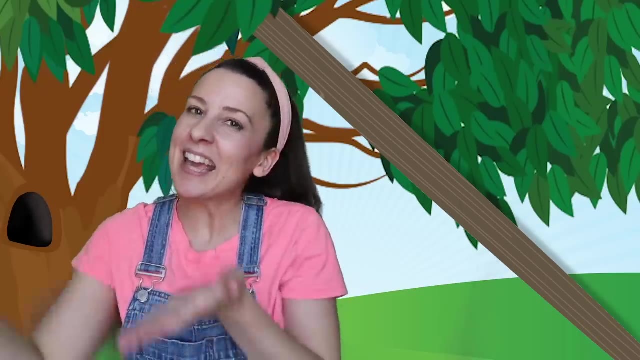 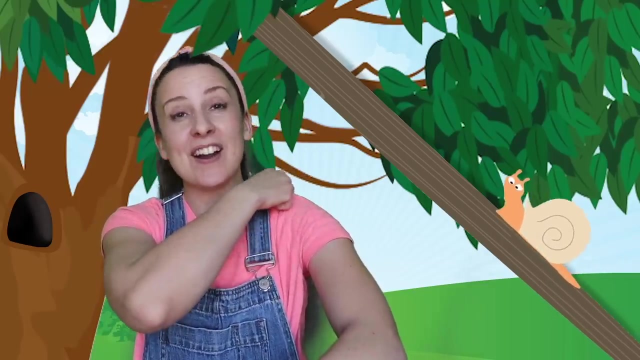 Slowly, slowly, very slowly up the wooden rail. Quickly, quickly, very quickly runs a little mouse Quickly, quickly, very quickly into his little house. And that was fun. Let's do it again. Slowly, slowly, very slowly creeps the garden snail. 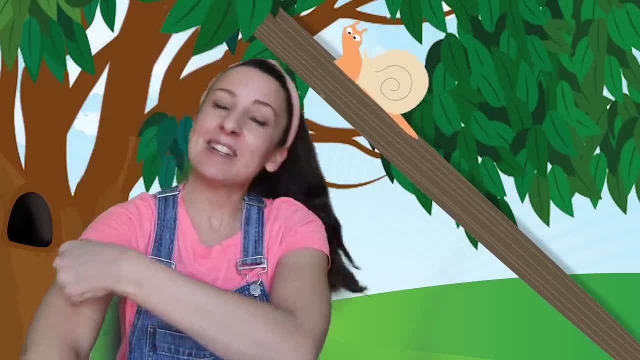 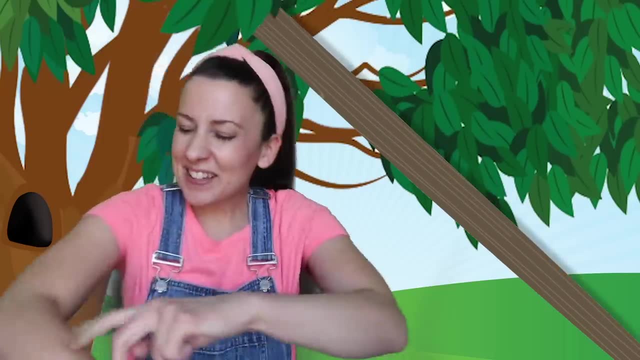 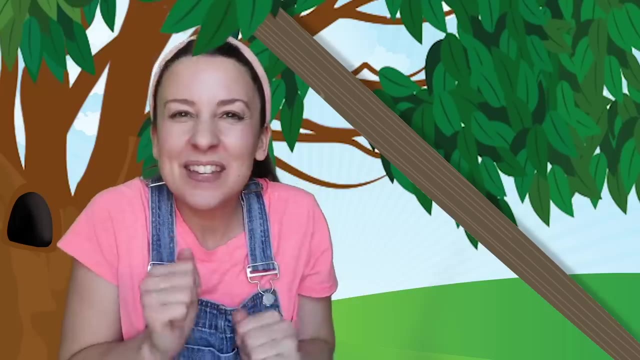 Slowly, slowly, very slowly up the wooden rail. Quickly, quickly, very quickly runs a little mouse Quickly, quickly, very quickly into his little house. And that was fun. We were quick like a mouse, Can you be quick? 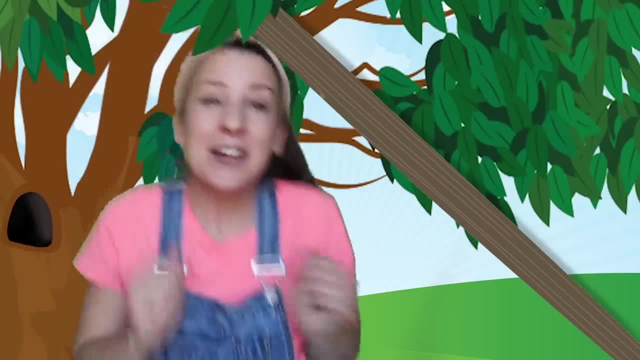 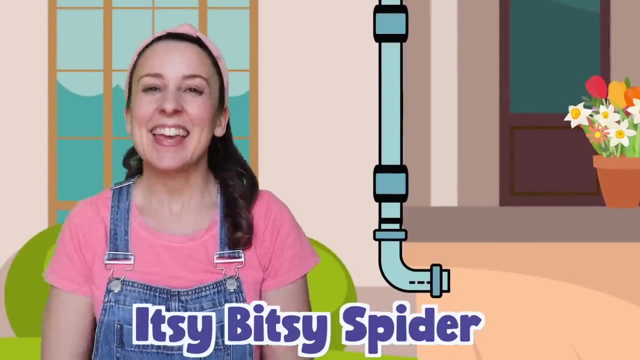 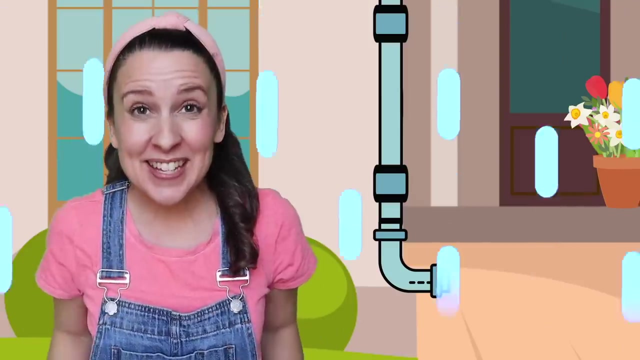 Quick, quick and slow like a snail. Quick, quick like the mouse and slow like the snail. Good job. The itsy bitsy spider went up the water spout. Down came the rain and washed the spider out. 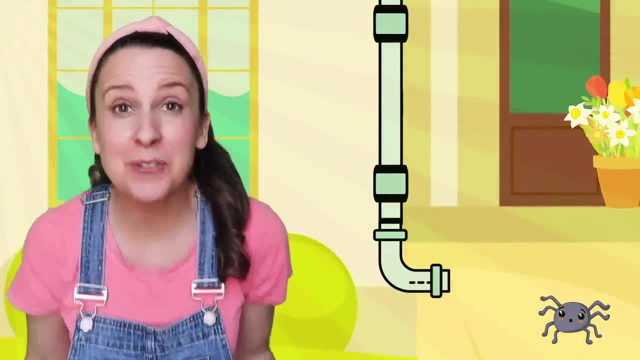 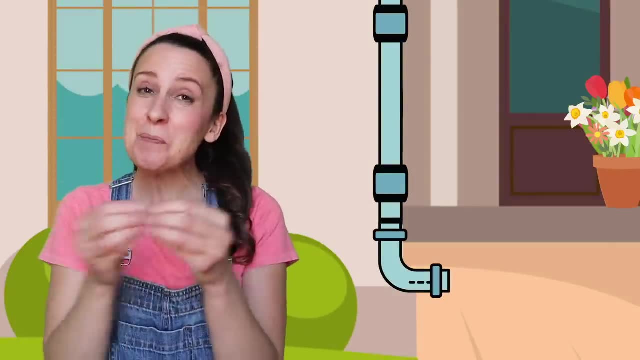 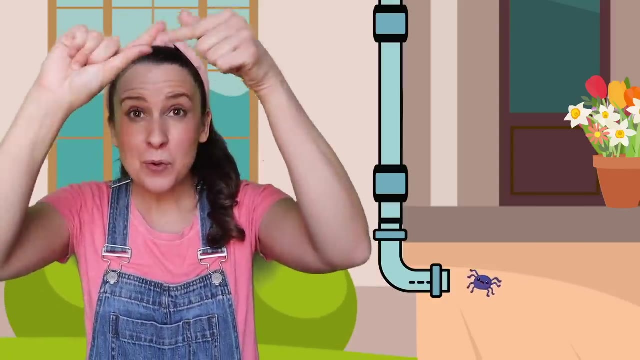 Out came the sun and dried up all the rain And the itsy bitsy spider went up the spout again. Let's do more. Let's do that again. The itsy bitsy spider went up the water spout. Down came the rain and washed the spider out. 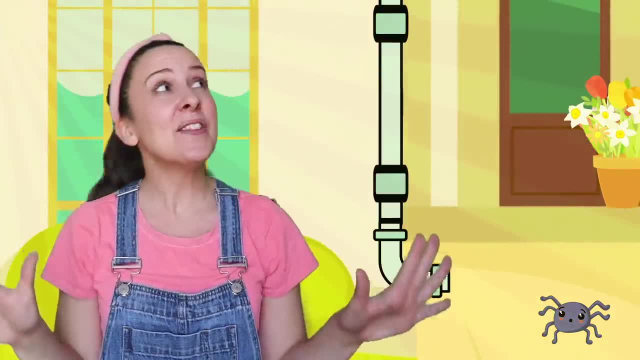 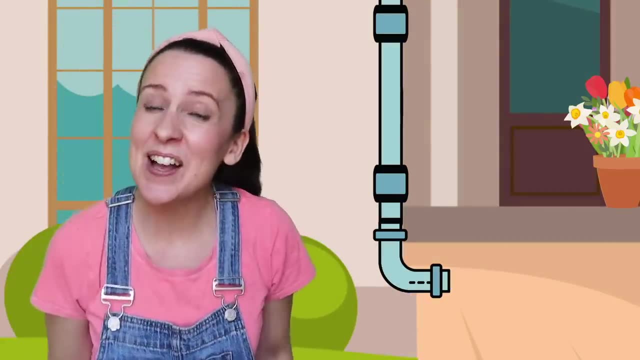 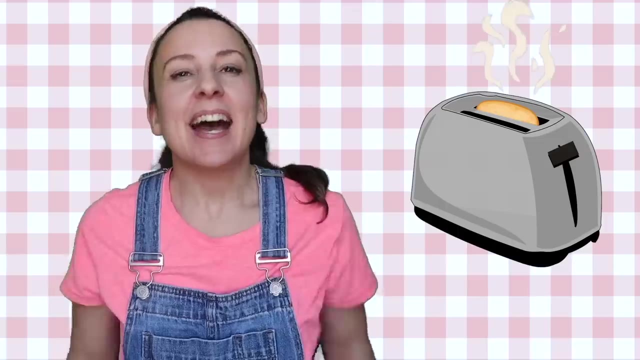 Out came the sun and dried up all the rain And the itsy bitsy spider went up the spout again. Great job with your spider. Can you pretend to be toast with me? I'm toast in the toaster. I'm getting very hot. 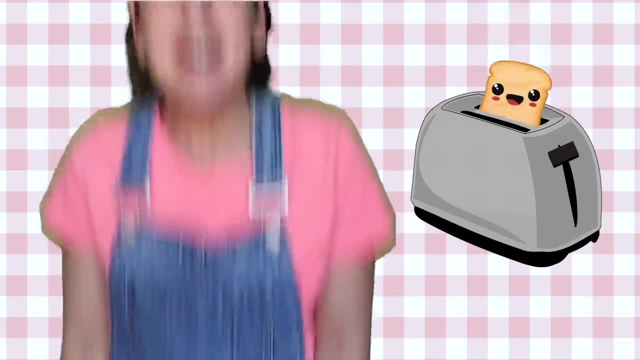 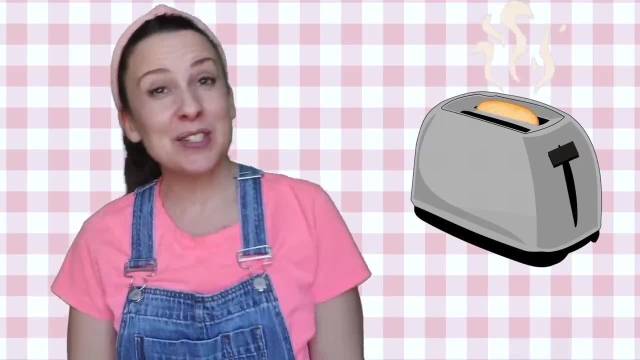 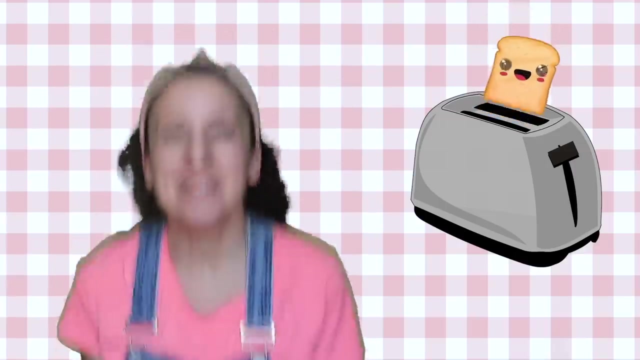 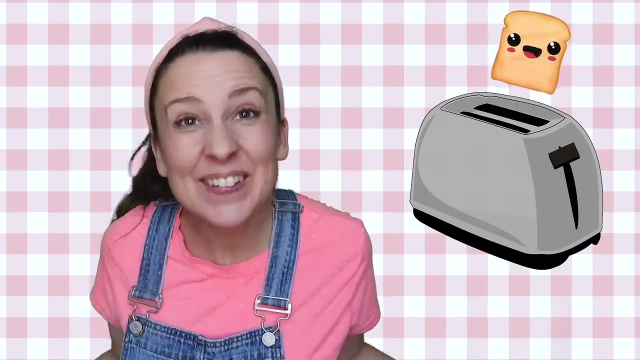 Tick-tock, tick-tock up, I pop. Let's do that again. That was fun. I'm toast in the toaster. I'm getting very hot. Tick-tock, tick-tock up, I pop. Hahaha, Did you pop up like toast? 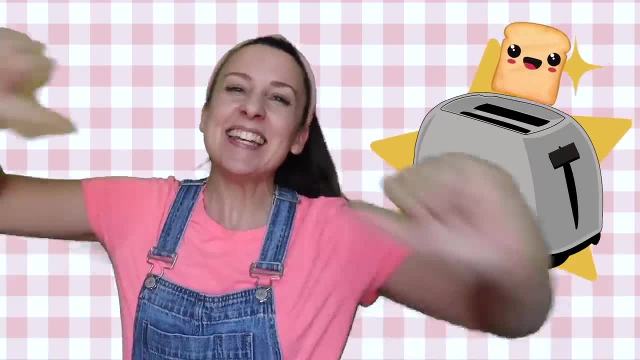 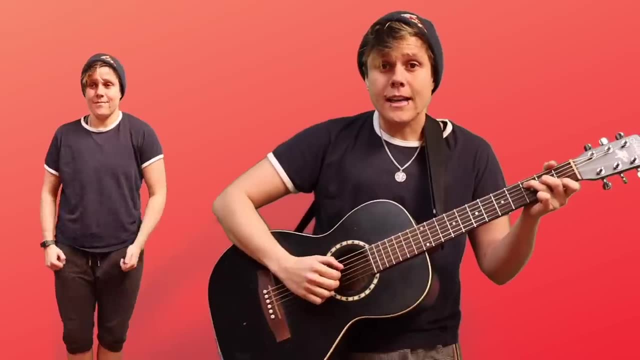 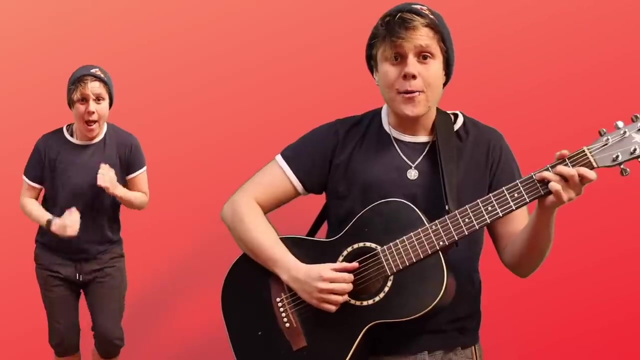 Good job, You did it. Say I did it, I did it. Walking, walking, walking, walking. Hop, hop, hop, hop, hop, hop, Running, running, running, running, running, running. Now we stop, Now we stop. 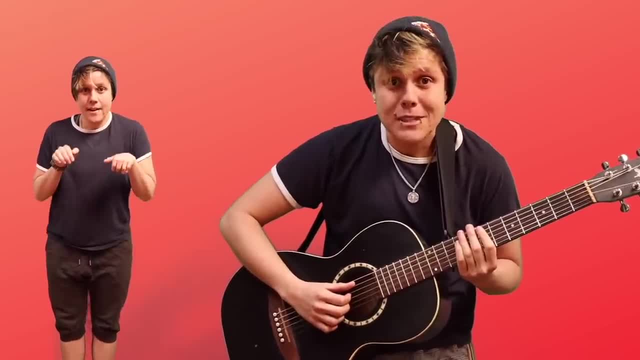 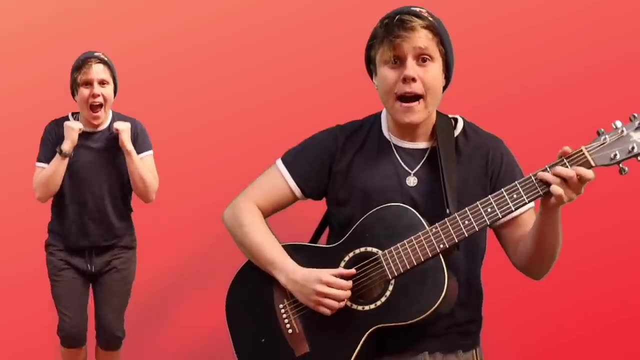 Yeah, that's it. Okay, let's try to tiptoe. Are you ready? Tiptoe, tiptoe, tiptoe, tiptoe, Hop, hop, hop, Hop, hop, hop. Running, running, running, running, running, running. 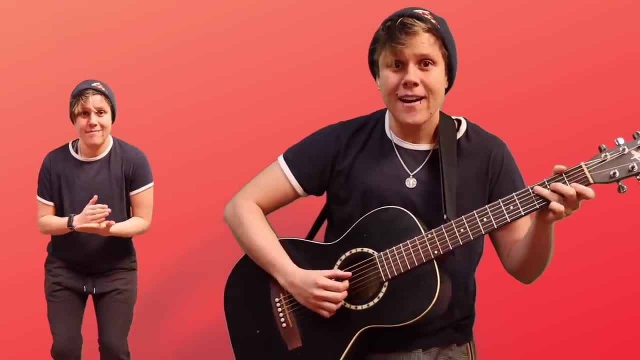 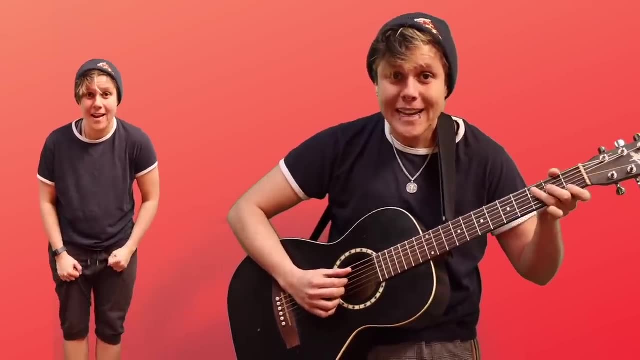 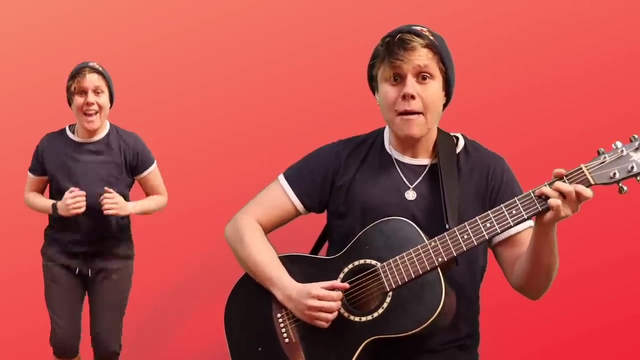 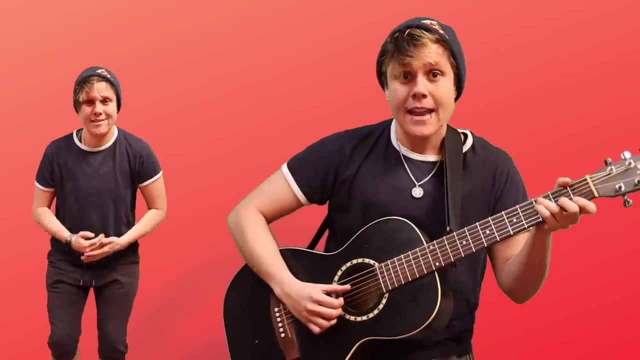 Now we stop, Now we stop. Wow, you all are so good at this. Okay, Okay, Let's try marching. Are you ready? Marching, marching, marching, marching, Hop, hop, hop, Hop, hop, hop, Running, running, running, Running, running, running. Now we stop, Now we stop. 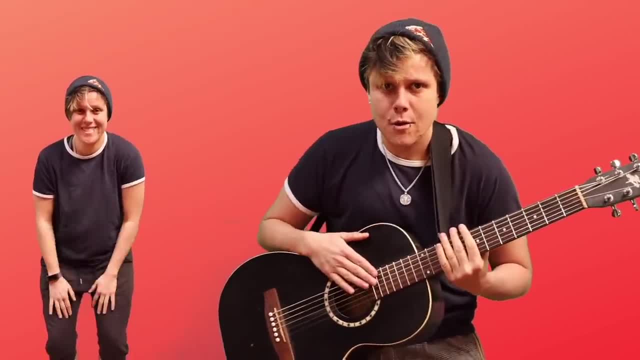 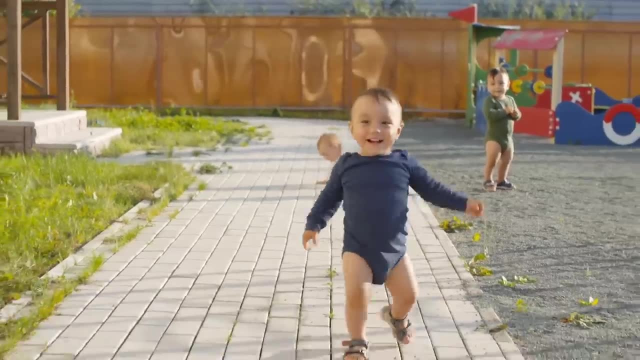 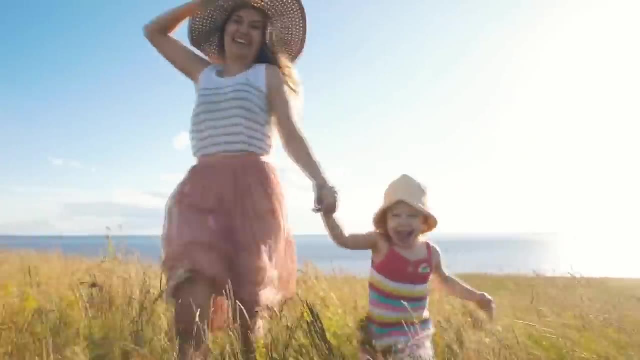 Wow, Y'all did so good. Do you think we could go a little bit faster? Okay, Let's try it. Marching, marching, marching, marching. Hop, hop, hop, Hop, hop, hop, Running, running, running, Running, running, running. Now we stop, Now we stop. 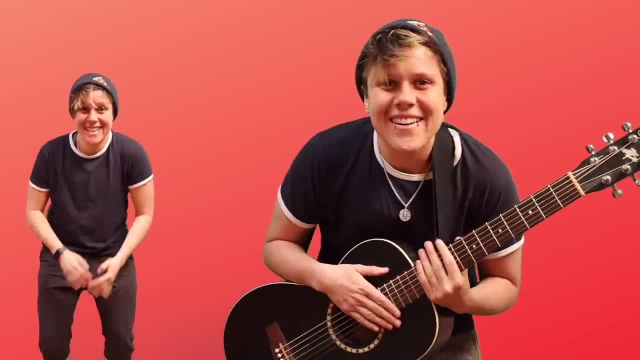 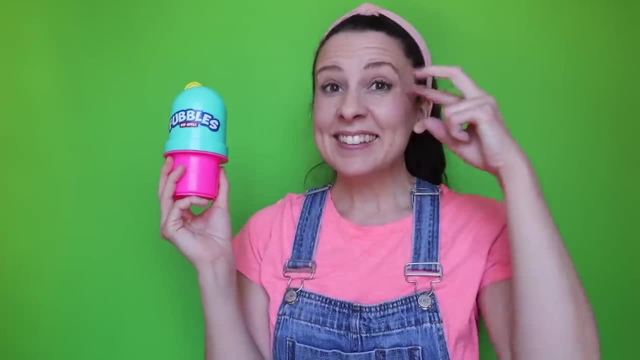 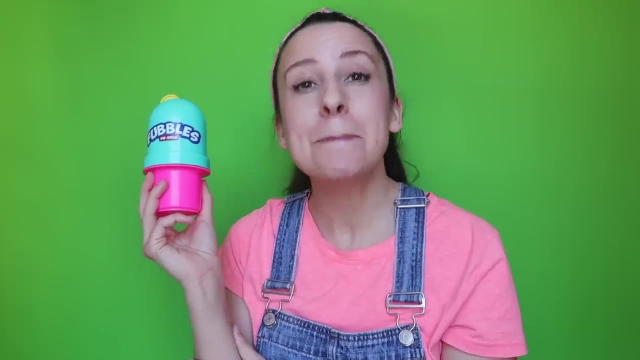 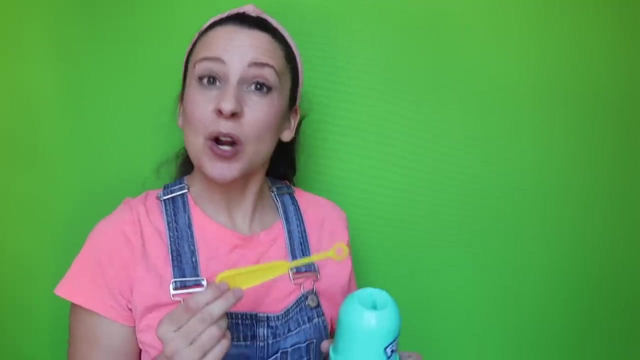 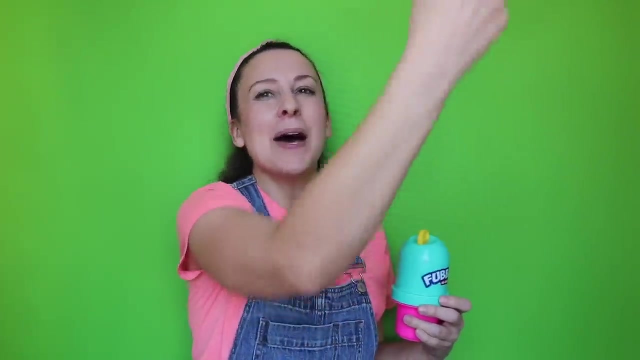 Wow, Y'all did so good, Awesome job at following directions. Okay, Bye-bye. Look Bubbles. Can you say bubble, Bubble, Bubble, Let's blow some bubbles. Ready, set, go. Wow, Pop, pop, I'm popping the bubbles. 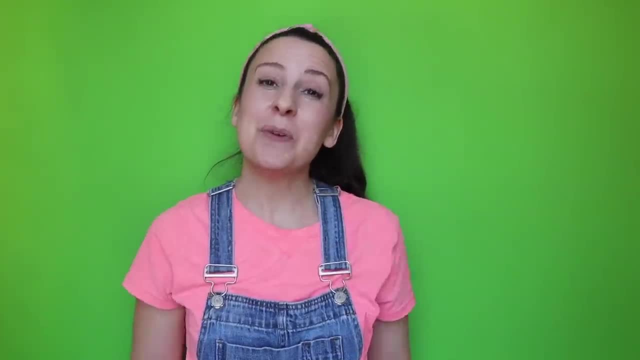 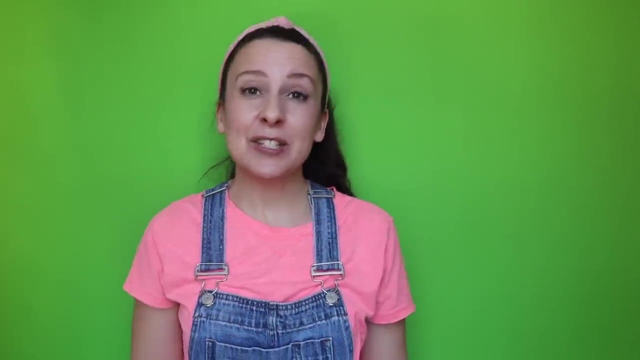 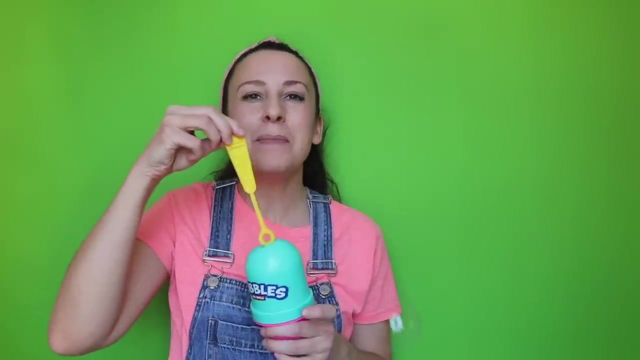 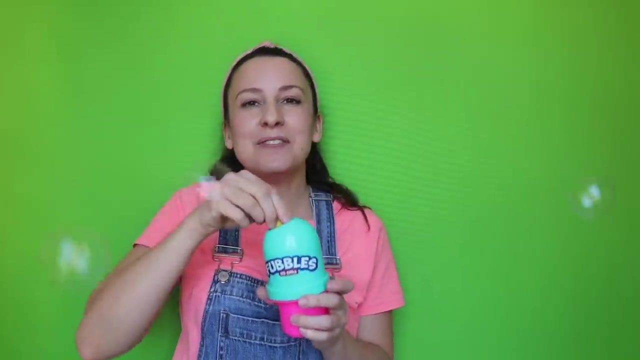 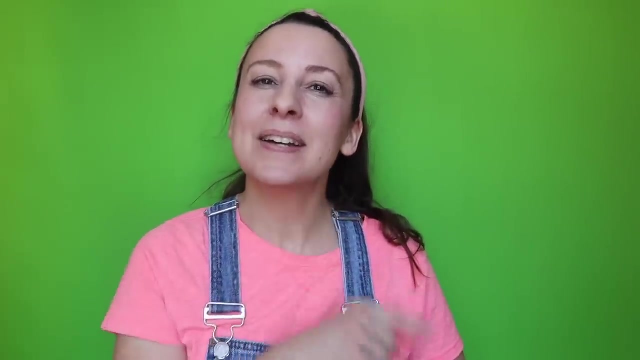 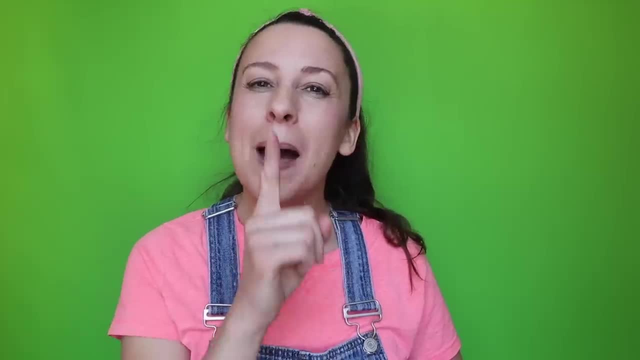 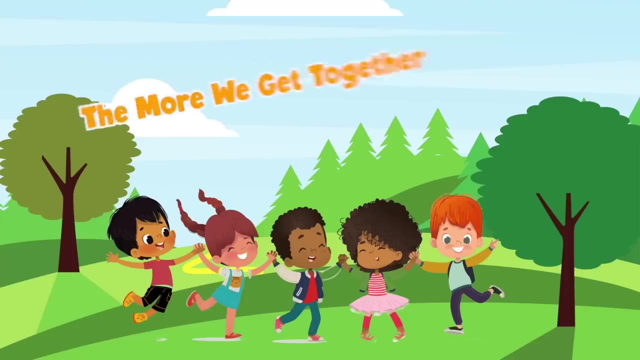 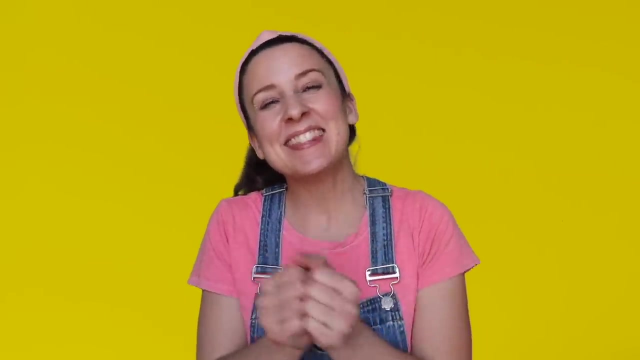 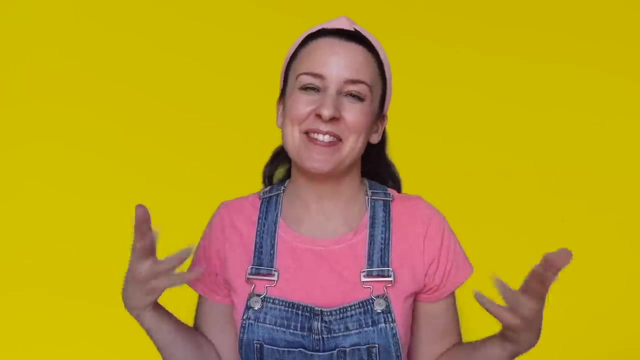 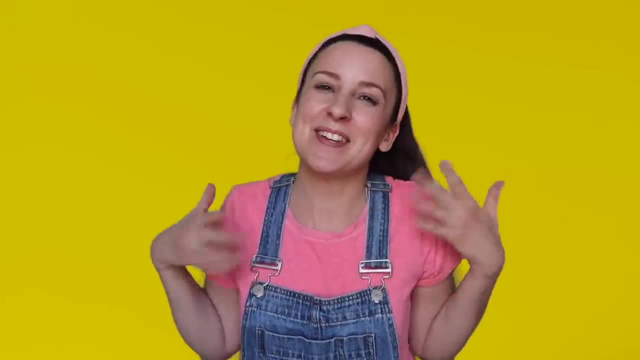 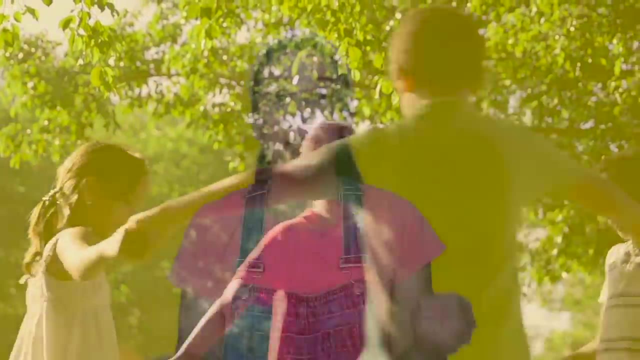 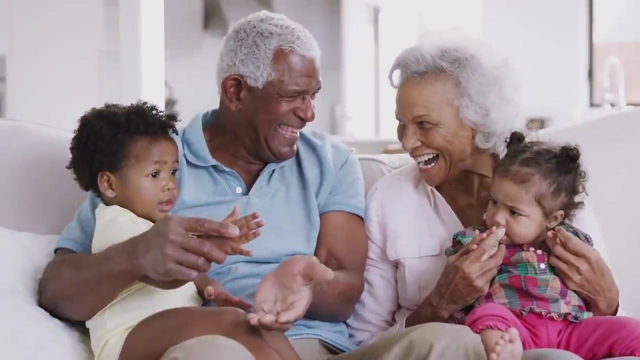 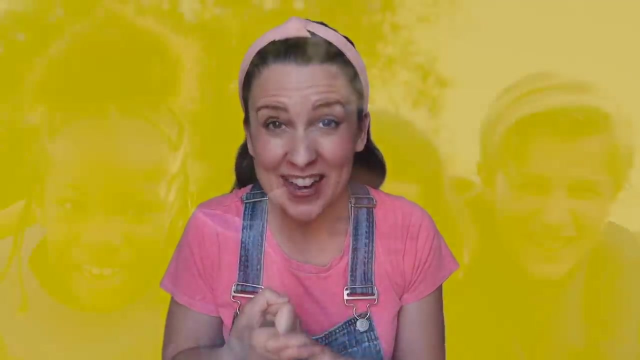 The more we get together, the happier we'll be. The more we get together, together, together, The more we get together, the happier we'll be, Cause your friends are my friends and my friends are your friends. The more we get together, the happier we'll be. 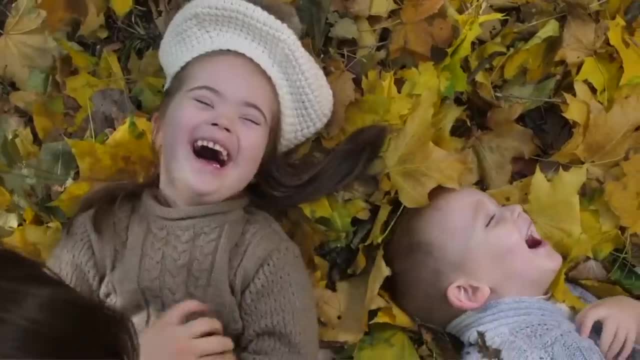 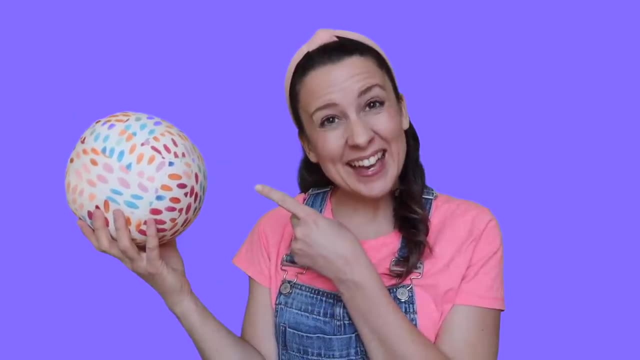 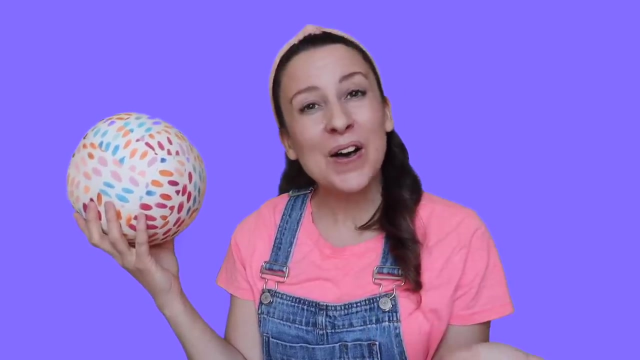 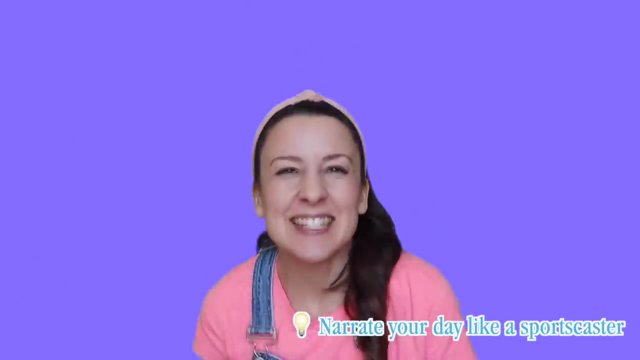 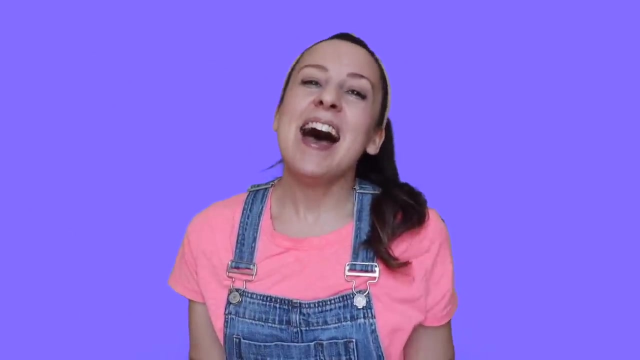 What's that? What is that? It's a ball Ball. Can you say: ball Ball, Throw the ball, catch the ball, Throw the ball, catch the ball. Yay, Throw the ball, catch the ball, Throw the ball, Uh-oh. 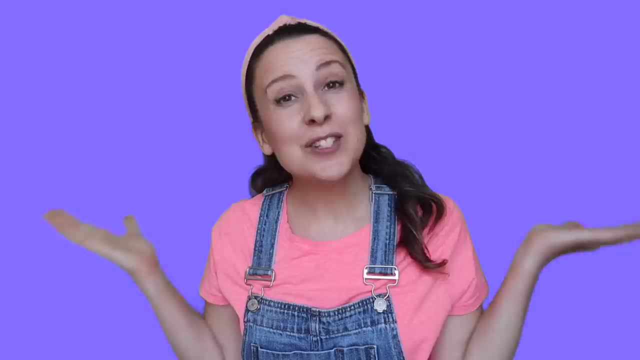 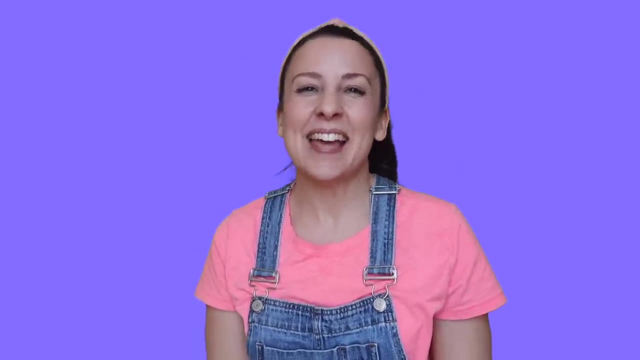 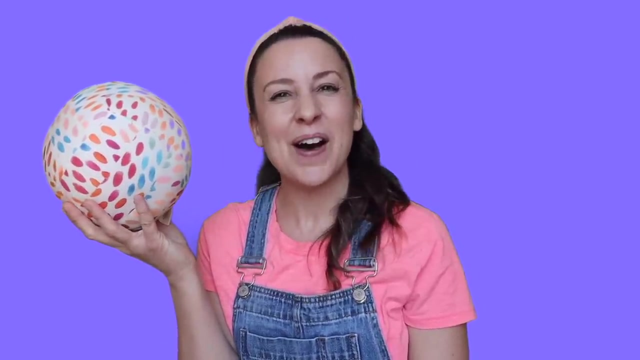 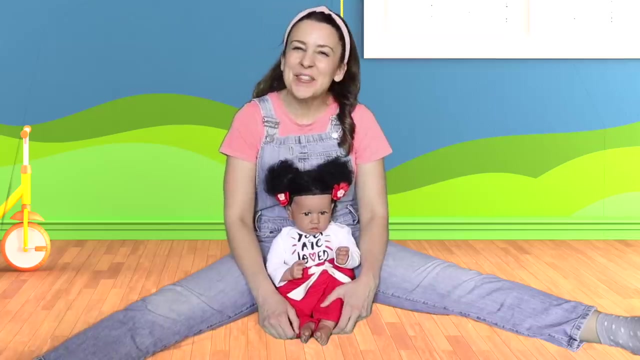 Can you say that, Uh-oh, I dropped the ball? Oh, no, Uh-oh, I'll pick it up. Here it is, I found it. I found the ball. Uh-oh, Uh-oh, Roll the ball, Catch the ball. 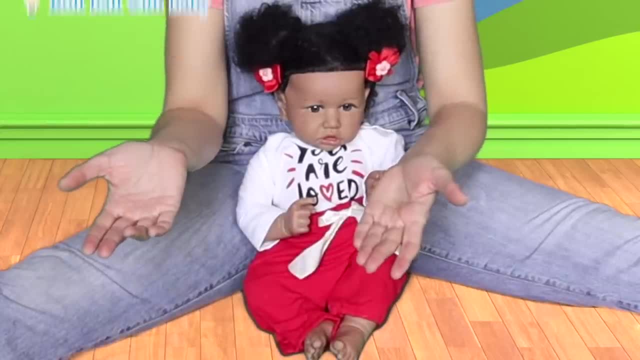 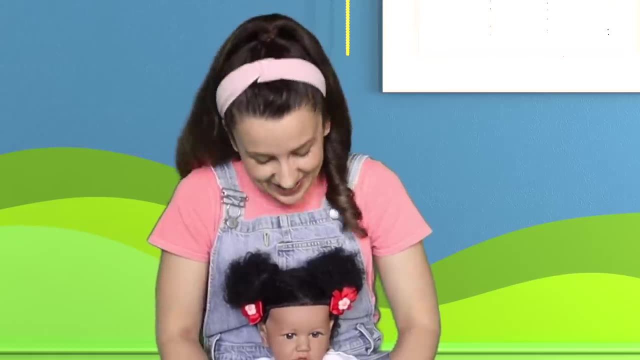 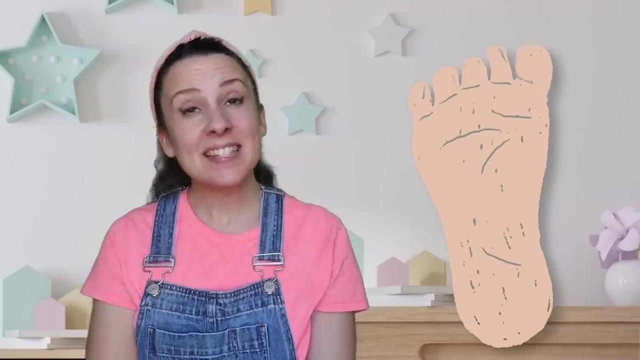 Now let's roll it Roll. Roll the ball, Roll the ball, Catch the ball. Let's roll it Roll. Yay, Clap clap, clap clap. This little piggy went to market. This little piggy stayed home. 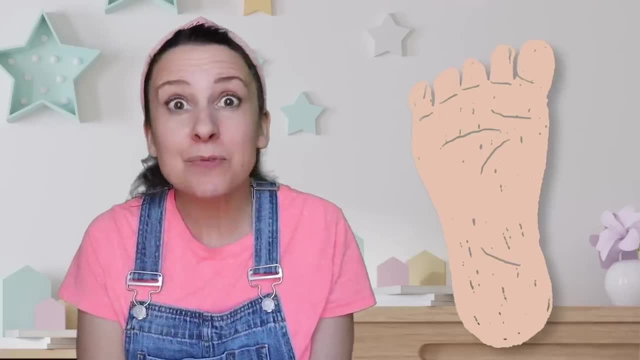 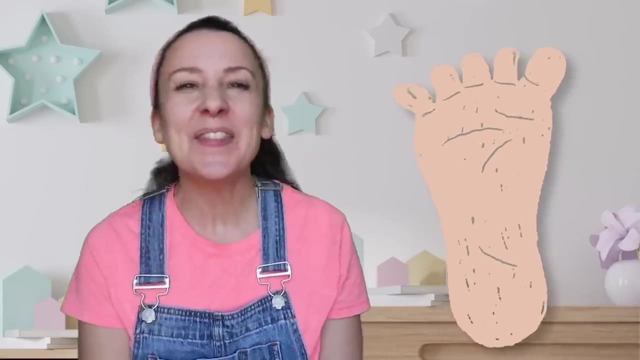 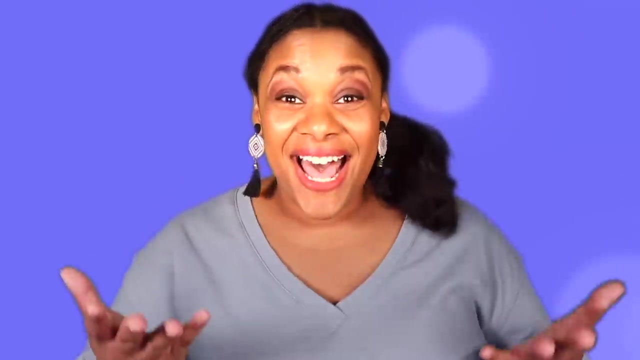 This little piggy had roast beef And this little piggy had none. And this little piggy went wee, wee, wee, all the way home. Let's sing: London Bridges, London Bridges, falling down, falling down, falling down, London Bridges, falling down. 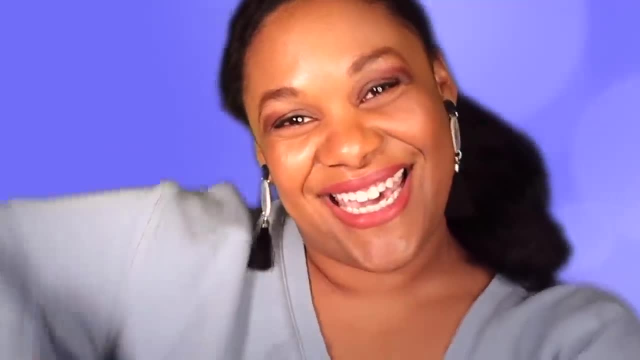 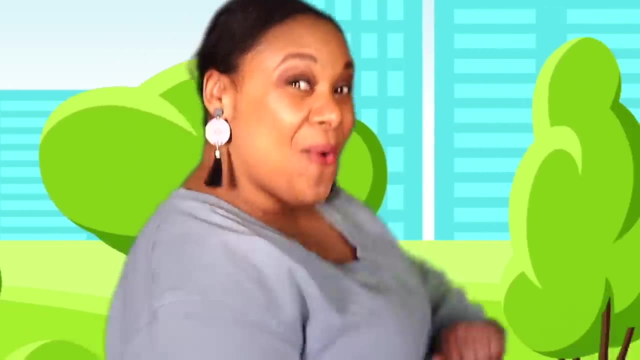 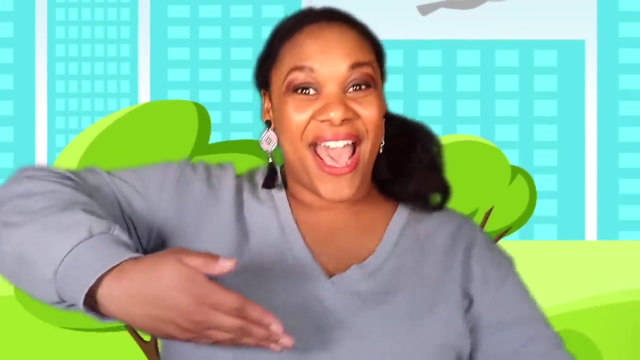 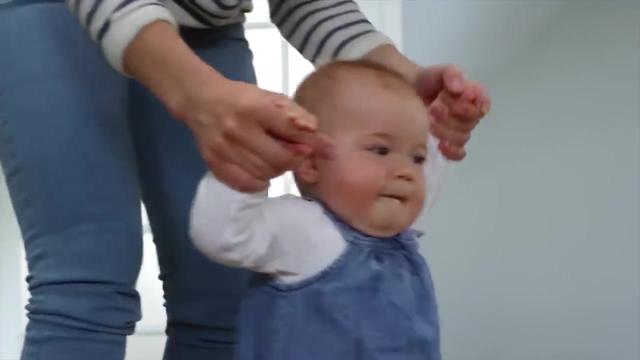 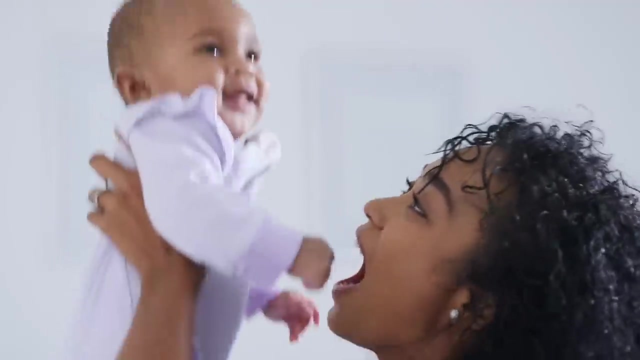 My sweet baby. So come and take a walk with me, walk with me, walk with me. come, take a walk with me, my sweet baby. London Bridge is falling down, falling down, falling down. London Bridge is falling down, my sweet baby. 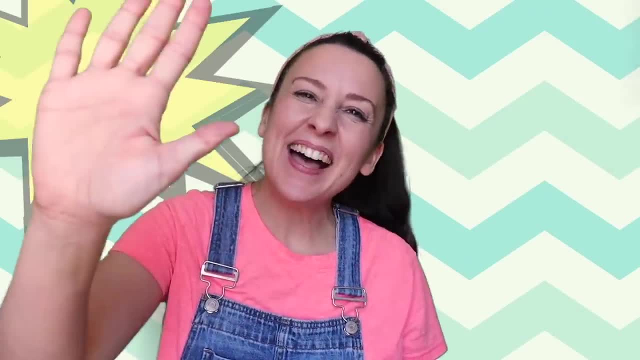 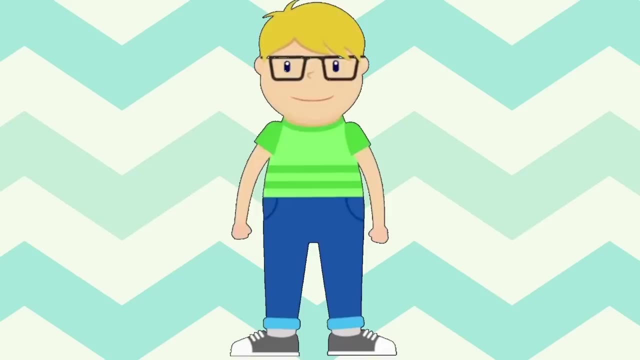 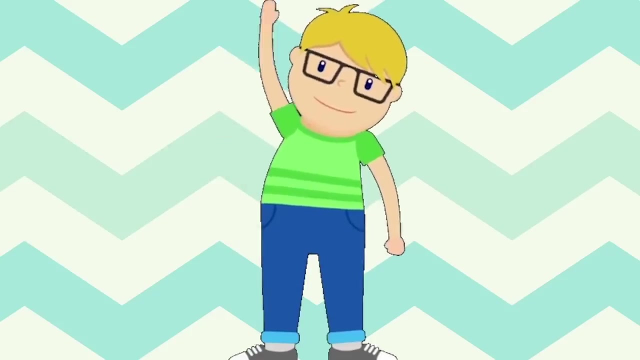 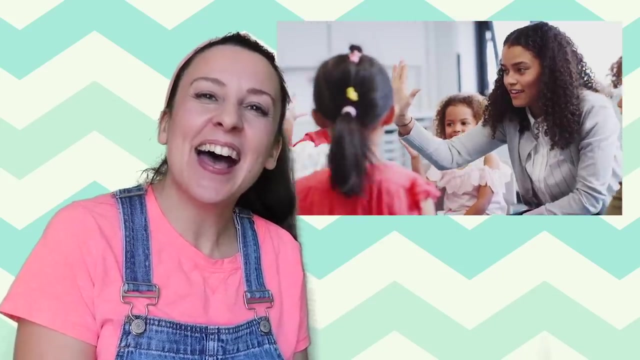 Can you give a high five, High five. Yay, Let's give a high five, High five. Can you give a high five to the little boy? High five, High five. So fun, High five. Yay, Giving a high five, High five, High five. 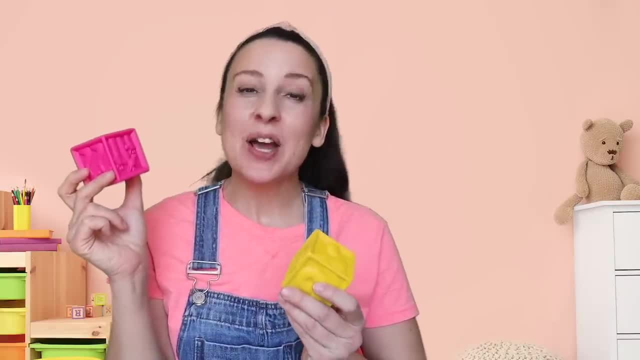 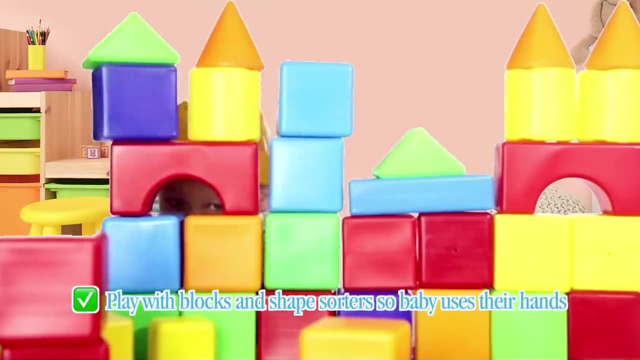 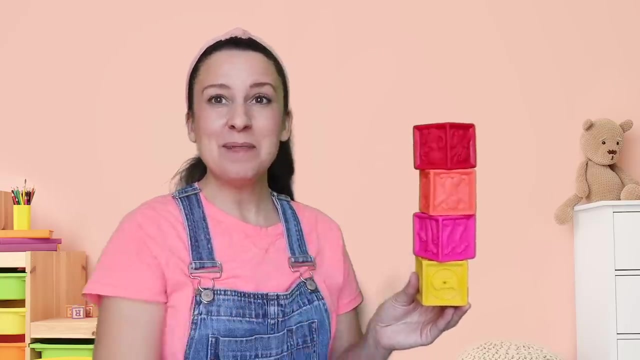 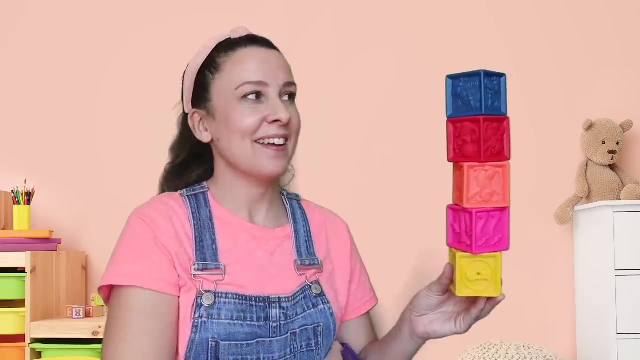 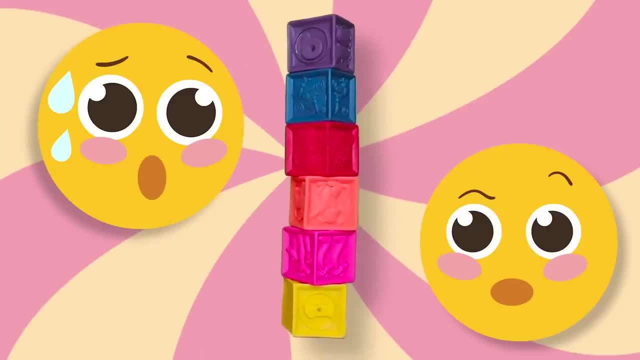 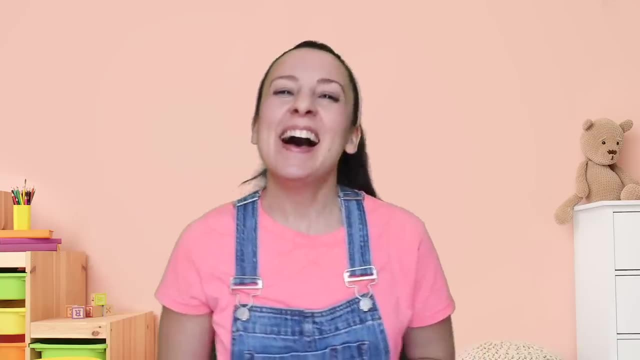 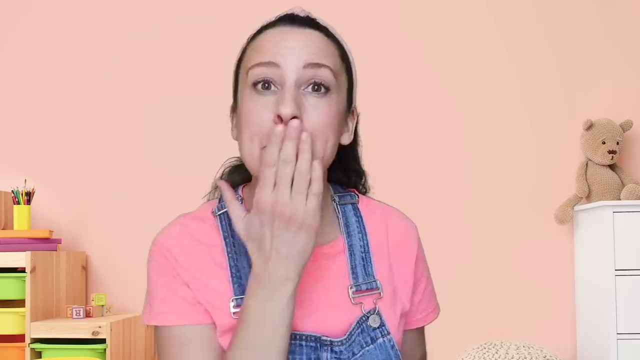 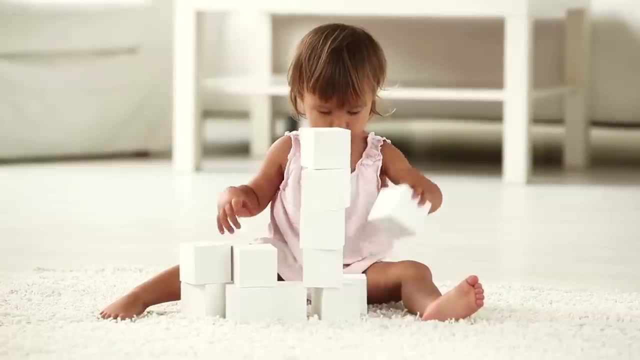 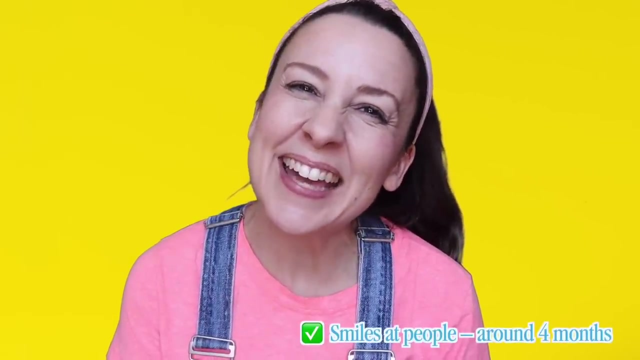 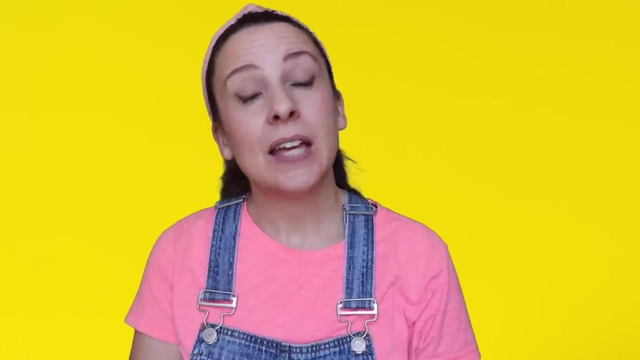 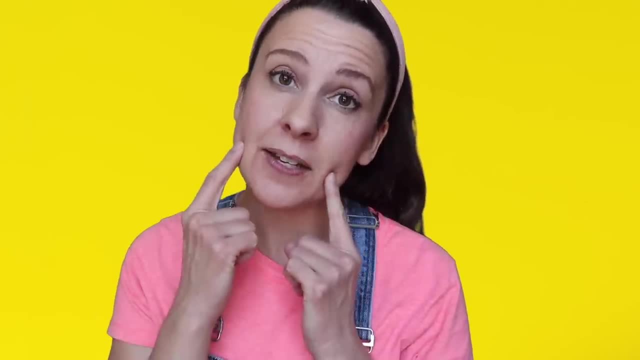 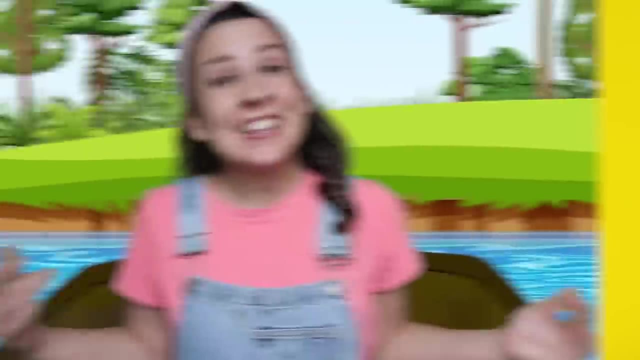 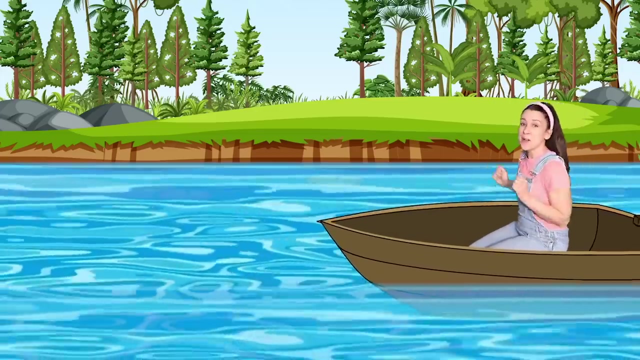 Can you frown? This is frowning, But now I'm happy again, I'm happy again. Yay, Let's sing. row, row, row your boat, Get out your paddles, Row, row, row your boat, gently. 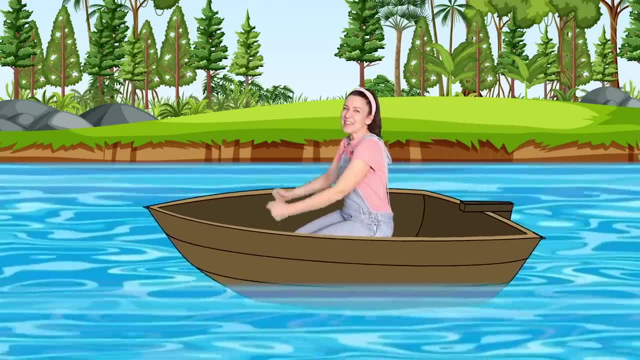 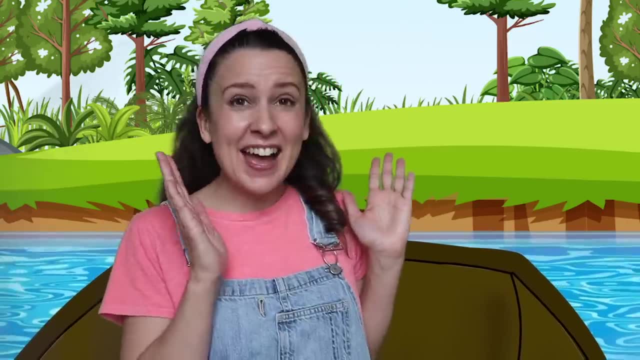 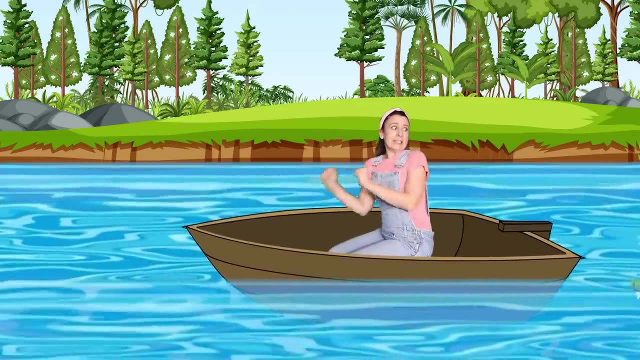 down the stream Merrily, merrily, merrily, merrily. life is but a dream This time. let's pretend we see a crocodile Row row. row your boat gently down the stream, If you. 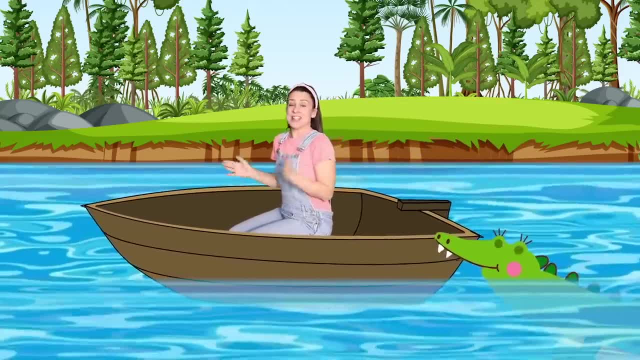 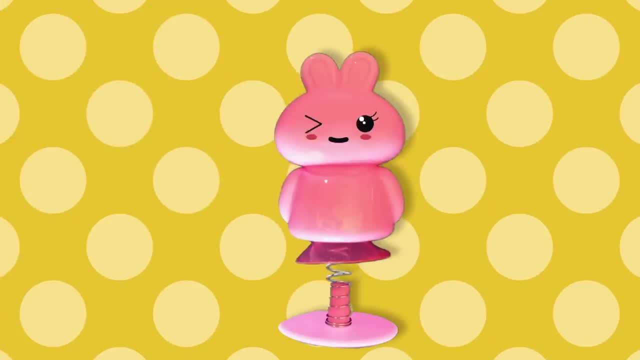 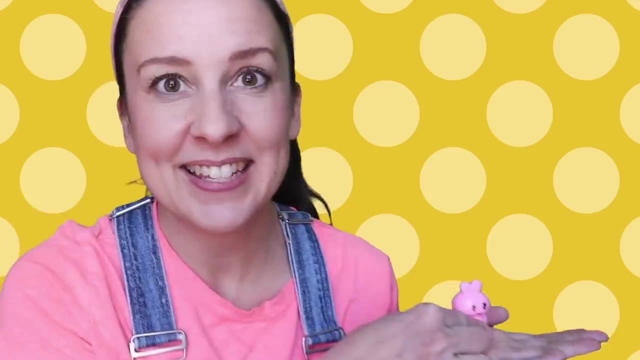 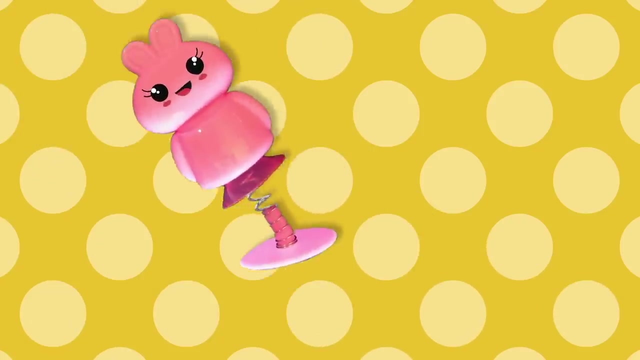 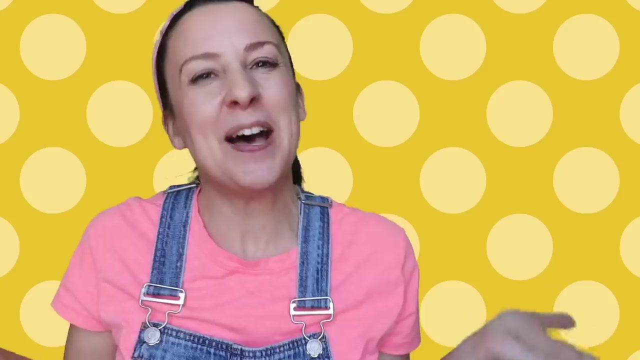 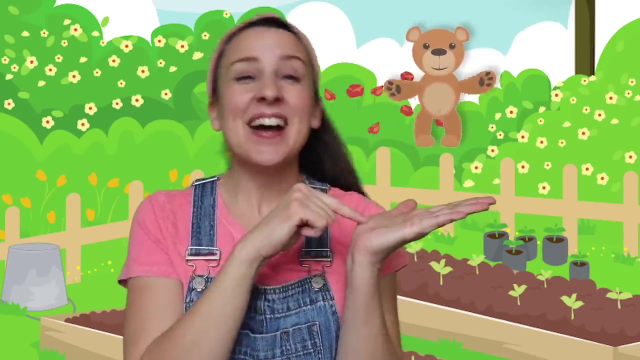 see a crocodile, don't forget to scream: Ah, Look, it's a little pink bunny. Let's say: go and see what happens. Ready set go. Whoa, It popped, It popped up, Pop, pop, pop. That was fun. Round and round the garden. 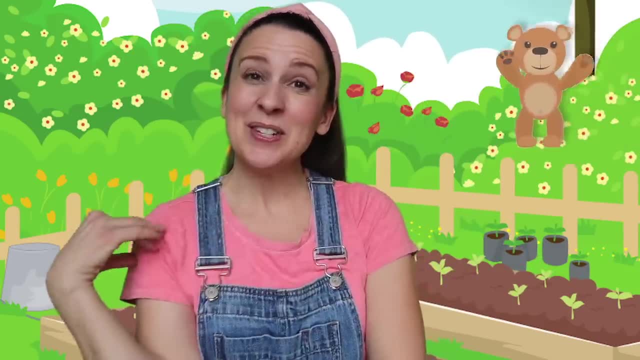 like a teddy bear, One step, two step, tickle you under there Round and round: the garden, the lake, the water, the sea. Let's sing row, row, row your boat gently down the stream. Let's sing row, row, row your boat gently down the stream If you see a crocodile. 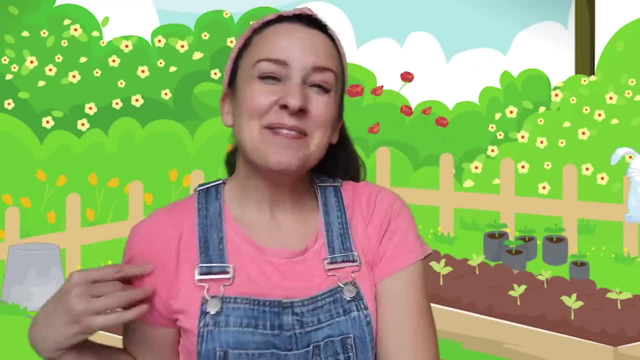 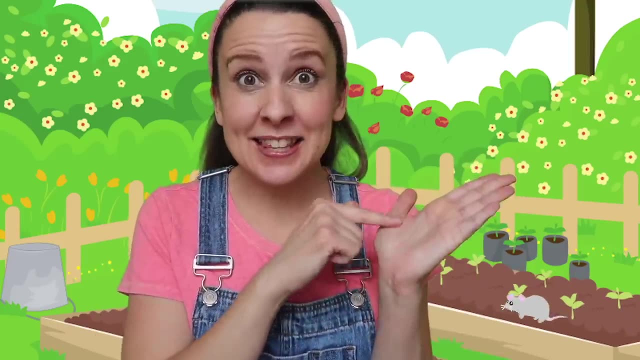 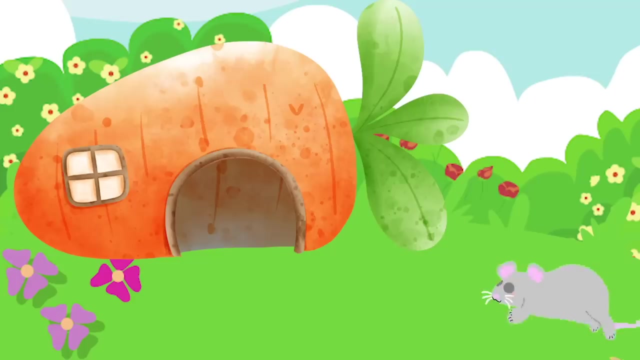 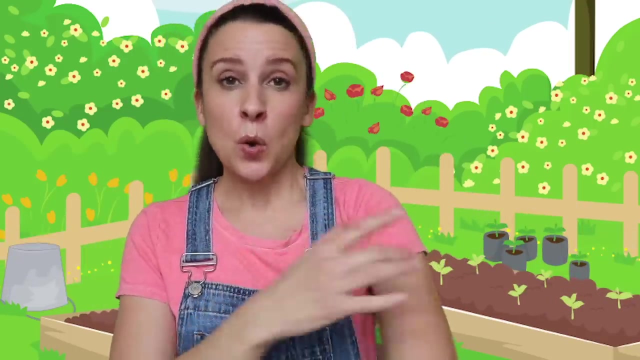 little bunny goes Hippity hop, hippity hop. he's gonna get your nose. Round and round the garden goes the little mouse Scurry scurry, scurry, scurry into his little house. Round and round the garden looking for a hare. Where are we going to find it? Right up there. 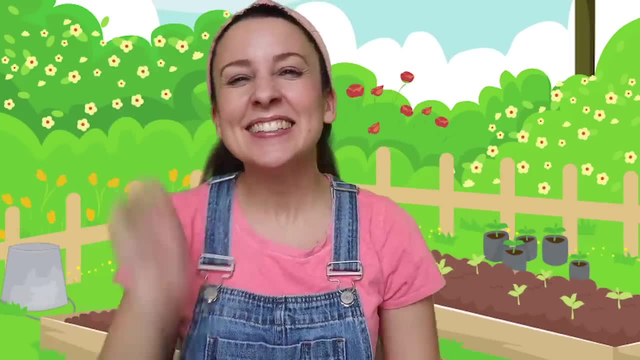 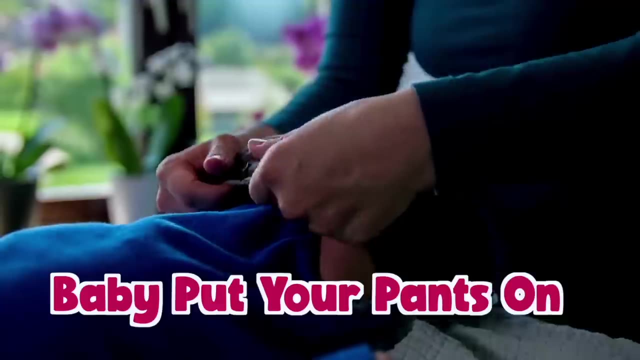 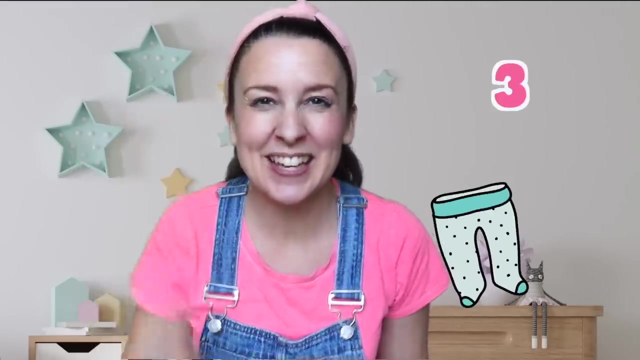 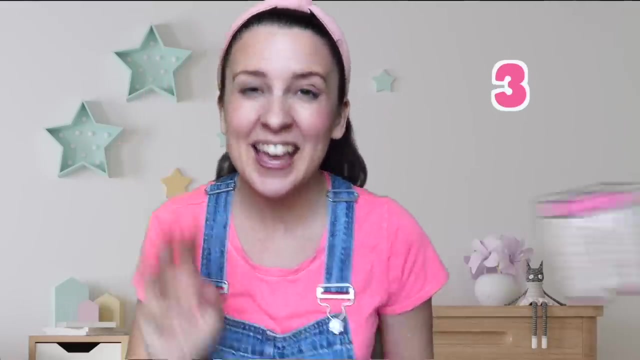 Yeah, right up there. Baby, put your pants on Pants on Pants on. Baby. put your pants on One, two, three. Baby put your pants on Pants on Pants on. Baby. put your pants on One, two, three. Leg to the left leg to the right, Wiggle. 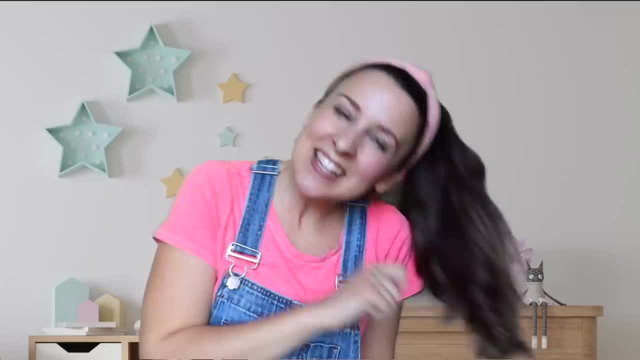 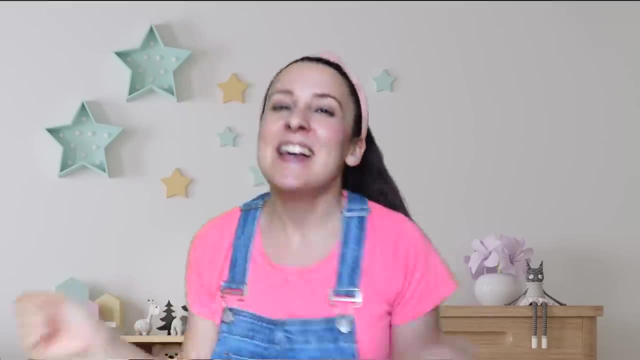 and pull them up tight Leg to the left leg to the right, Wiggle and jiggle and pull them up tight. Baby put your pants on, pants on, pants on. Baby put your pants on One, two. 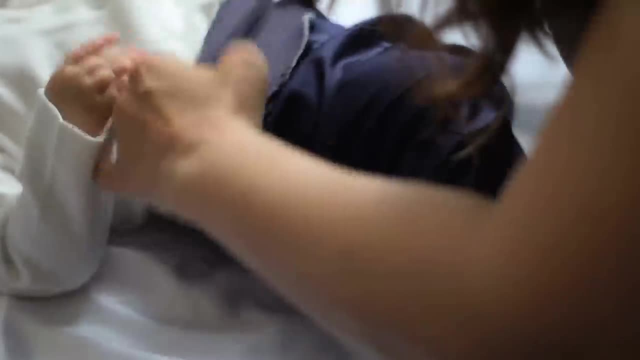 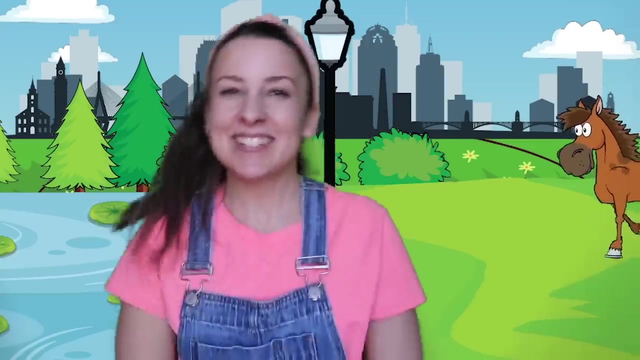 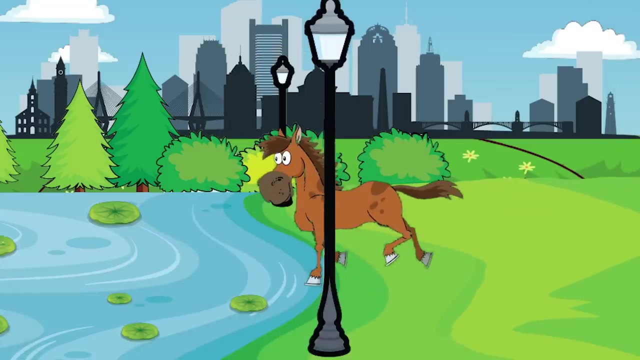 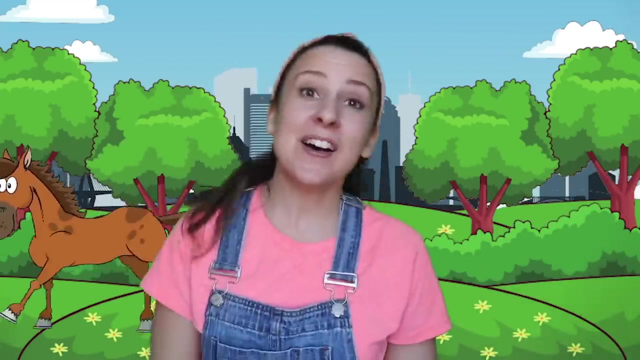 three Baby. put your pants on pants on pants on Baby. put your pants on One, two, three Trot trot to Boston. Trot trot to Lynn. Watch out, baby, or you might fall. Trot trot to Boston. Trot trot to Dover. Watch out, baby, or you might fall over. So. 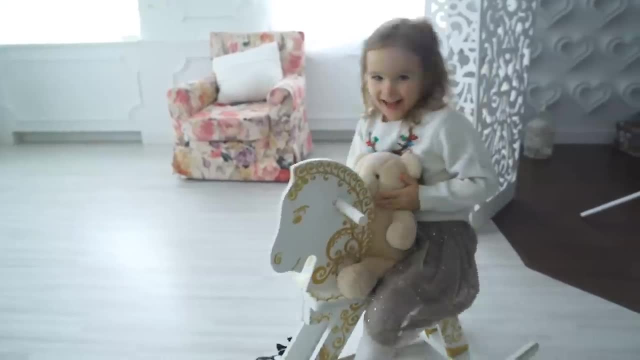 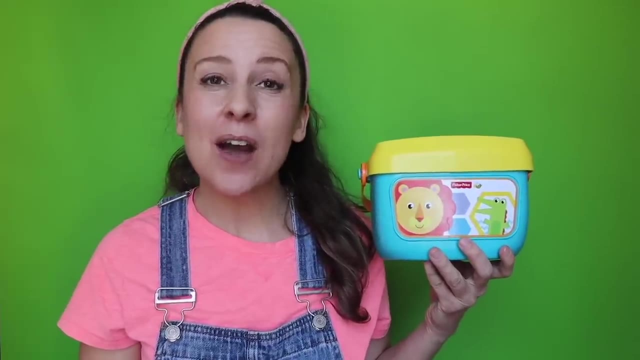 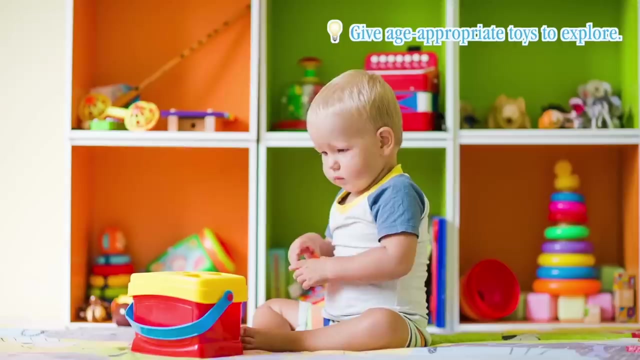 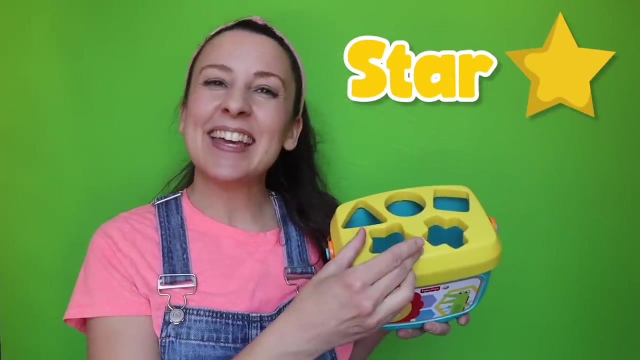 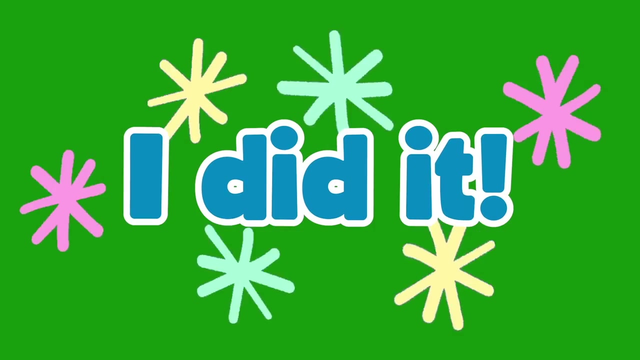 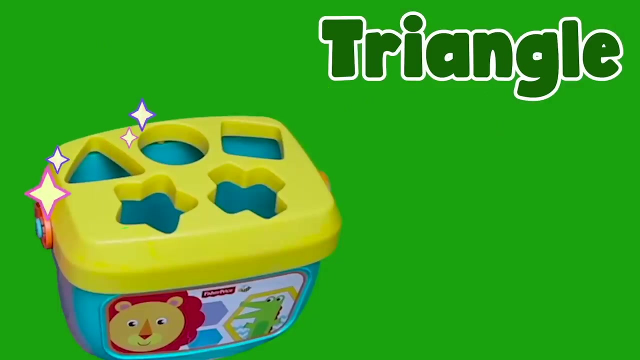 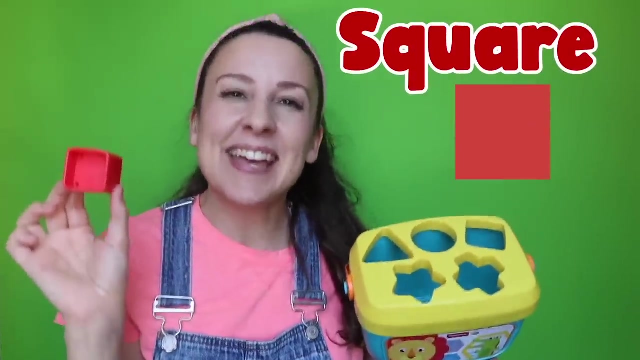 silly, Wow. Can you say wow, Wow, It's a shape sorter. Let's put the shapes in Star, star in. I did it. Can you say I did it? I did it. Triangle, triangle in Square. you say in, Put it in, put it in, put it in. 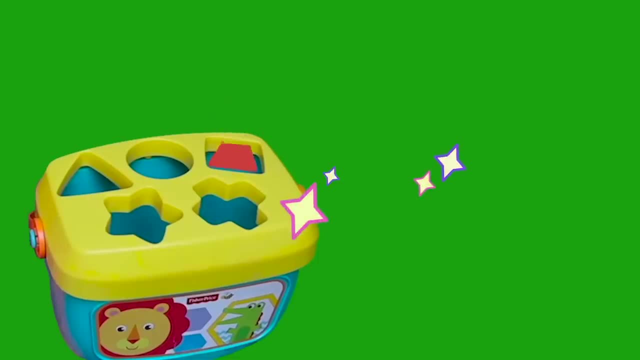 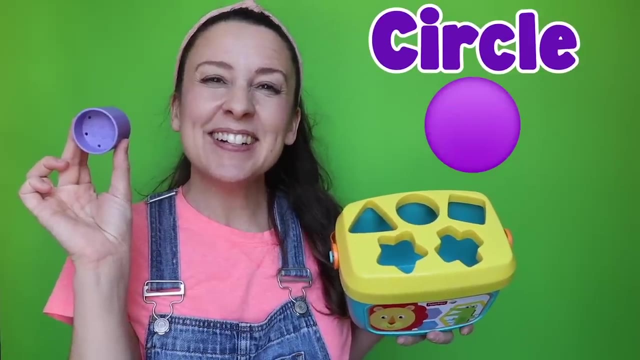 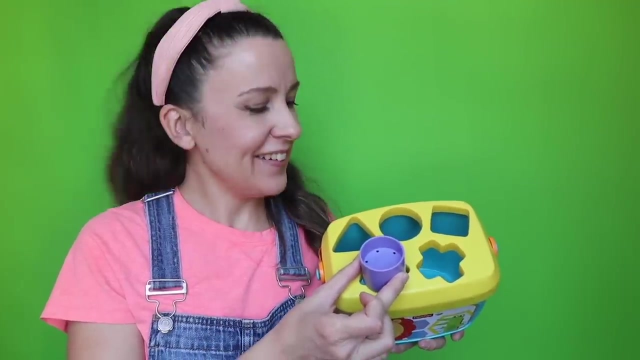 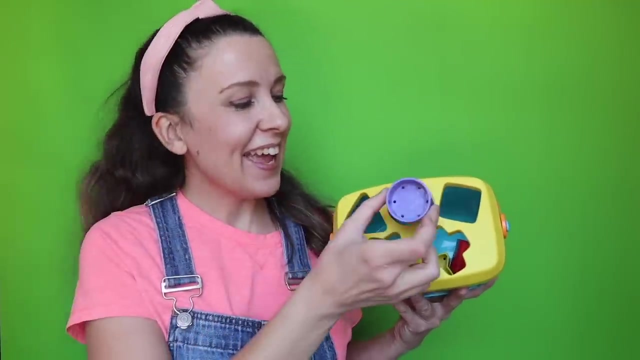 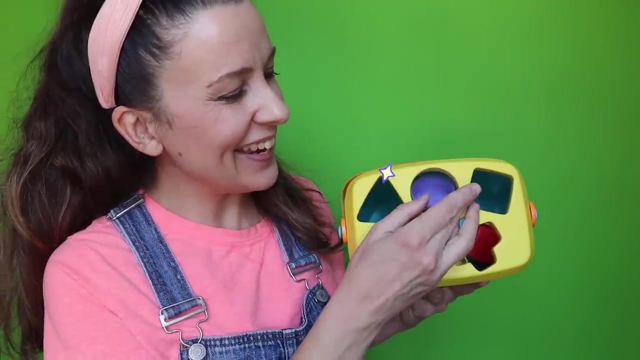 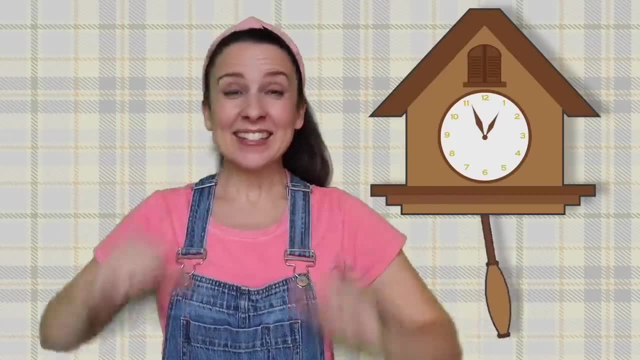 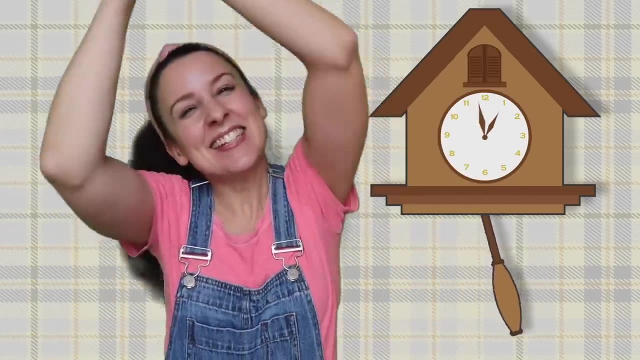 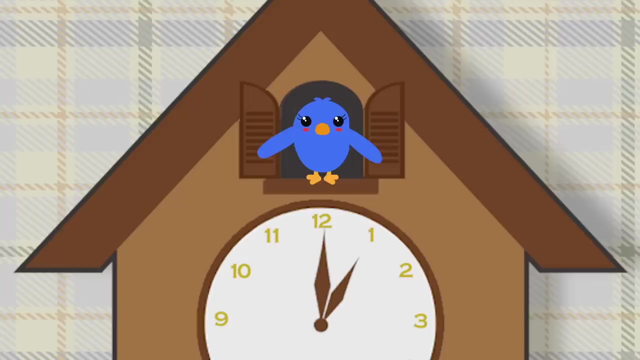 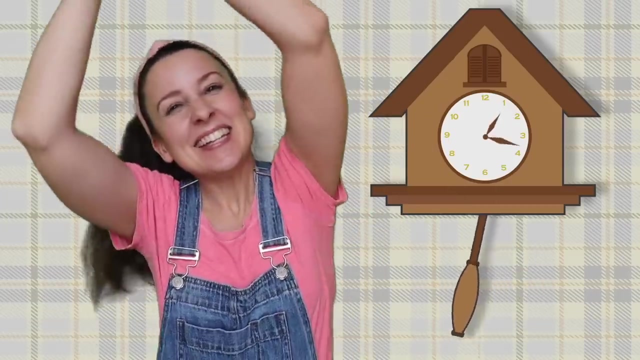 pretend to be a clock with me. Tick tock, Tick tock. I'm a little cuckoo clock. Tick tock, Tick tock. Now I'm striking one o'clock. Cuckoo, Cuckoo. Tick tock, Tick tock, I'm a little. 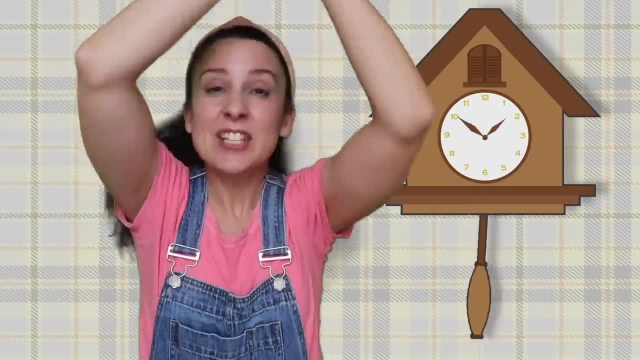 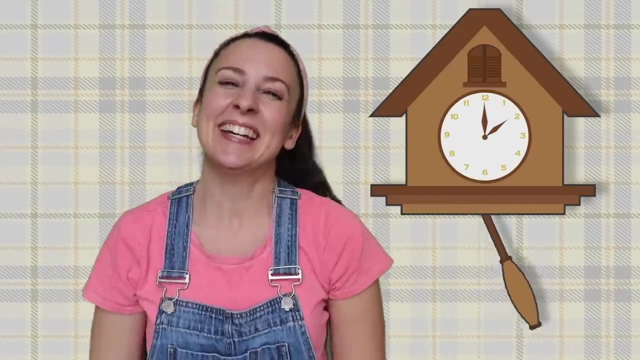 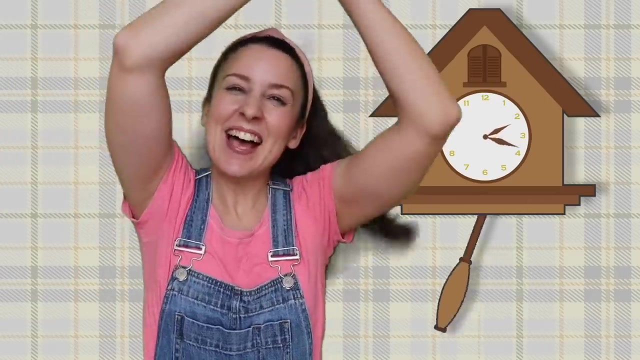 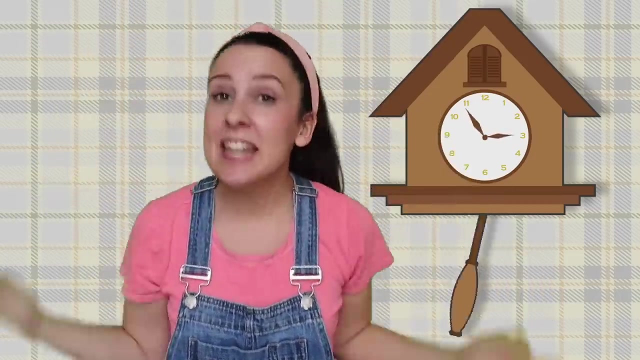 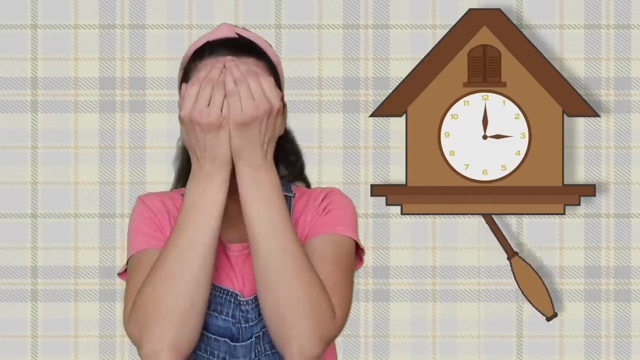 cuckoo clock. Tick tock, Tick, tock. Now I'm striking two o'clock. Cuckoo Cuckoo. Tick tock, Tick tock. cuckoo clock. tick tock, tick tock. now I'm striking 3 o'clock. cuckoo, cuckoo, cuckoo. 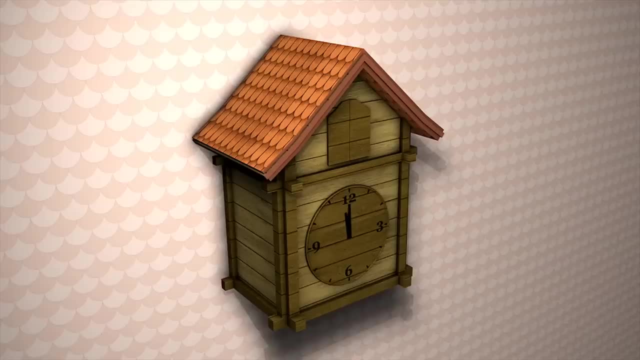 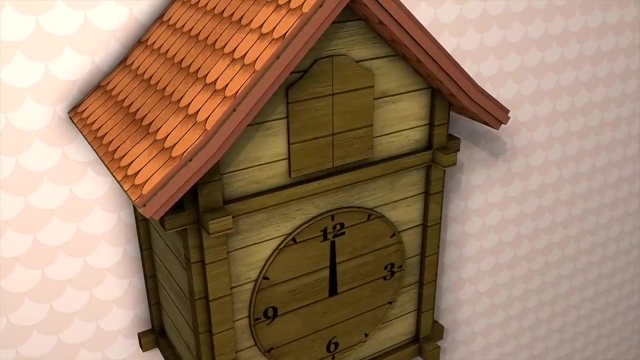 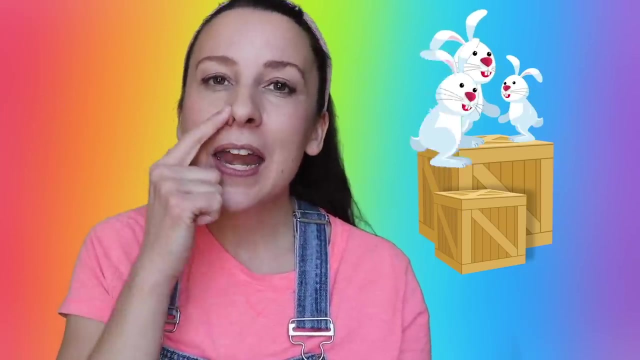 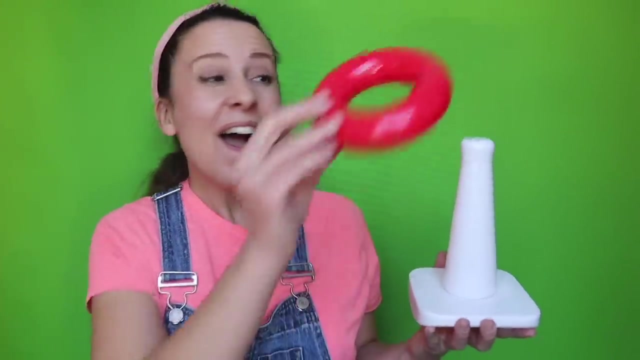 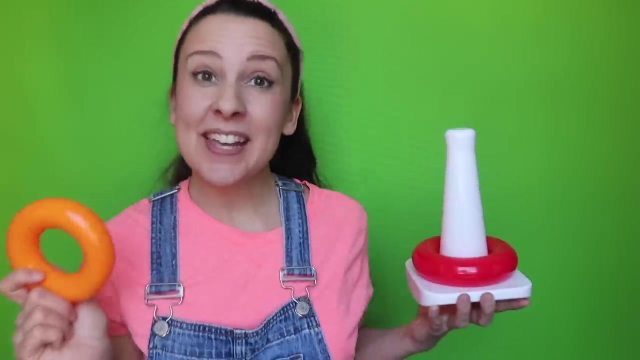 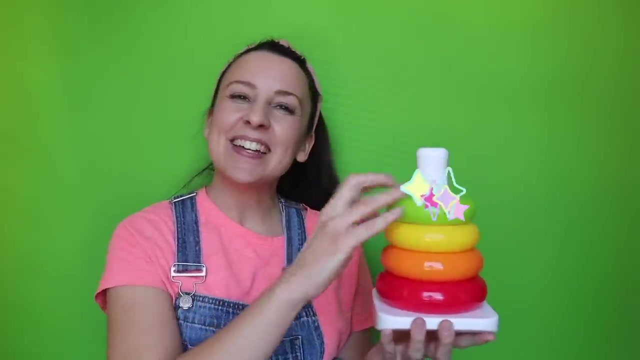 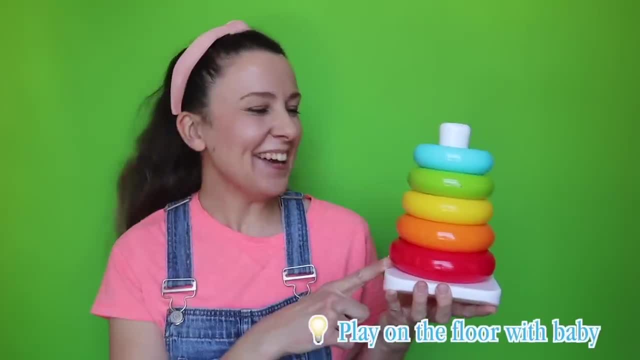 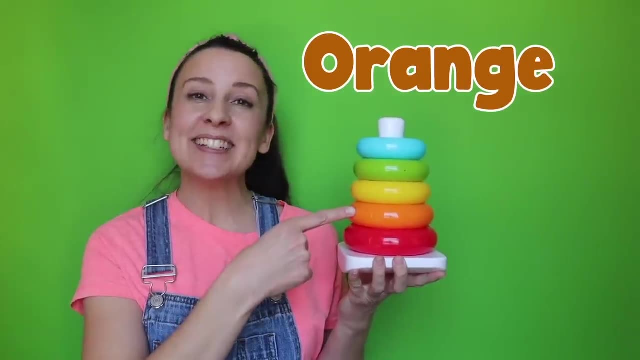 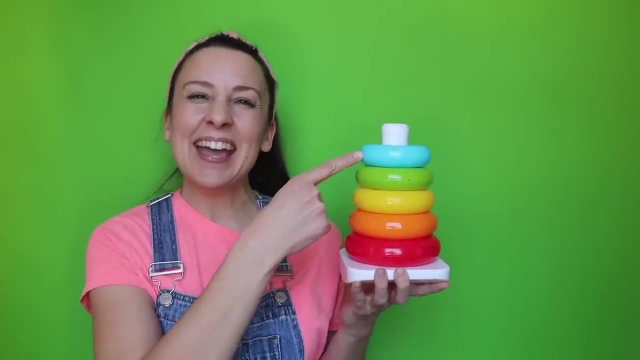 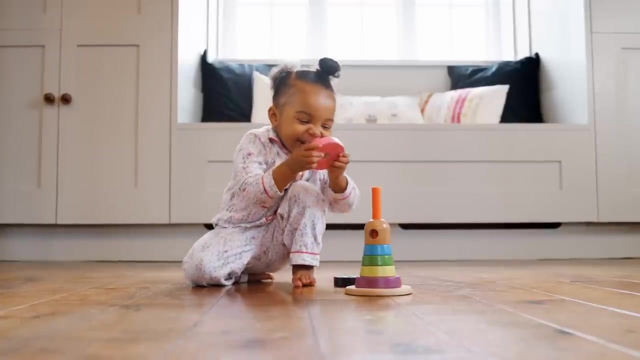 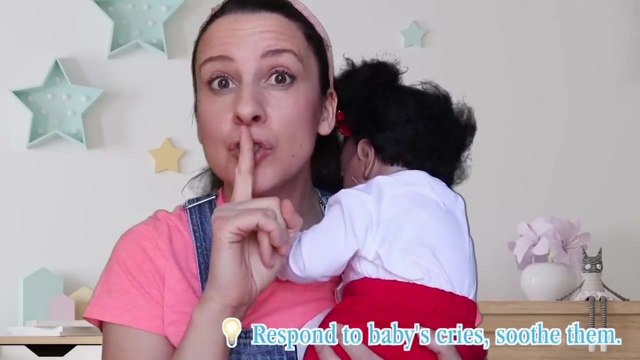 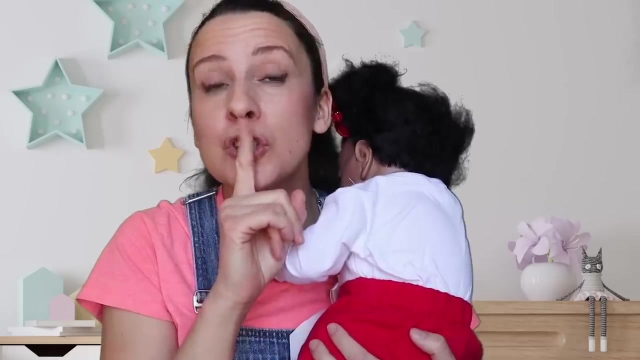 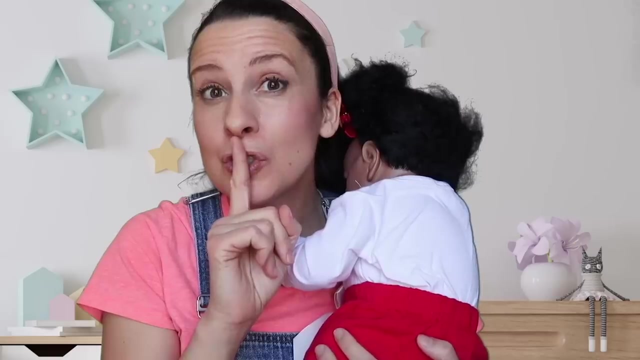 the rings on the stacker. yay, that was fun. let's do the colors red, orange, yellow, green, blue. yay, we did it. shhhh, can you do that? we have to be quiet. the baby is sleepisch. be quiet, the baby is sleeping. shhh, good job, only for today. 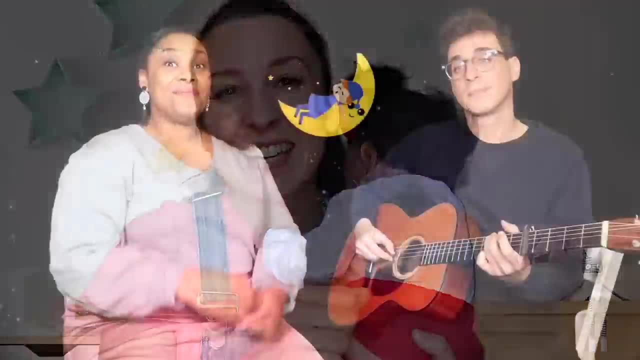 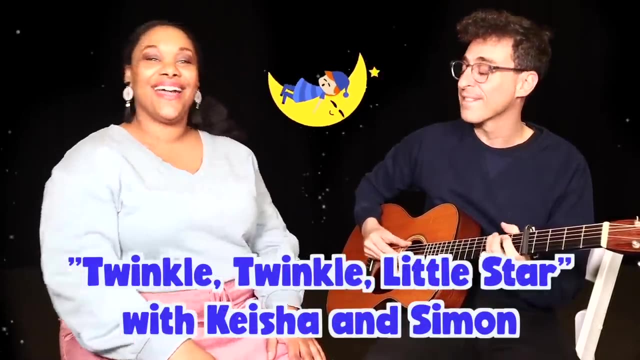 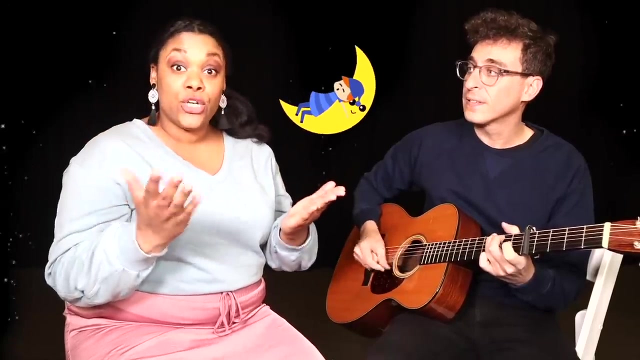 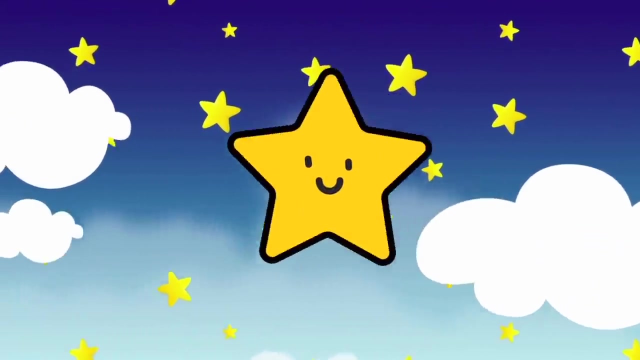 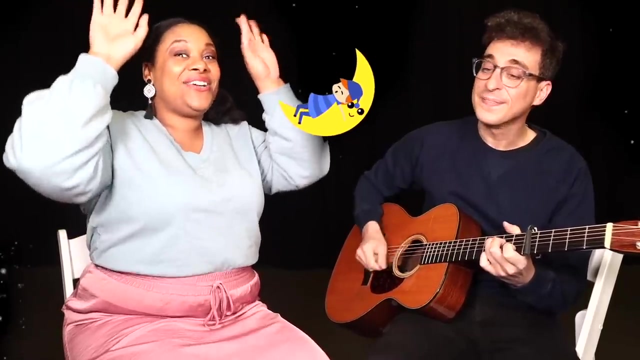 you did it. y'all being quiet, Let's sing Twinkle Twinkle. Will you sing with me? Twinkle twinkle little star, How I wonder what you are, Up above the world so high Like a diamond in the sky. Twinkle twinkle, little star, How I wonder what you are. 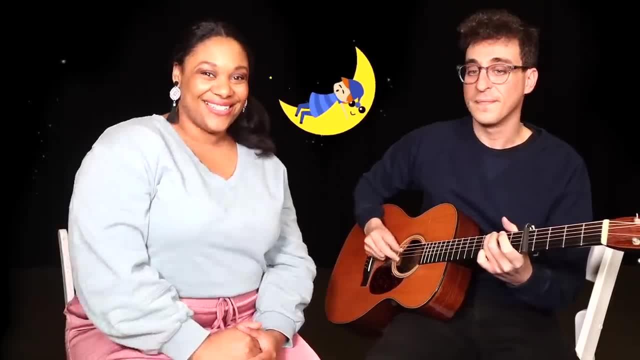 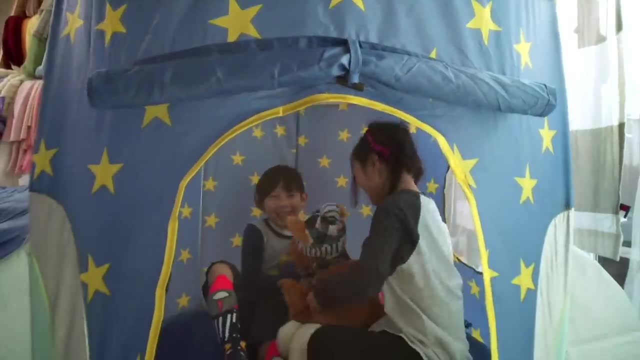 Can you do those twinkle fingers with me? All right, here we go. Twinkle twinkle little star, How I wonder what you are, Up above the world, so high Like a diamond in the sky. Twinkle twinkle little star, How I wonder what you are. 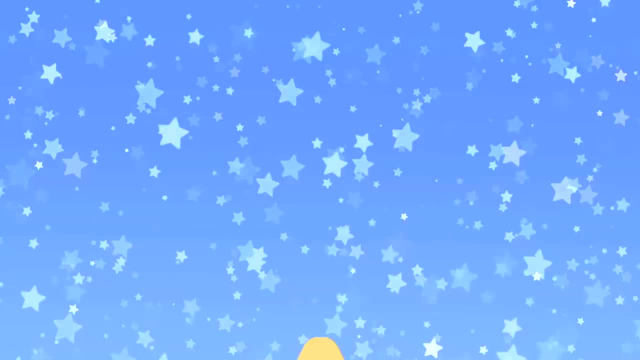 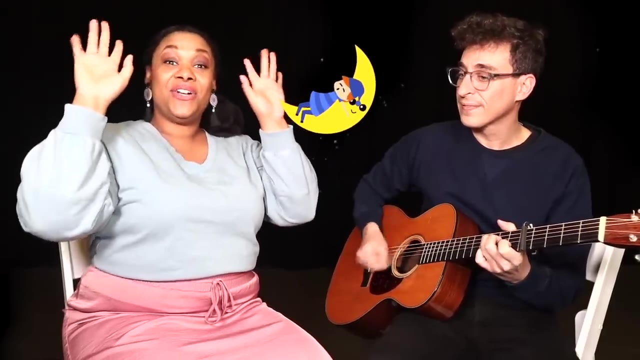 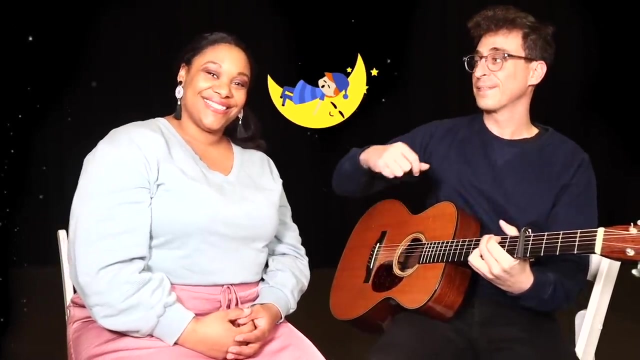 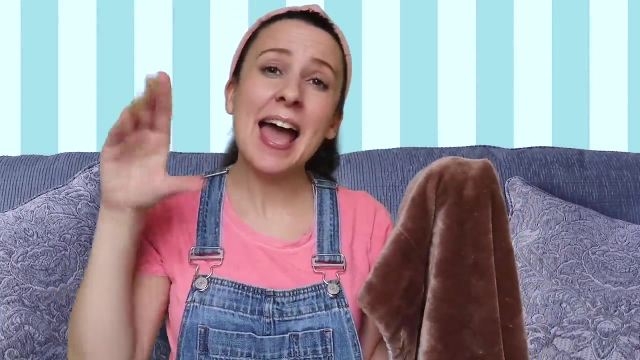 Up above the world, so high Like a diamond in the sky, Twinkle, twinkle little star. How I wonder what you are. Hmm, where is the apple? Where is the apple? Hmm, do you think it's under the blanket? 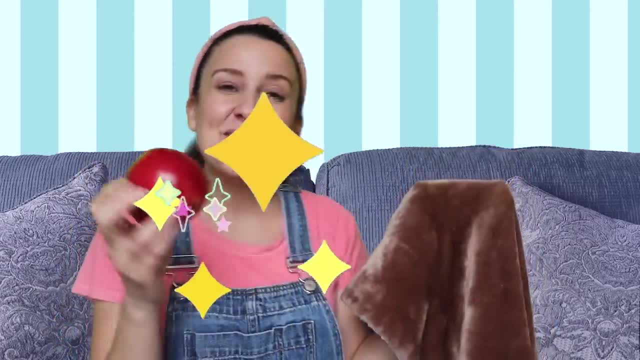 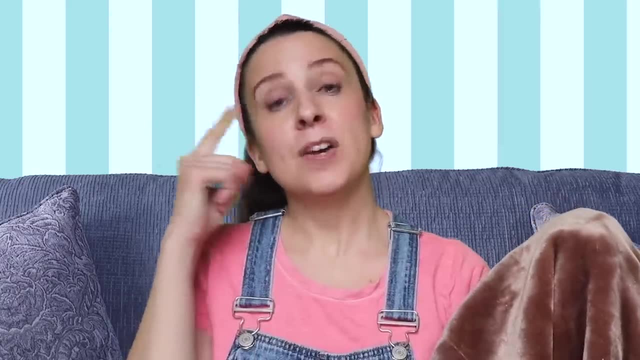 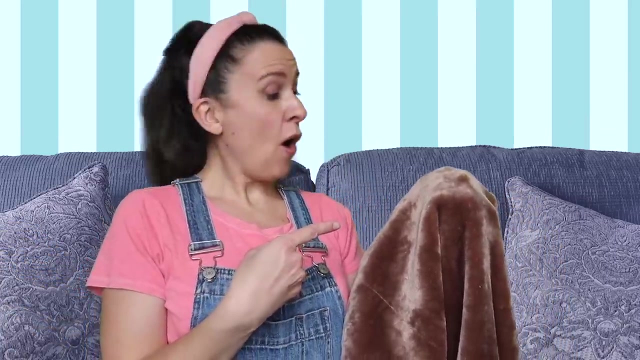 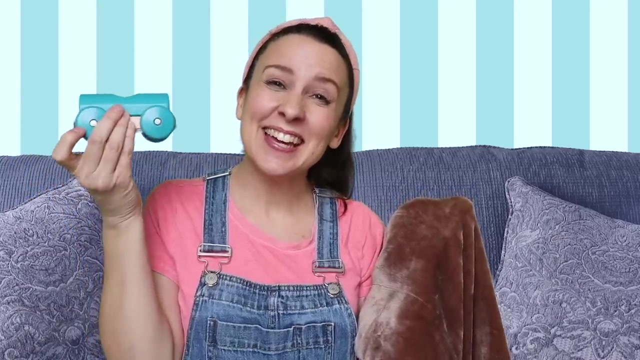 Let's check. Oh wow, the apple was under the blanket. Hmm, where is the car? Hmm, where is it Under the blanket? Let's check. Oh, vroom, vroom, The car was under the blanket. We found it. We found the car. 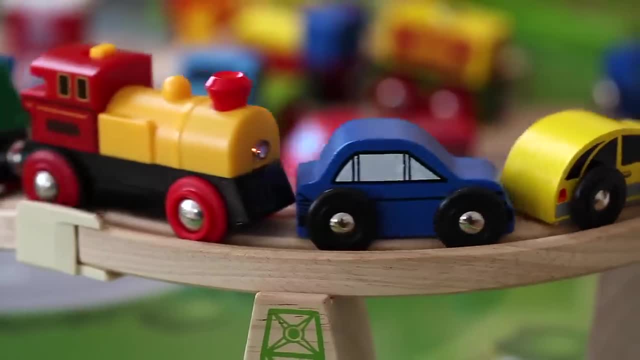 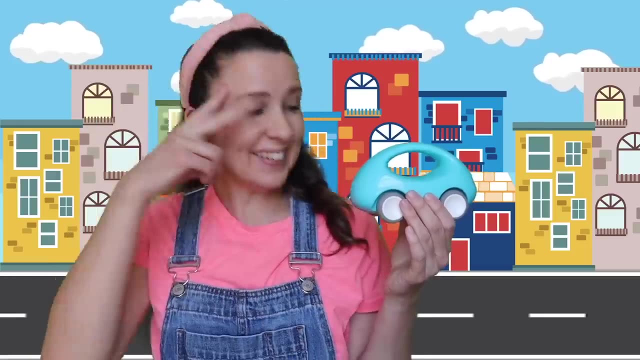 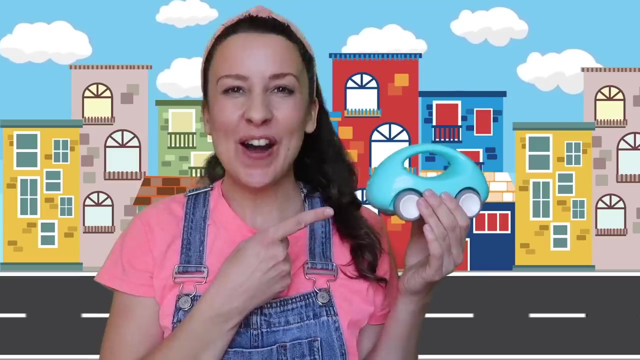 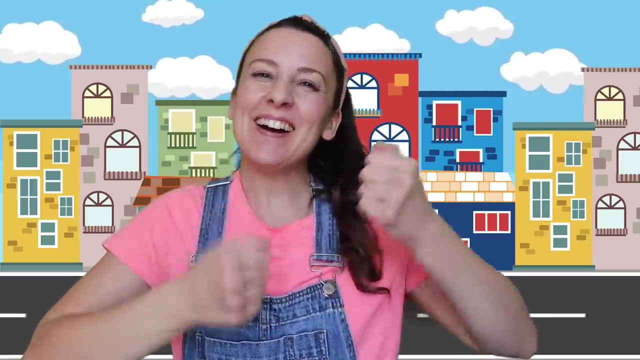 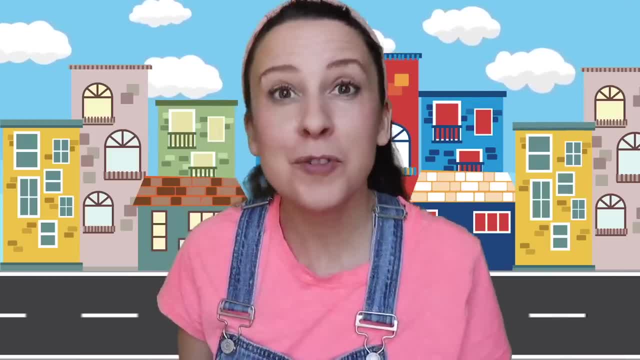 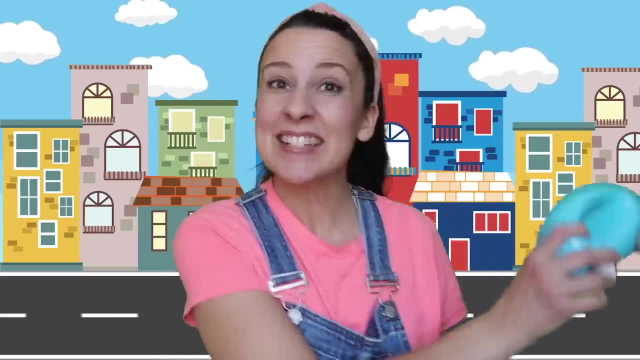 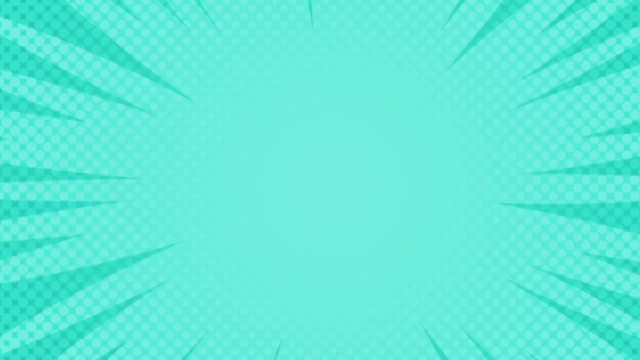 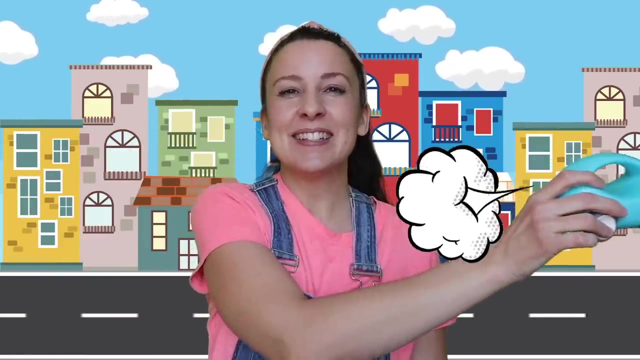 Vroom, vroom and the car will come out. Vroom, vroom, vroom. Here it is. Vroom vroom, vroom, Going fast, So fast, Fast. Now it's going slow, Slow car, Slow car, Bye, bye, car Say. 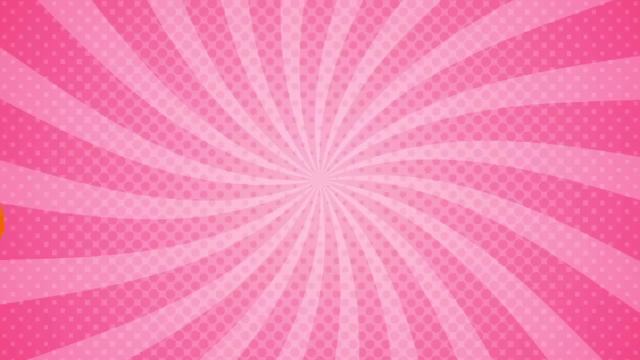 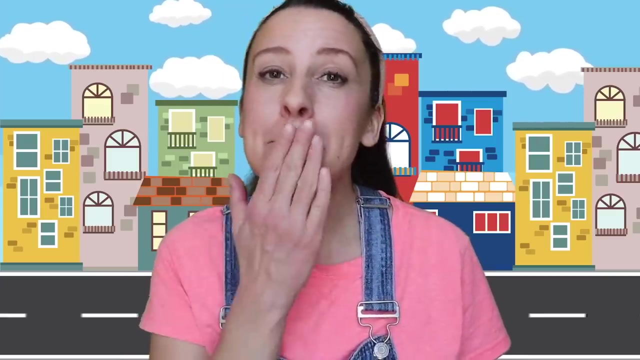 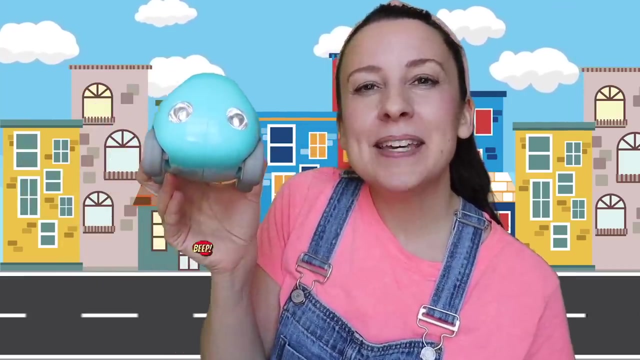 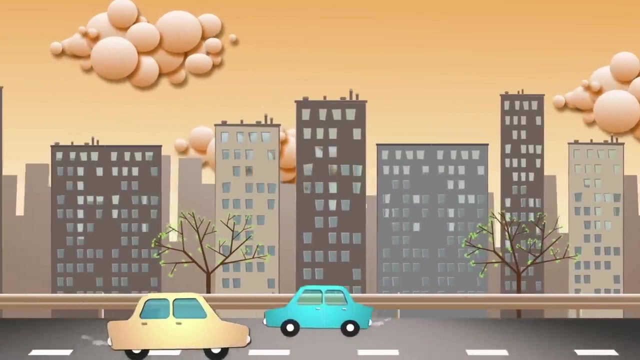 bye, bye to the car, Bye bye, car. Can you say: beep, beep, Beep, Beep. Here comes the car, Beep, beep, Beep, beep, Beep, beep, Driving away. Hey, do you see who I have with me? 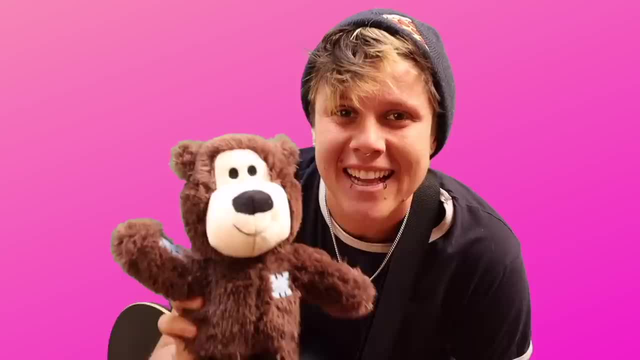 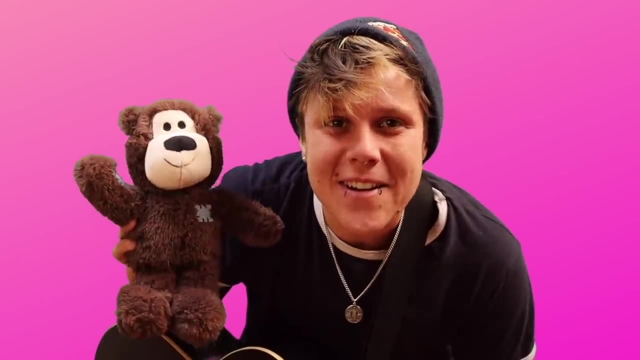 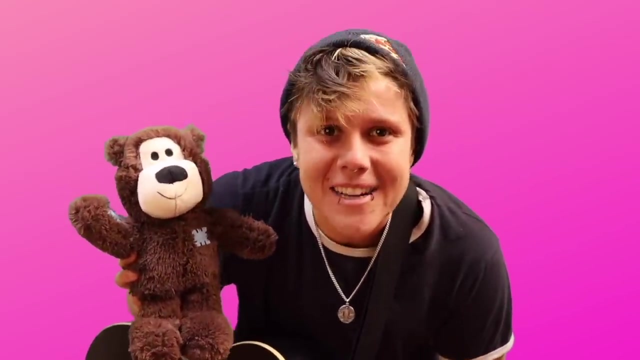 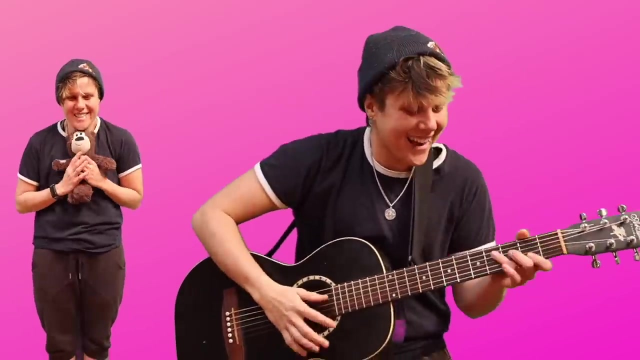 Yeah, it's my stuffy. Their name is Patches. Hi, We're going to be doing a song with our stuffies. Can you go get your stuffies so that we can sing along? Okay, awesome, You can follow along with the jewels right up here. Okay, let's go. 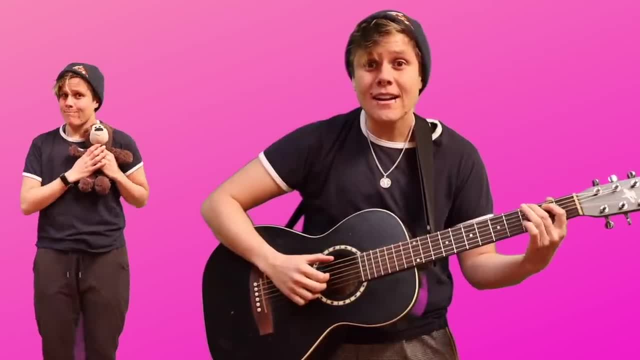 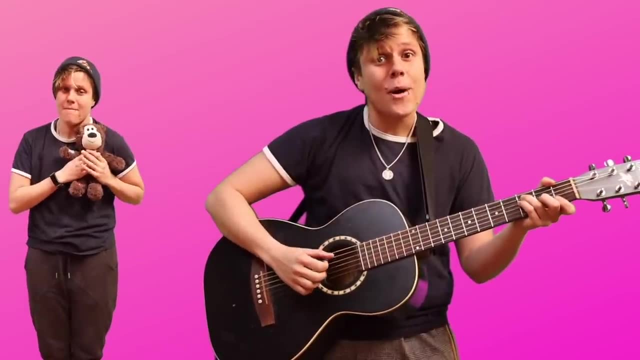 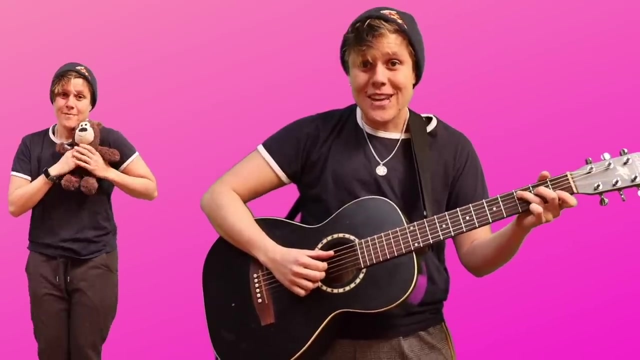 Put your stuffy on your heart, on your heart. Put your stuffy on your heart, on your heart. Put your stuffy on your heart. What a lovely way to start. Put your stuffy on your heart, on your heart. Put your stuffy on your knees, on your knees. Put your stuffy on your knees. 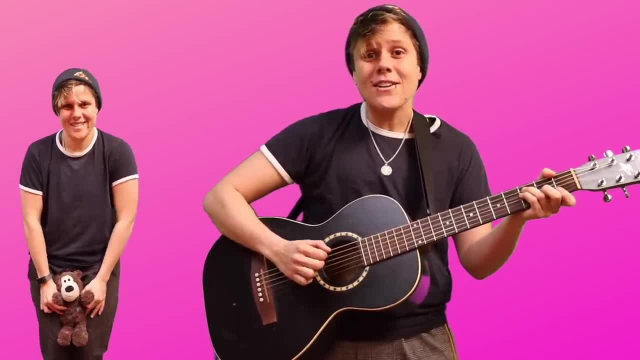 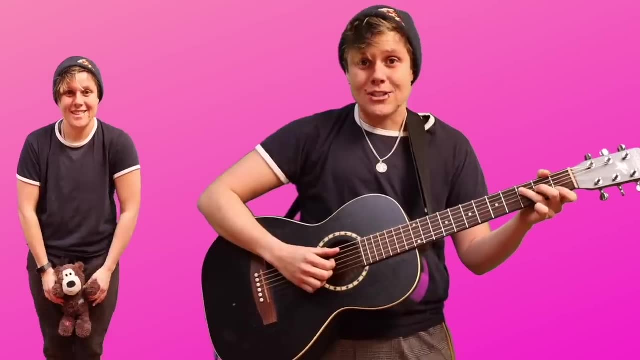 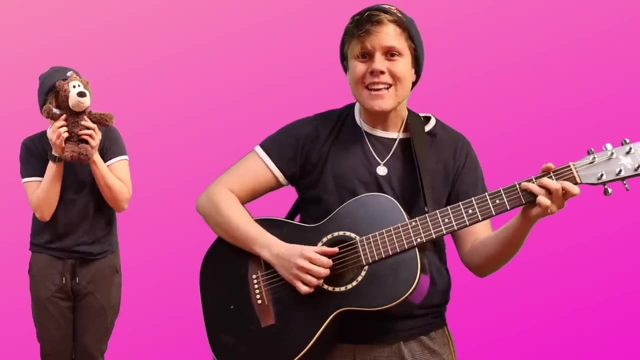 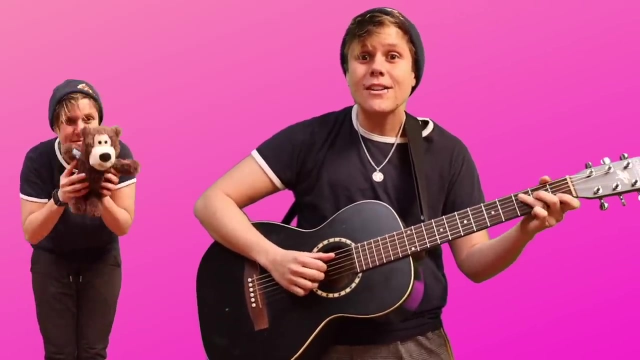 on your knees. Put your stuffy on your knees and you'll both be filled with glee. Put your stuffy on your nose on your nose. Put your stuffy on your nose on your nose. Put your stuffy on your nose. then move it to your toes. Put your stuffy on your nose- on your nose Put. 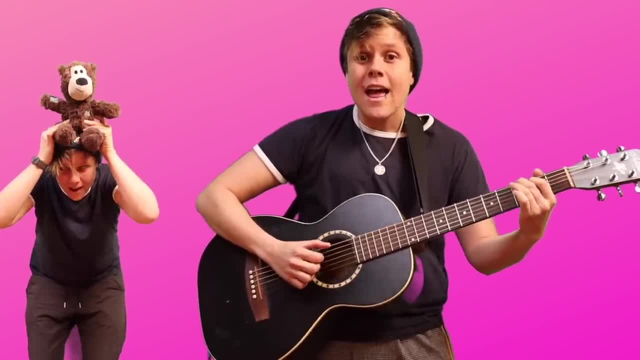 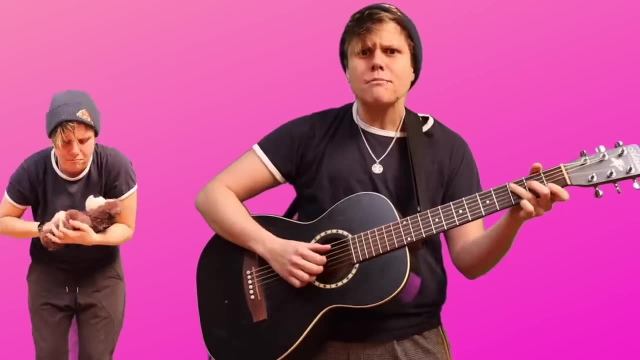 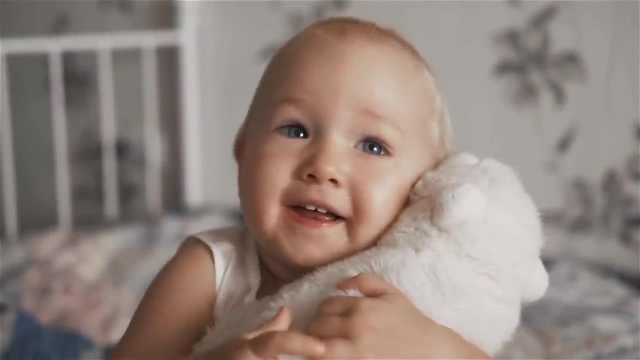 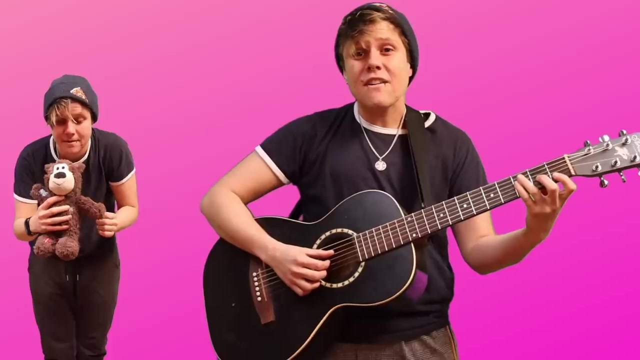 your stuffy on your head on your head. Put your stuffy on your head on your head. Put your stuffy on your head. then put them straight to bed. Put your stuffy on your head on your head. Give your stuffy a big, big hug. Give your stuffy a big, big hug. Give your stuffy a. 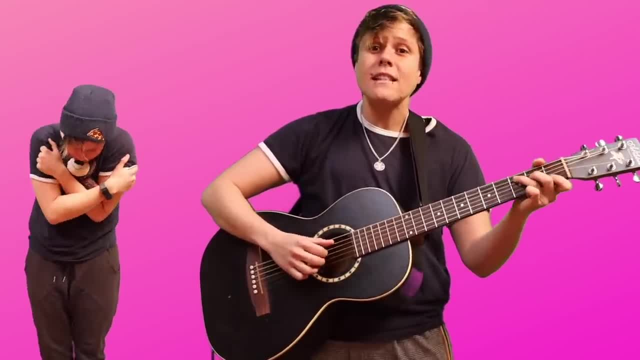 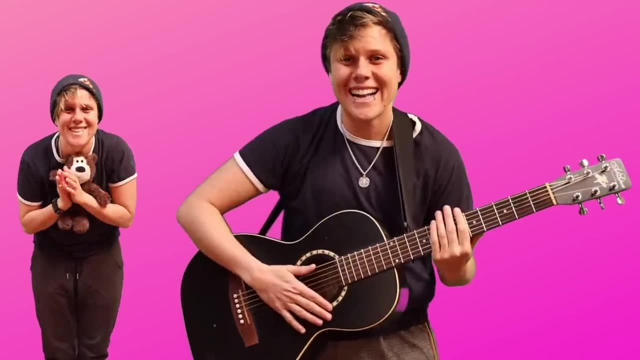 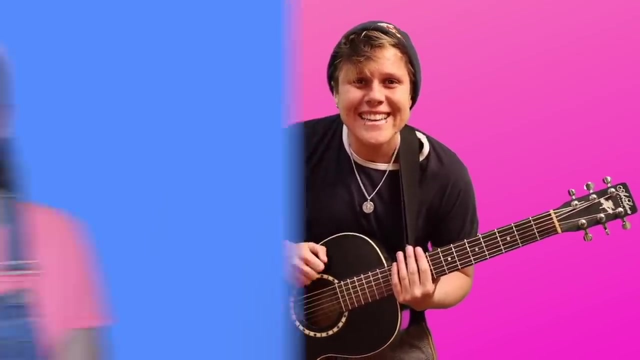 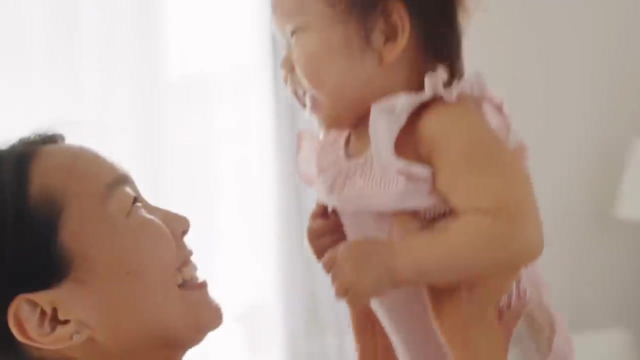 big big hug. Make them feel so safe and loved. Give your stuffy a big big hug. Yeah, Aw, thanks for doing that song with me. Bye stuffy, Bye friend. Acabaca soda cracker. acabaca boo. Acabaca soda cracker, up goes you, Acabaca soda cracker. 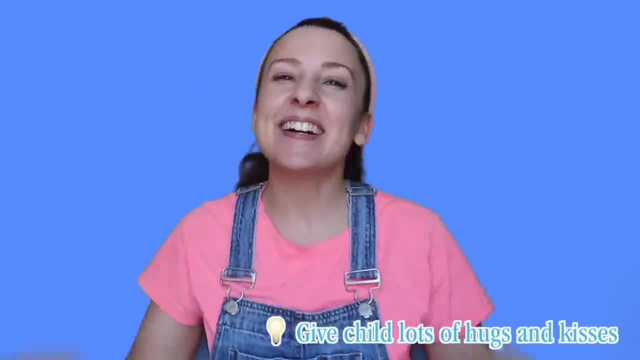 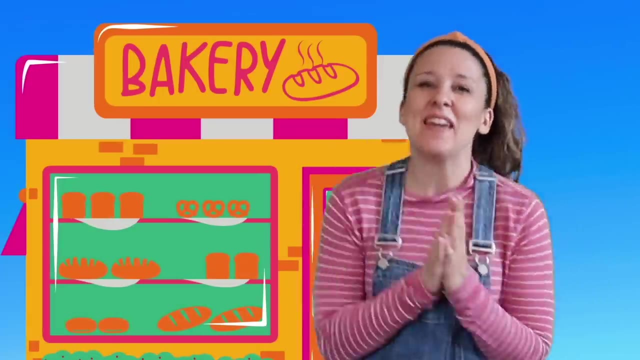 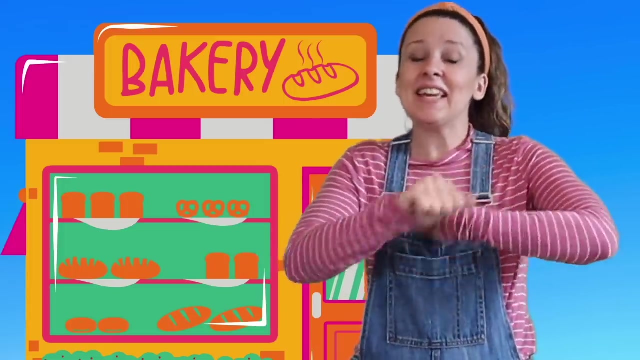 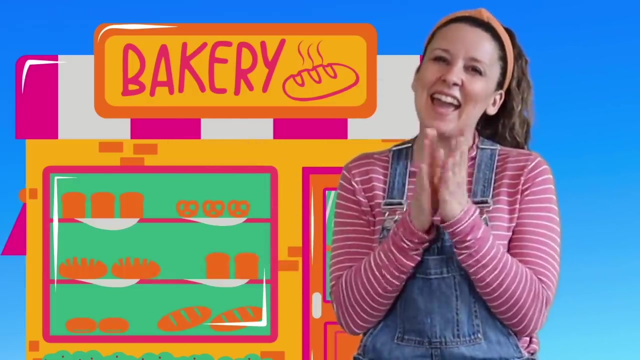 acabaca boo, Acabaca soda cracker. I love you. Yay, Patty cake, patty cake, baker's man, Bake me a cake as fast as you can. Pat it, pat it, pat it, Roll it, mark it with a, B and put it in the oven for baby and me, Yay. 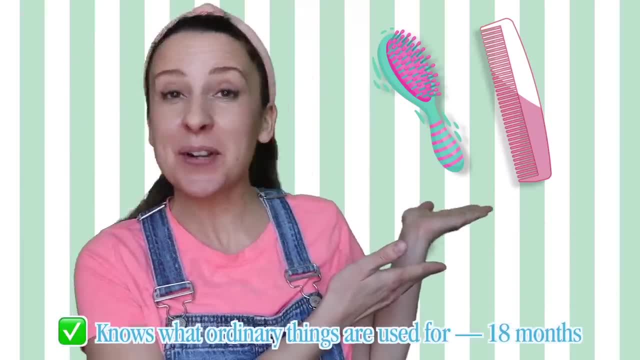 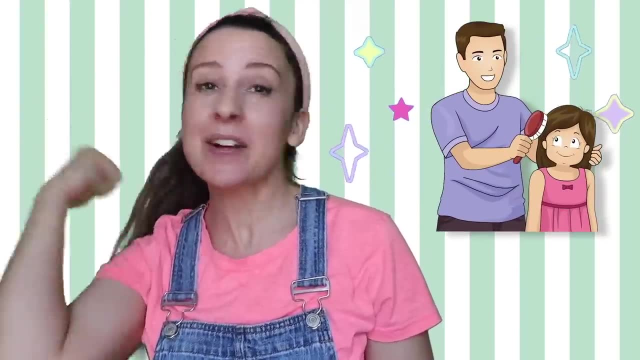 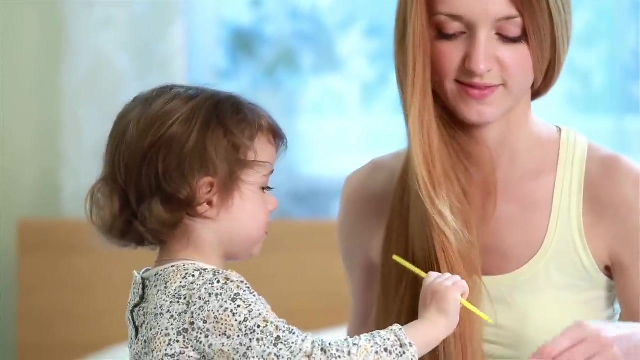 What do we do with a brush or a comb? Yeah, we brush our hair. When our hair is messy, we brush it, Good job. What do we do with a phone? Yeah, we talk on the phone. Hello, Hi mommy. 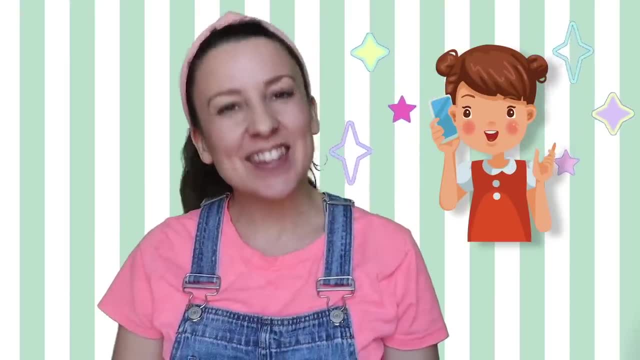 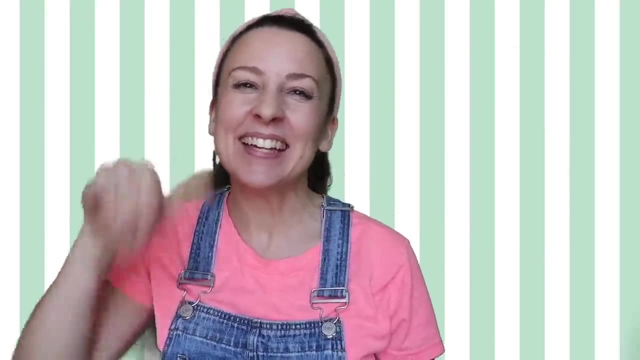 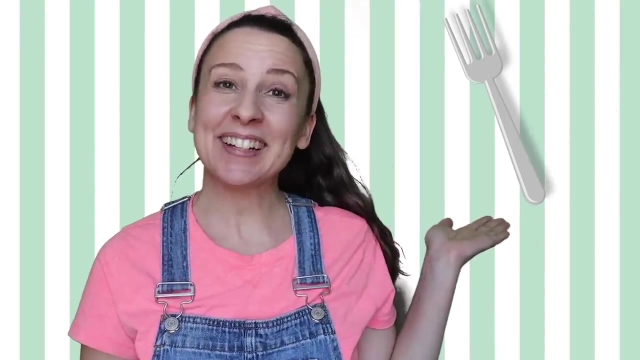 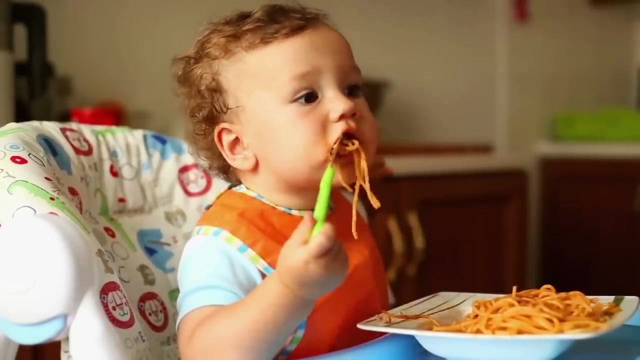 How are you? Bye-bye, Mmm. What do we do with a fork? Yeah, we eat with a fork. Eat with a fork, We eat with a fork. Nice, Now sit back and sit on your bed. Next, put your whole hand up, Put your. 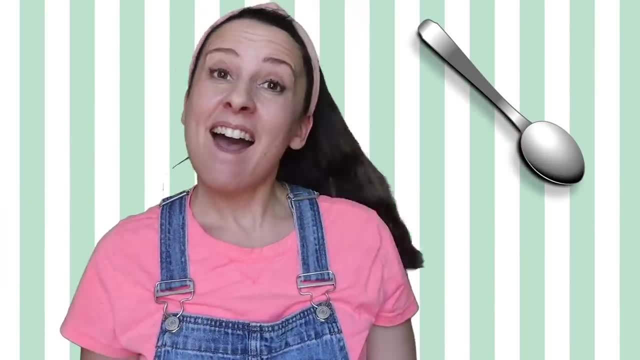 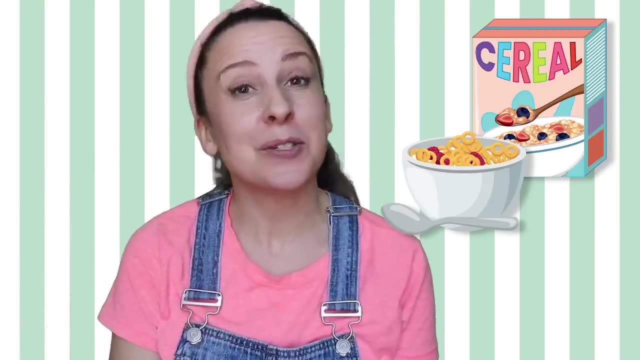 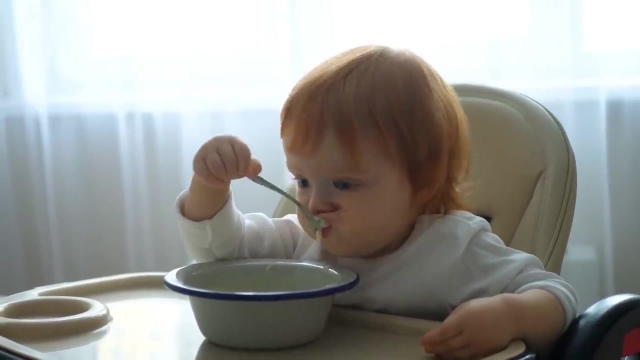 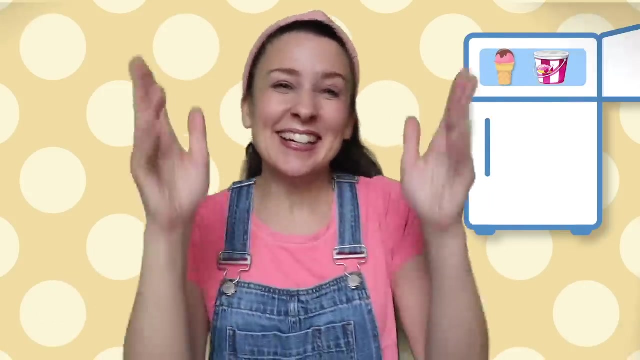 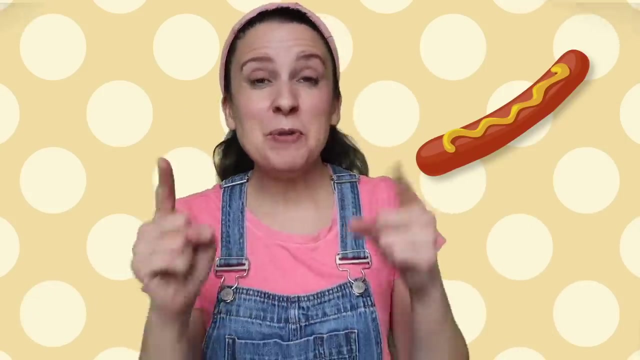 What do we do with a spoon? We eat with a spoon, Maybe cereal or soup, Good job. You be the ice cream and I'll be the freezer. You be the lemon and I'll be the squeezer. You be the hot dog and I'll be the bun. You be the baby and we'll have. 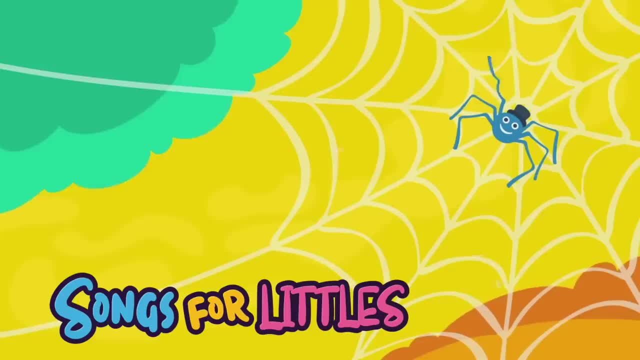 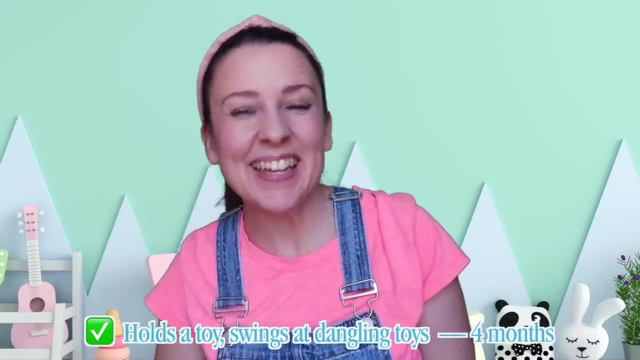 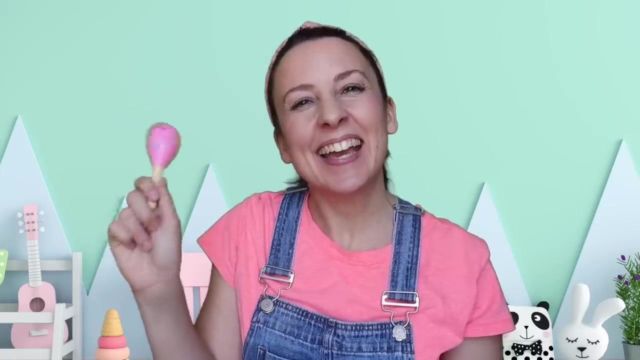 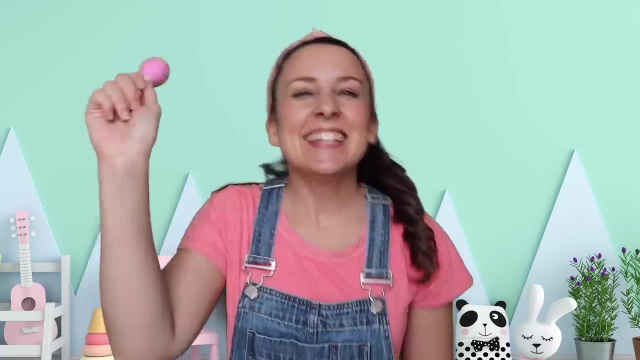 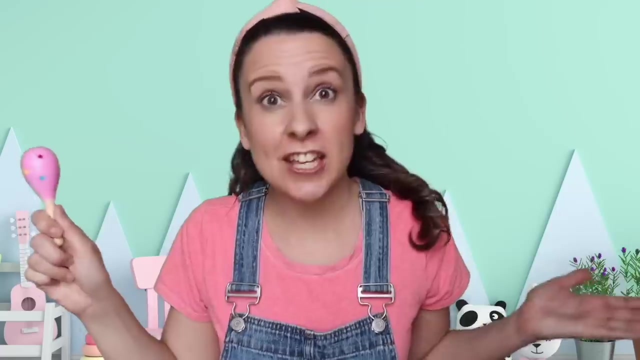 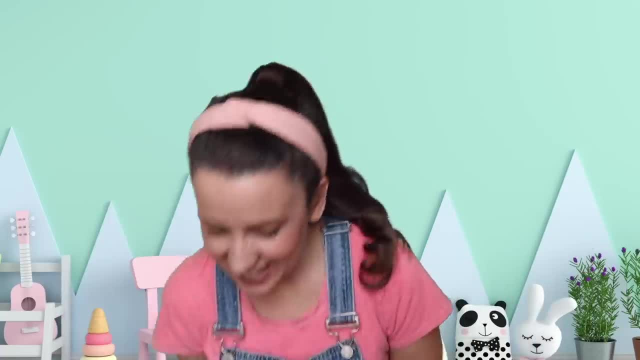 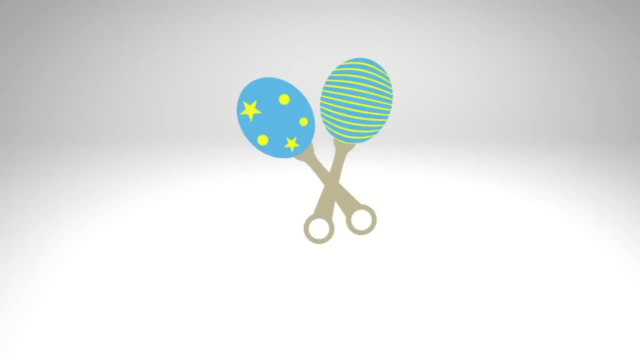 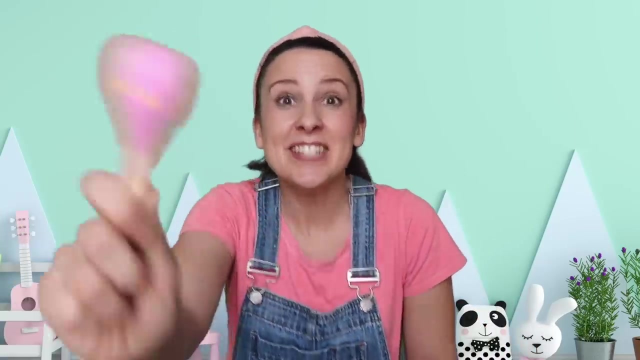 Shake your shaker. Shake it high and shake it low. Shake it yes, shake it no. Shake it high and shake it low. Shake your shaker, Shake it near and shake it far. Drive your shaker like a car. Shake it near and shake it far. Shake your shaker. Shake your shaker. 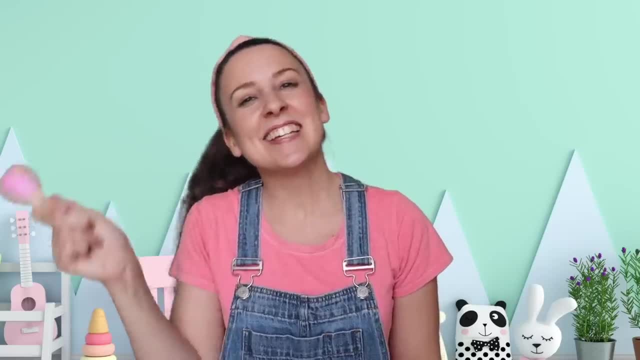 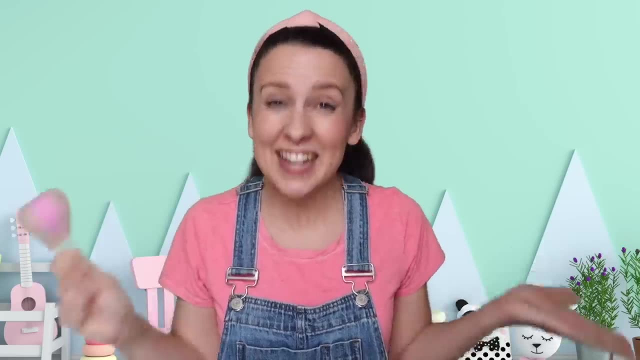 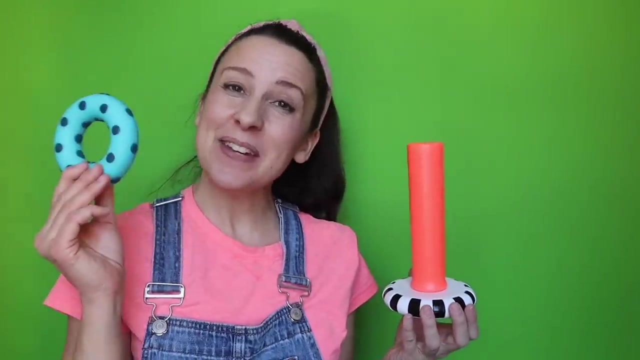 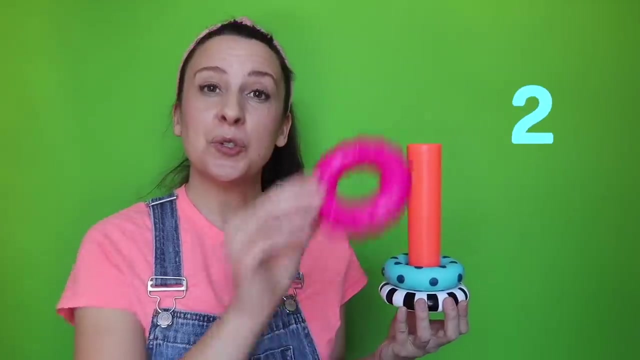 Shake your shaker. Shake it fast and shake it slow. Shake it stop. shake it go. Shake it fast and shake it slow. Shake your shaker. Great job shaking your shaker. Let's see how many rings we have: One, two, three, four, five, six, seven, eight, nine. 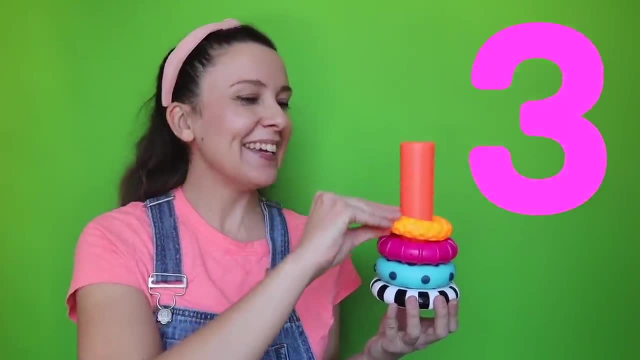 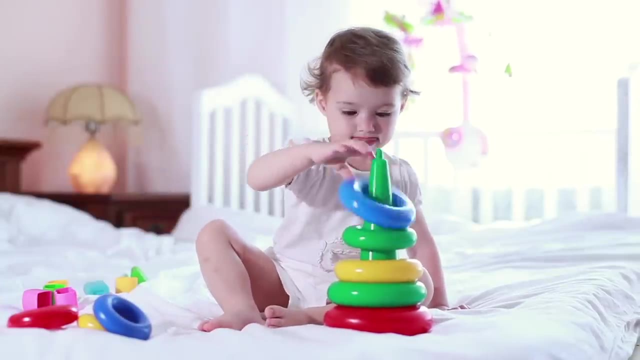 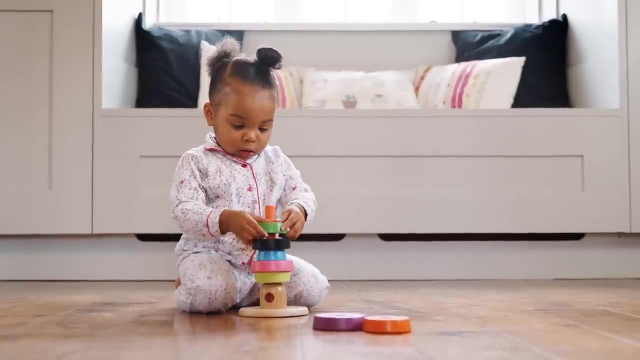 twelve, 13,, 14,, 15,, 16,, 17,, 18,, 19,, 20.. Let's see how many rings we have: One, two, three, four, five, six, 17,, 18,, 19,, 20.. 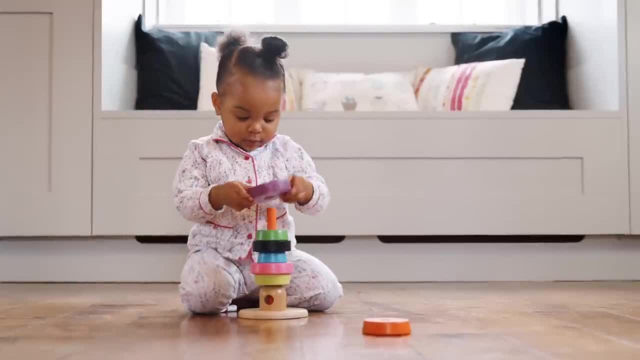 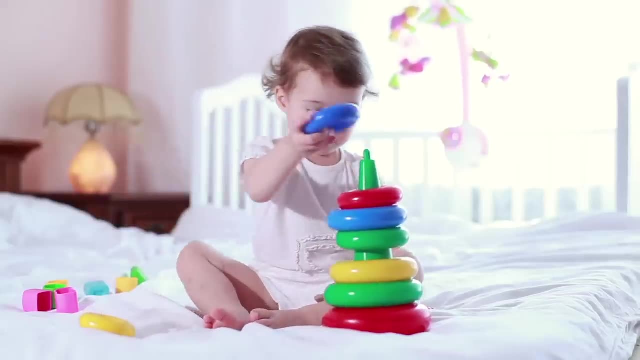 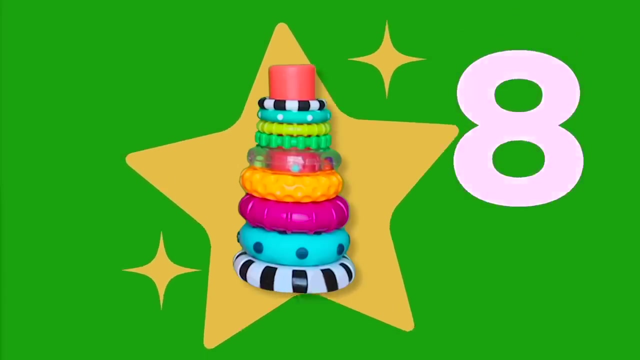 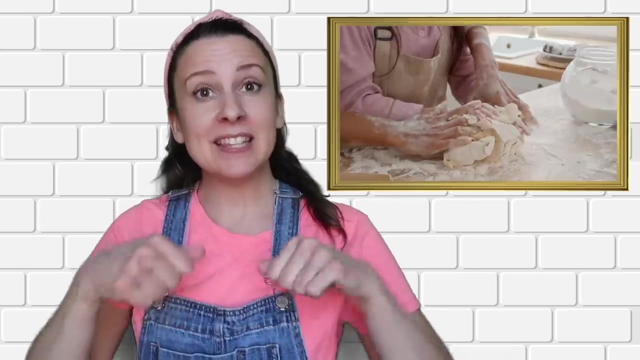 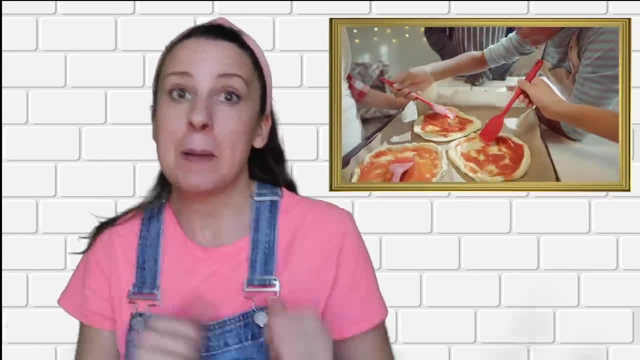 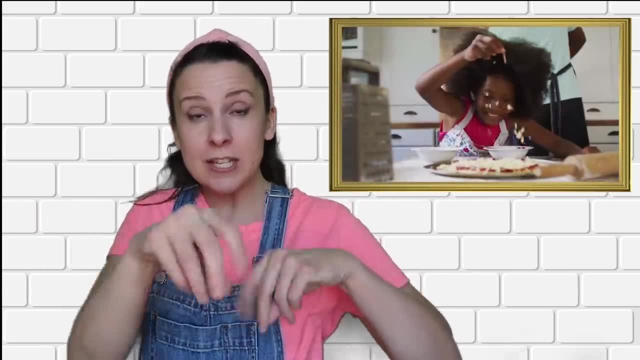 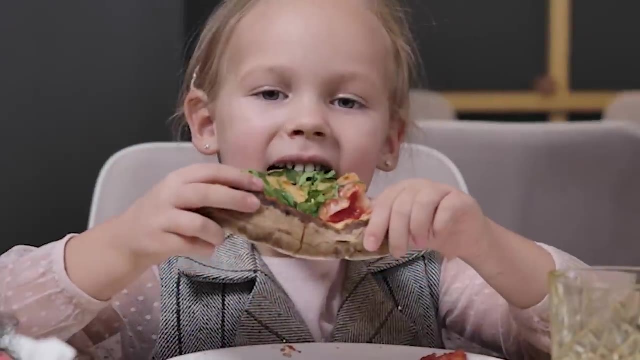 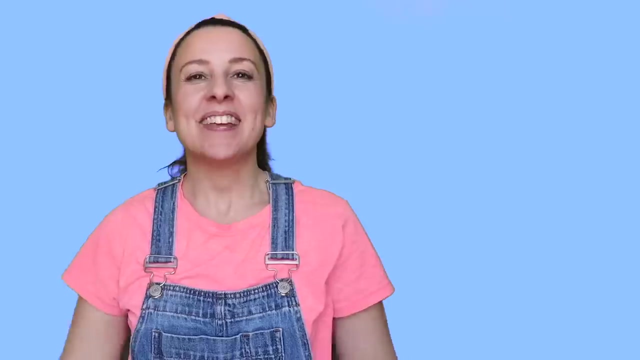 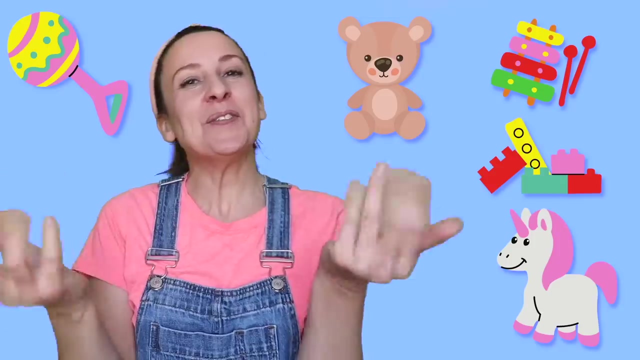 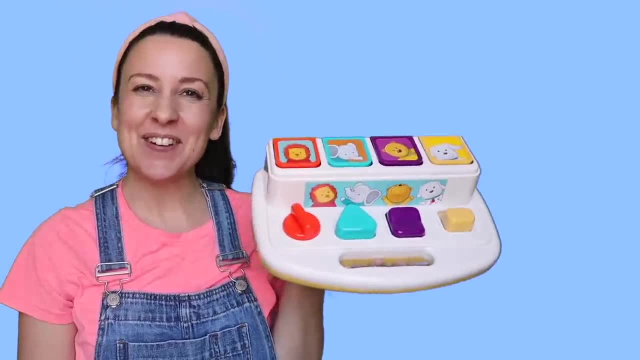 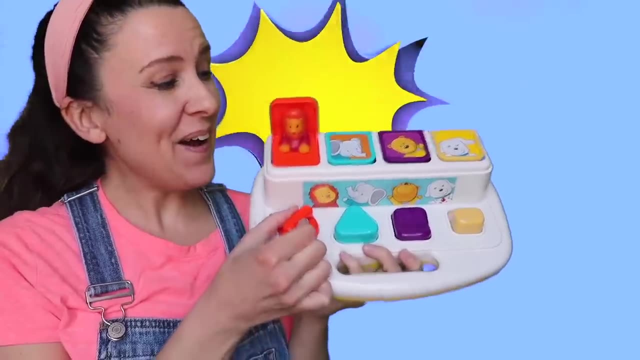 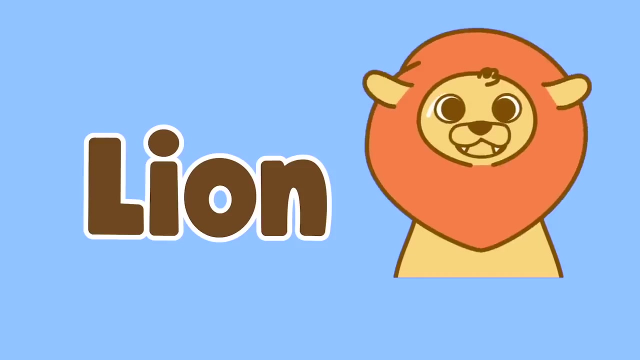 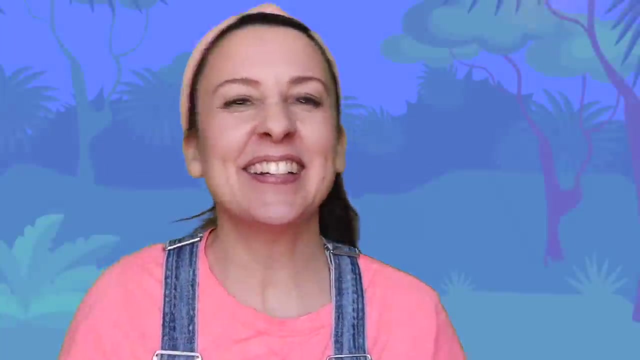 Let's play with this toy. You say pop, and we'll see what happens. Pop, Oh wow, A lion popped up. A lion popped up. Can you pretend to be a lion Roar? Can you roar like a lion Roar? 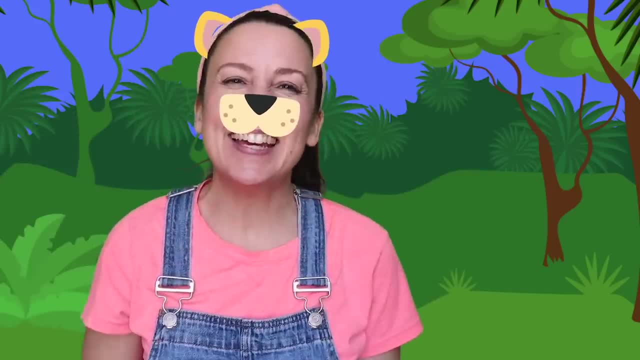 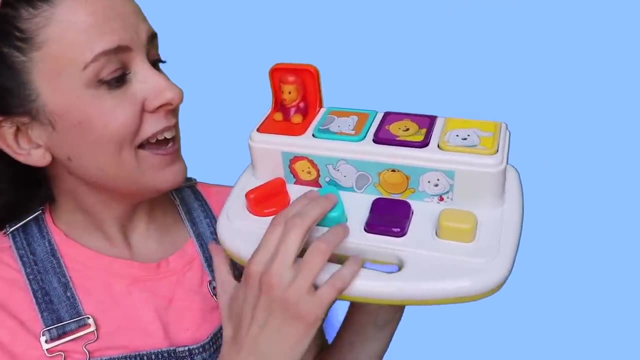 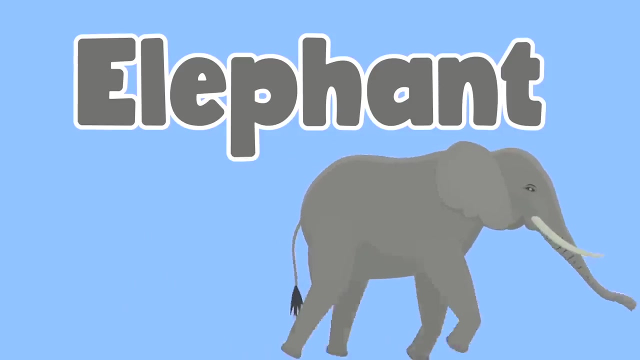 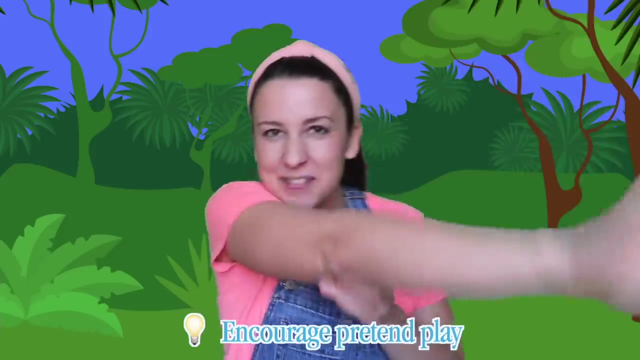 Roar A lion. Let's see who's next. Say pop, Pop. Oh, It's an elephant. Can you pretend to be an elephant with me? Elephant with a big trunk, Howoo, Howoo, We're elephants. 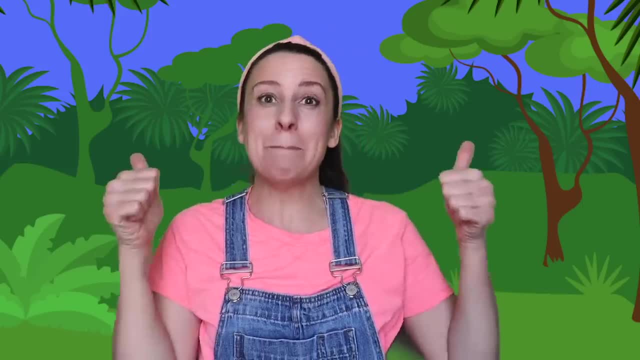 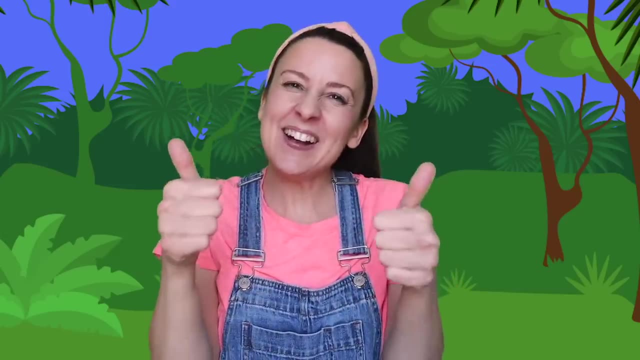 Stomp, stomp, stomp. Can you stomp like a big elephant? Stomp, stomp, stomp, Stomp, stomp, stomp. Good job, Who's next? Let's see Say pop Pop. 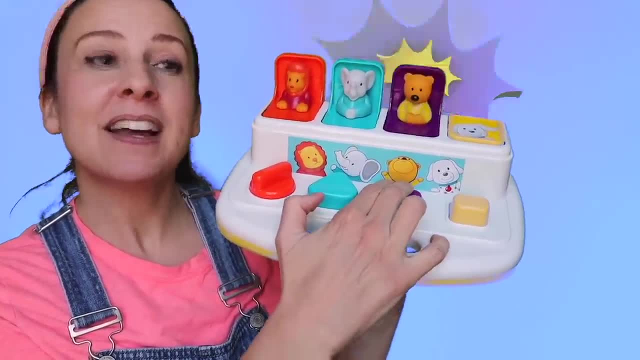 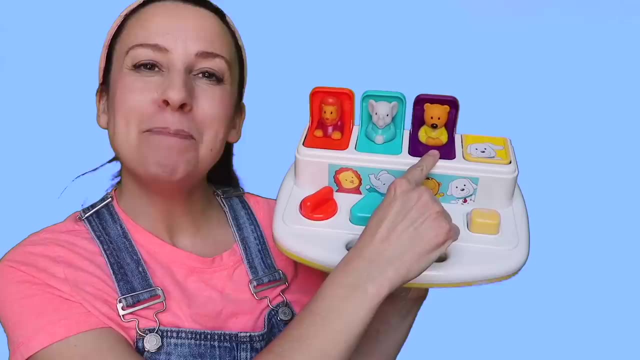 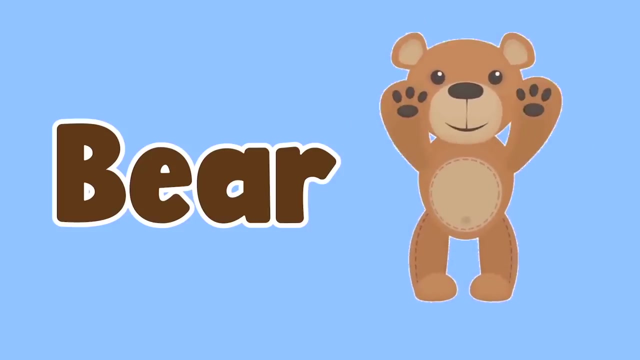 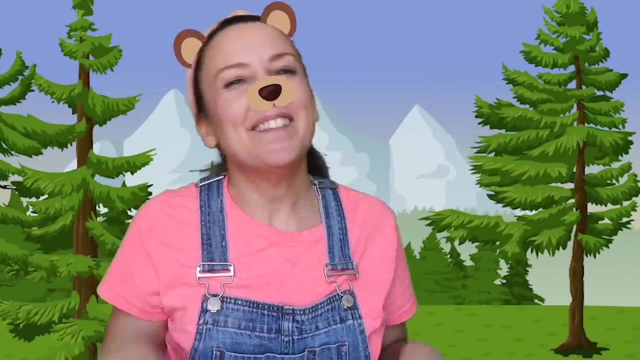 We have to say it louder: Pop, It worked. It's a bear. I see a bear. Hi bear Roar. Roar, Roar, Let's pretend to be bears. Can you pretend to be a bear, Roar? 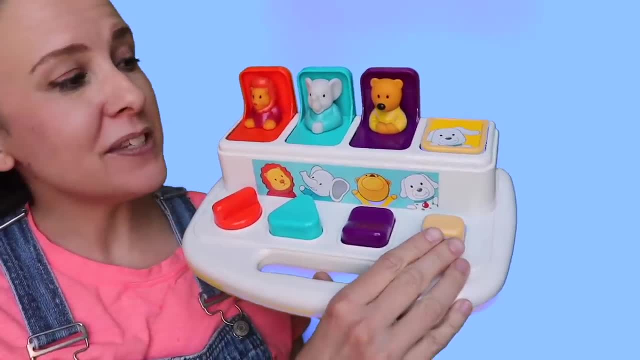 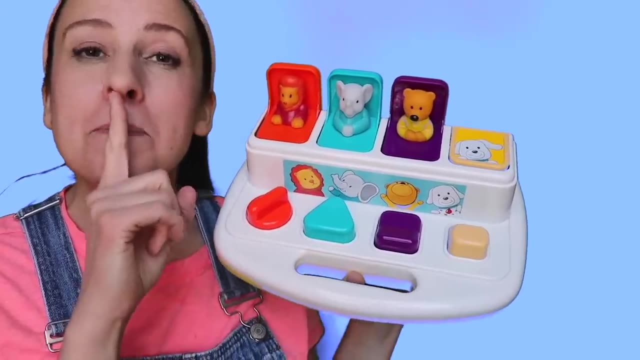 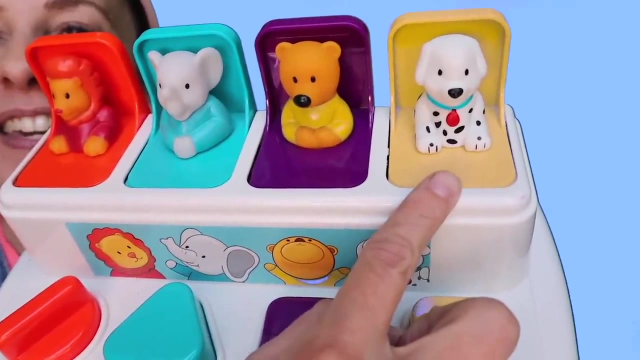 I'm a bear. Say pop, and we'll see what the last one is: Pop. Let's say it louder. Pop, It worked. Oh, It's a little doggy. Hi, doggy, It's a black and white doggy, So cute. 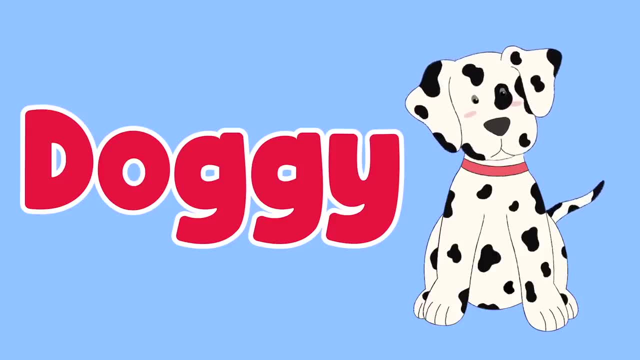 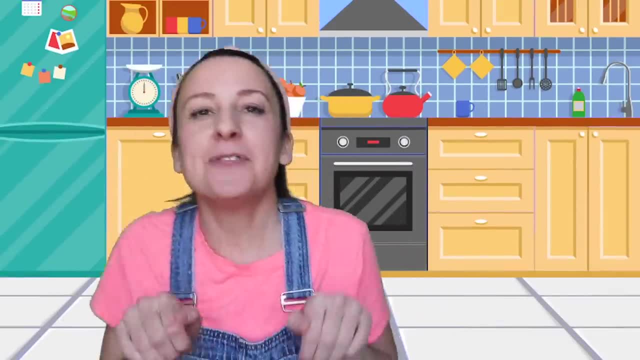 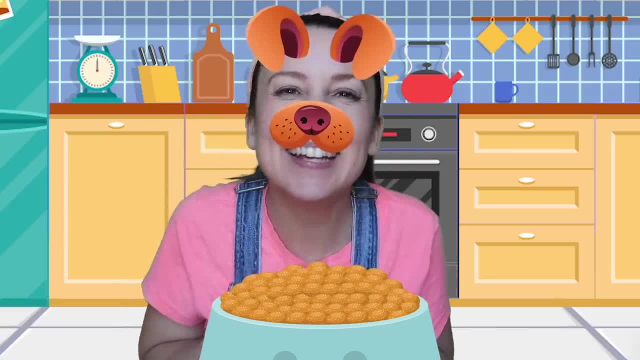 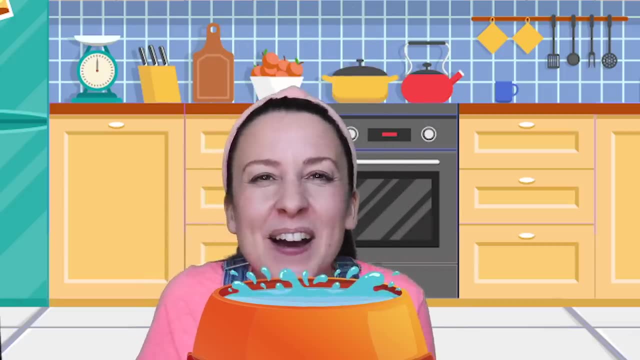 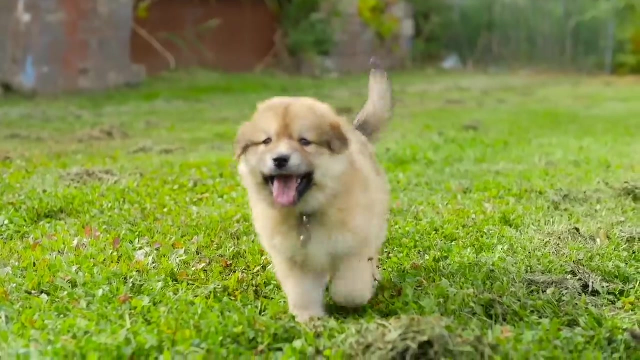 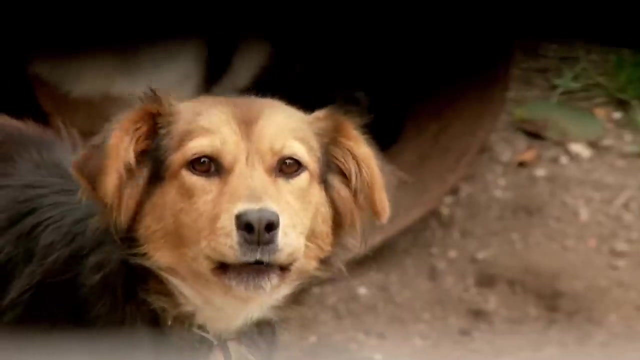 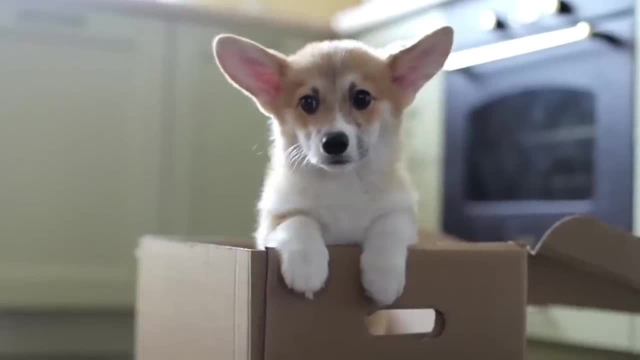 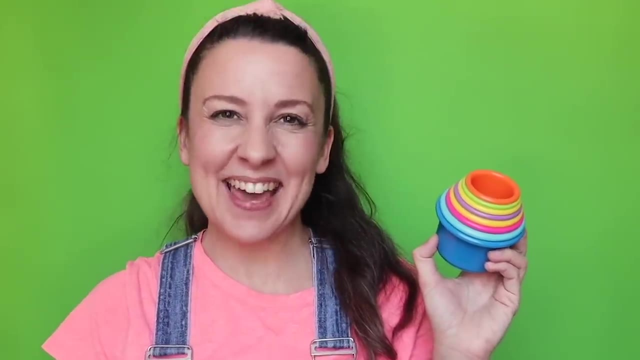 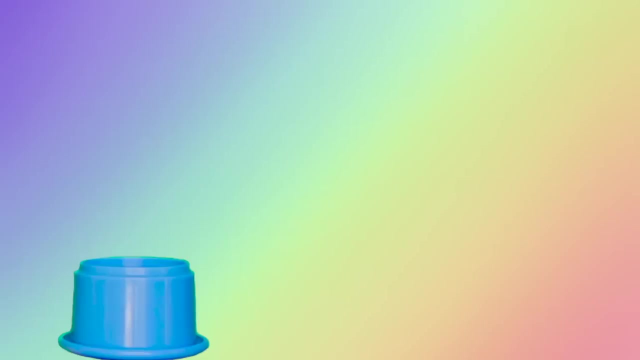 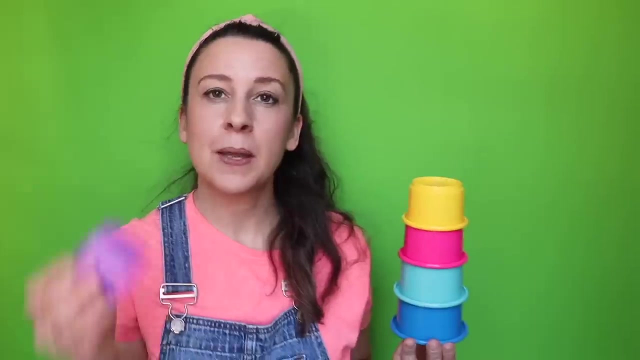 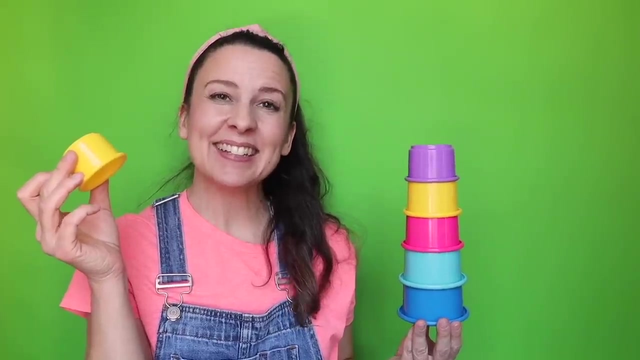 The dog in the house says woof, woof, woof, Woof, woof, All day long Nesting cups. Let's stack them Dark blue, Light blue, on Pink, on Yellow, on Purple, on Yellow again. 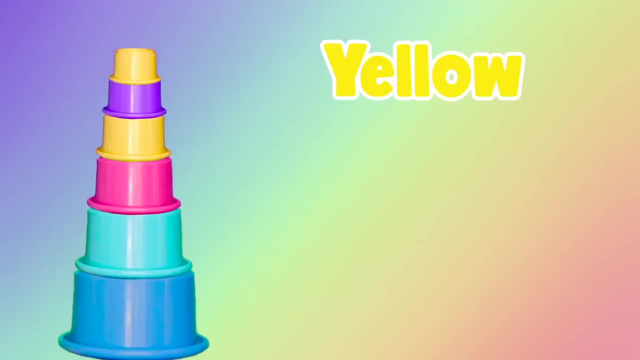 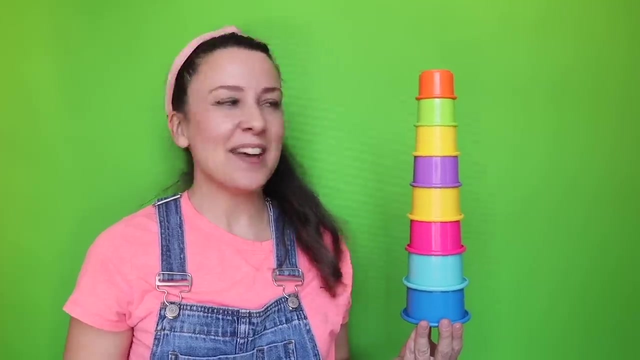 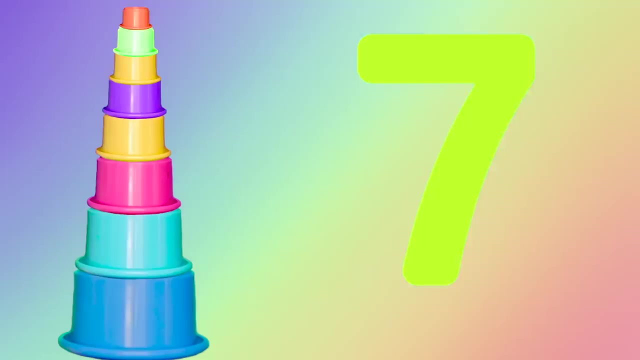 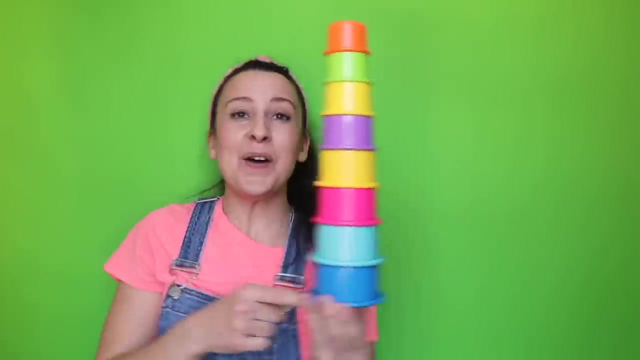 Yellow, on Green, on Orange, on. Let's count them: One, two, three, four, five, six, seven, eight. We have eight cups. Wow, Whoa, Whoa, Whoa, Whoa, Uh oh. 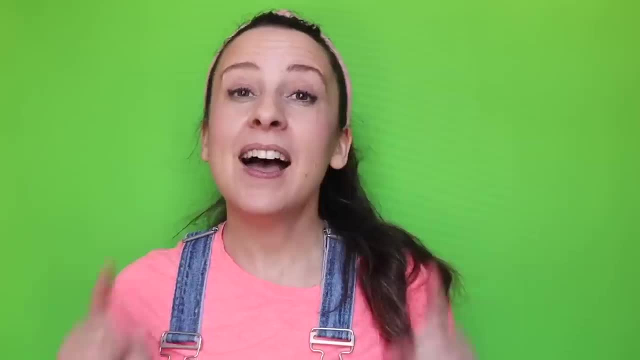 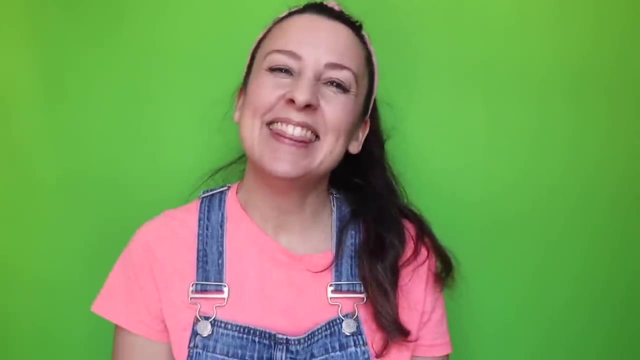 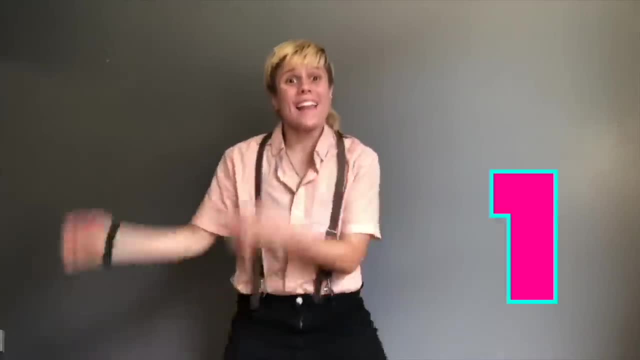 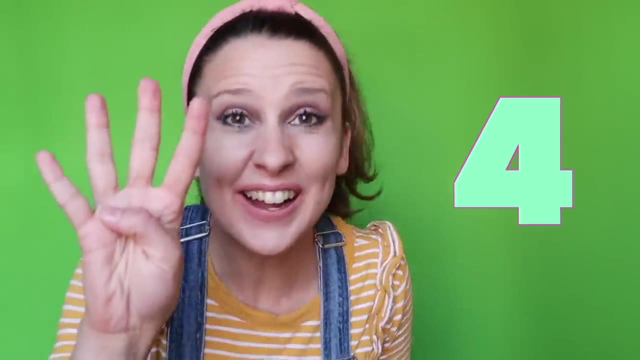 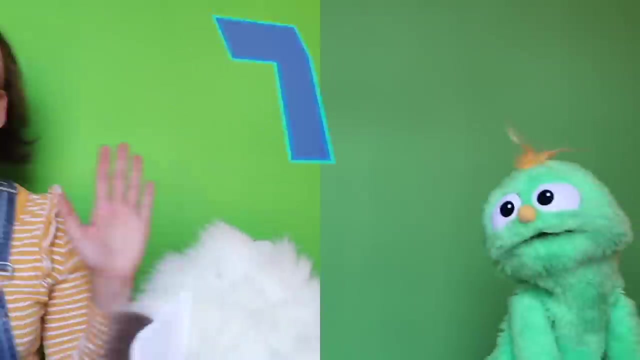 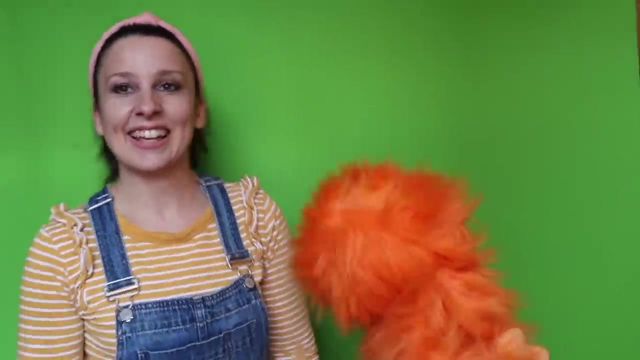 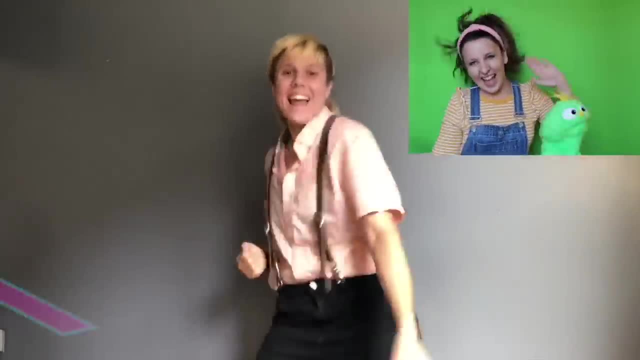 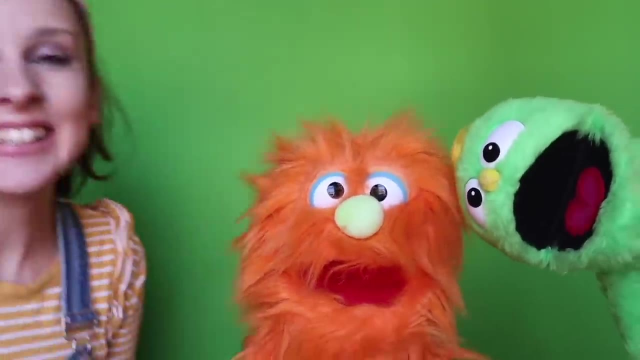 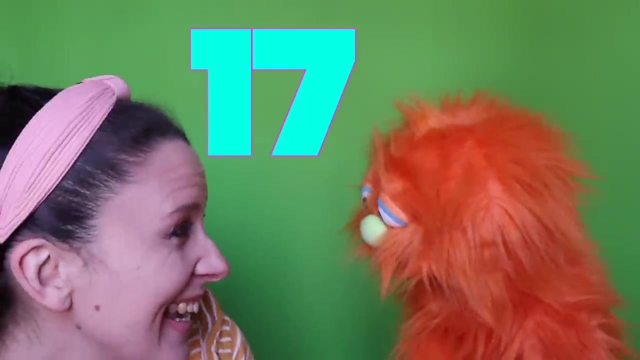 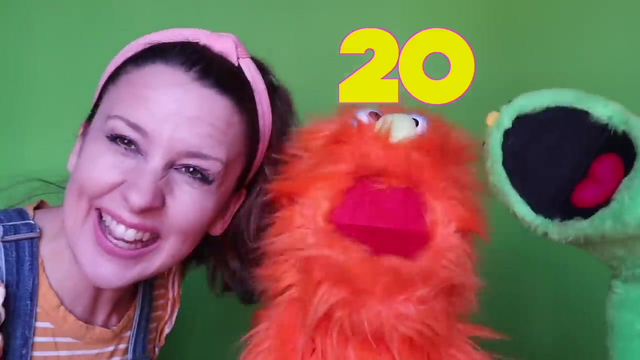 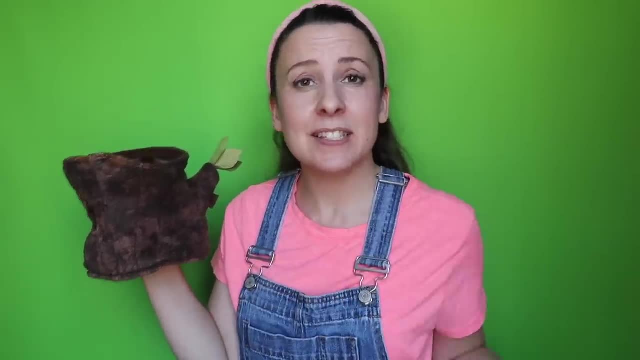 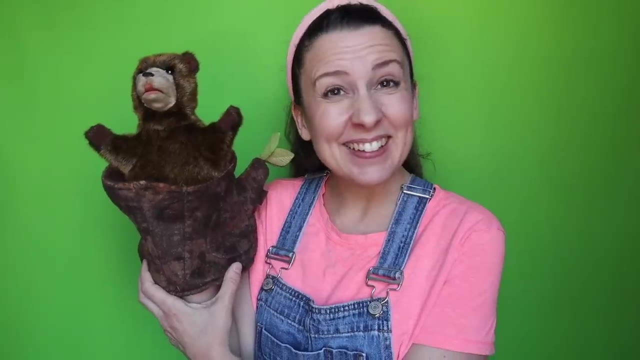 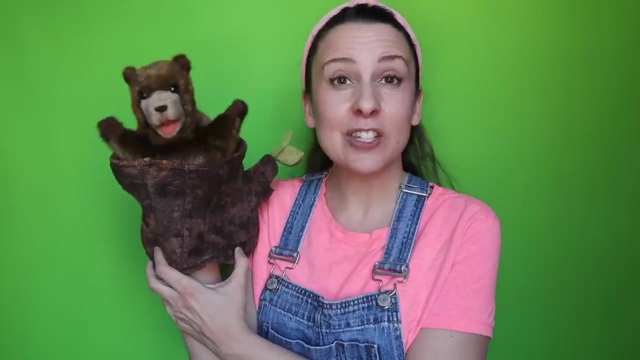 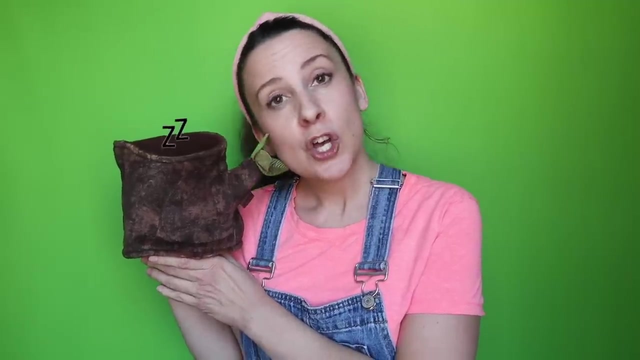 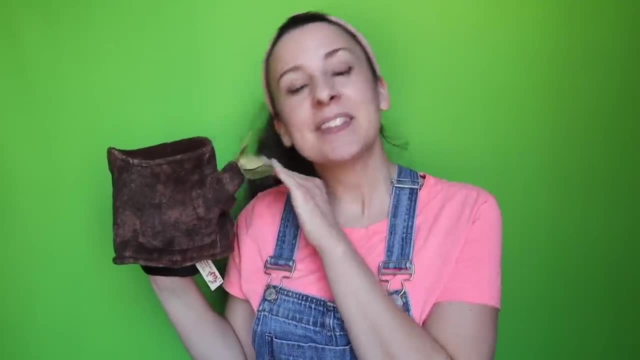 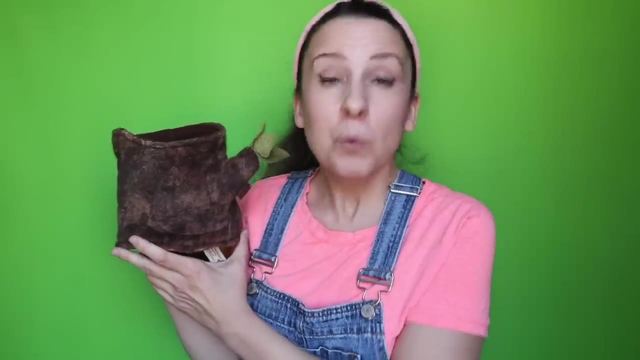 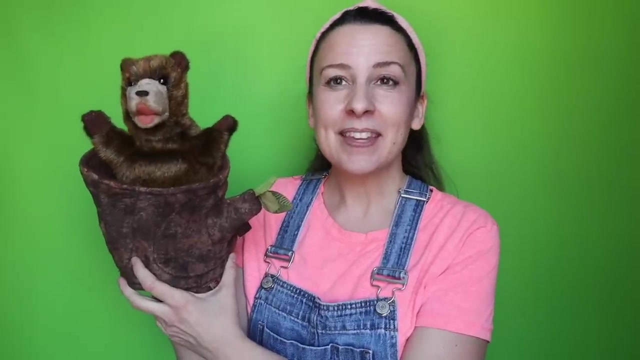 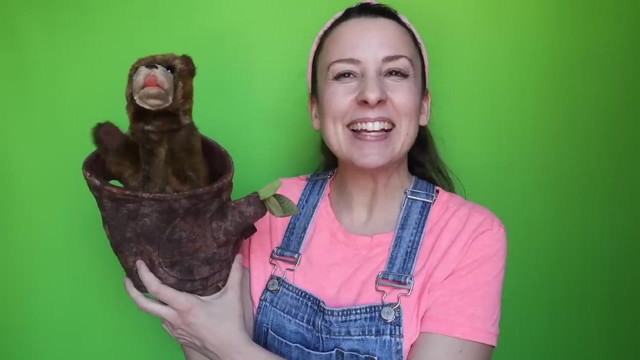 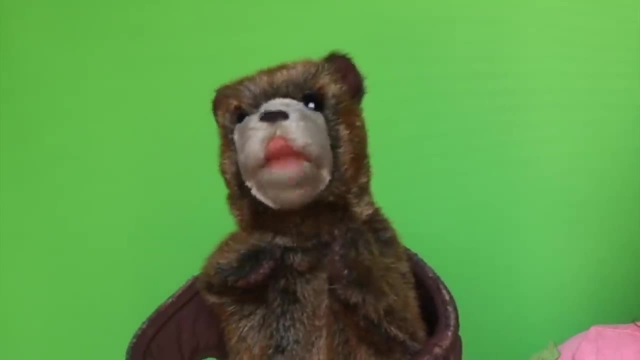 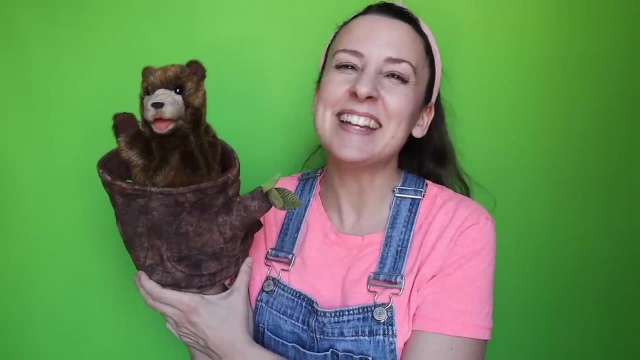 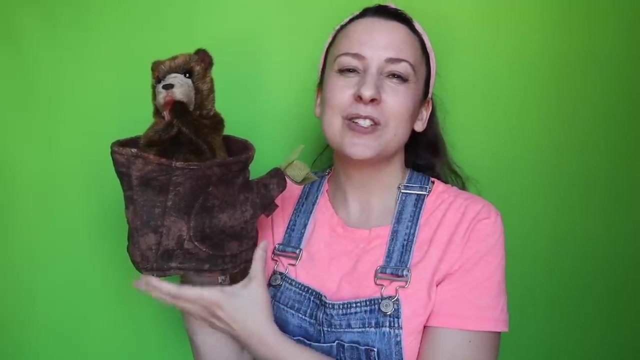 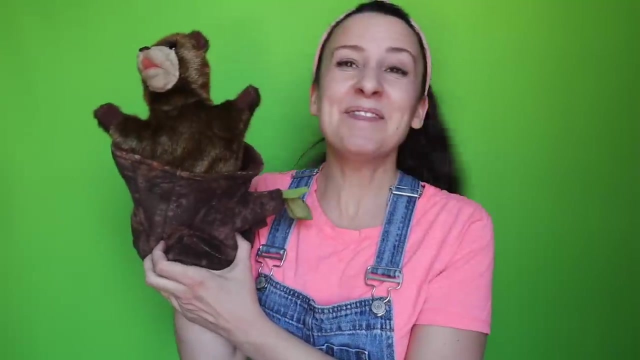 Wow, Wow, Wow, Wow. Ah, That was a big surprise. Thank you, Thanks, And thank you all so much. Thank you, Okay. Hello. I hope everyone has a wonderful day. See you guys soon. Bye, tired, Good night, Wake up, Let's go back to sleep. Oh, we're so tired. Good night. 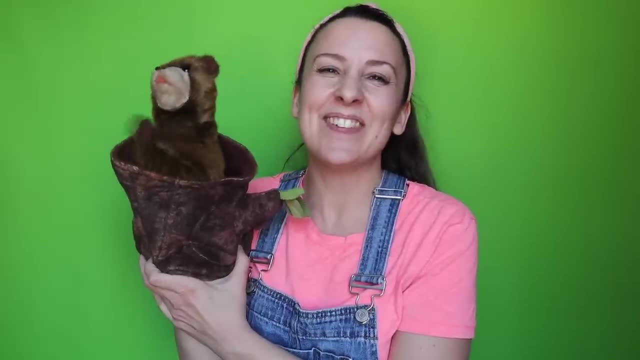 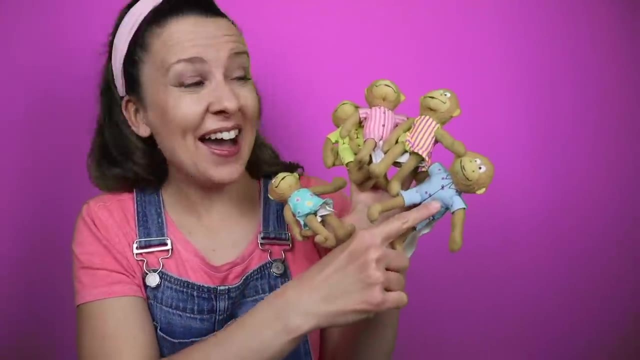 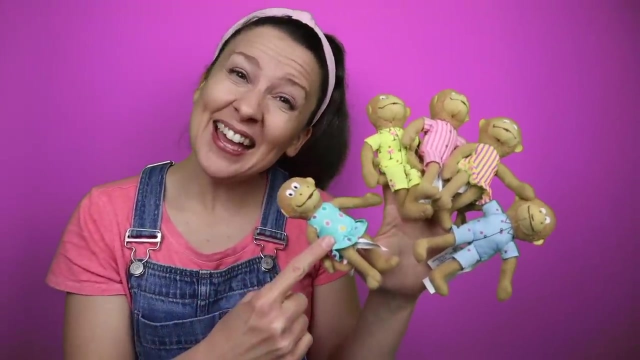 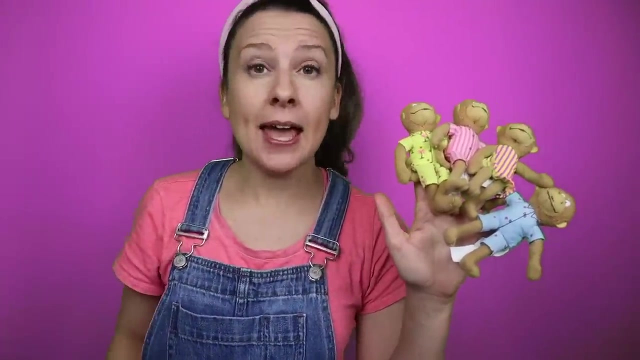 Wake up. Yay, that was fun. Good night bear, I love you. How many monkeys do I have? One, two, three, four, five, Five little monkeys jumping on the bed. One fell off and bumped his head. Mama called the doctor and the doctor said: no more monkeys jumping on the bed. How many are left? One, two, three, four, Four little monkeys jumping on the bed: One, two, three, four, Five little monkeys jumping on the bed. One fell off and bumped his head. Mama called the doctor and the doctor said: no more monkeys jumping on the bed. How many are left now? One, two, three. 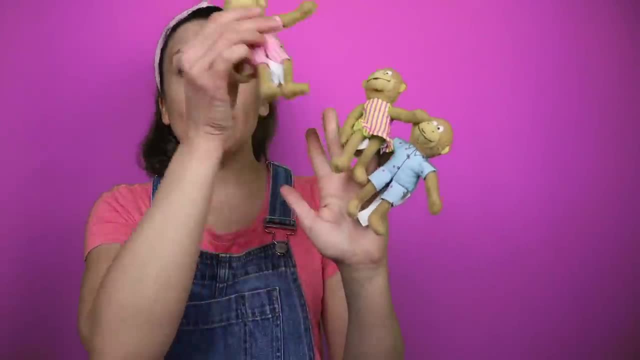 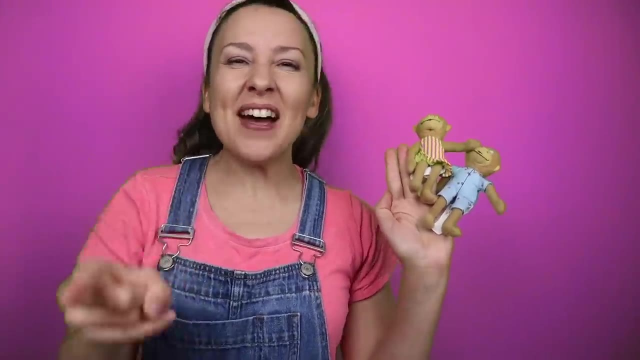 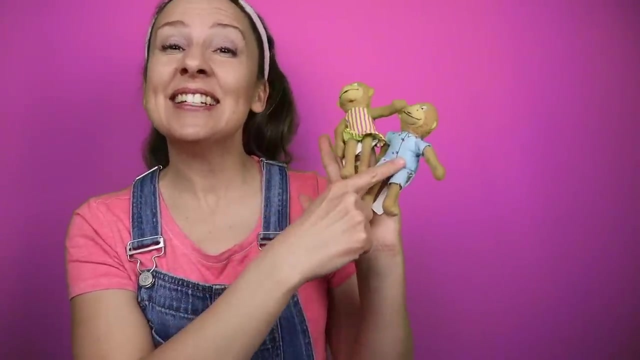 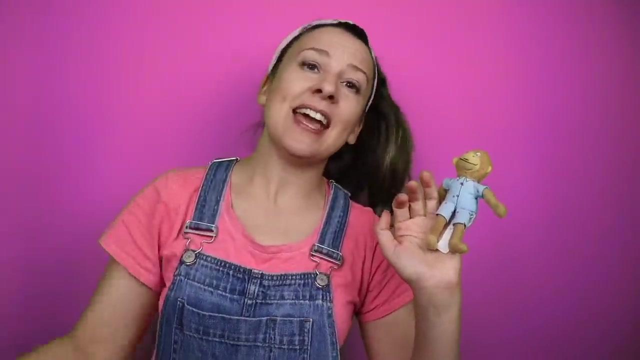 Three little monkeys jumping on the bed. One fell off and bumped his head. Mama called the doctor and the doctor said: no more monkeys jumping on the bed. One fell off and bumped his head. One fell off and bumped his head. Mama called the doctor and the doctor said: no more monkeys. 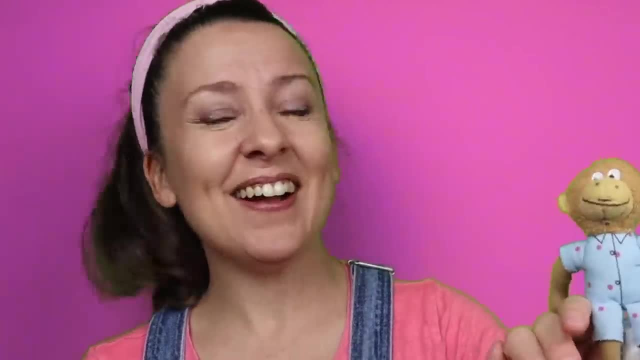 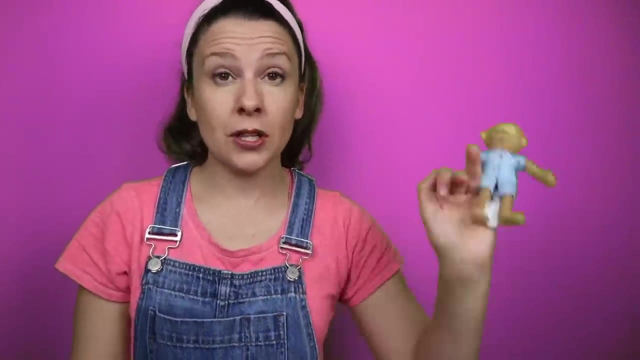 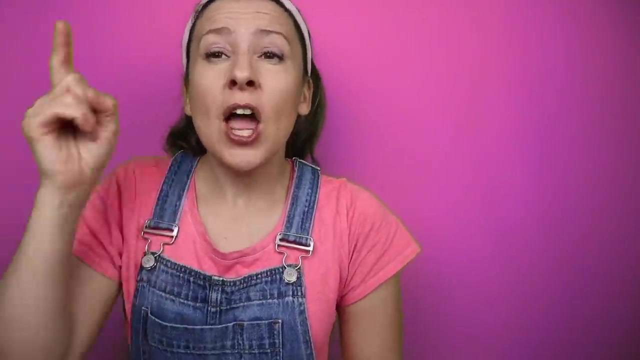 jumping on the bed. Good job, How many are left now? Just one little monkey. One little monkey jumping on the bed. He fell off and bumped his head. One fell off and bumped his head. Mama called the doctor and the doctor said: no more monkeys jumping on the bed. Let's say it nice and loud. 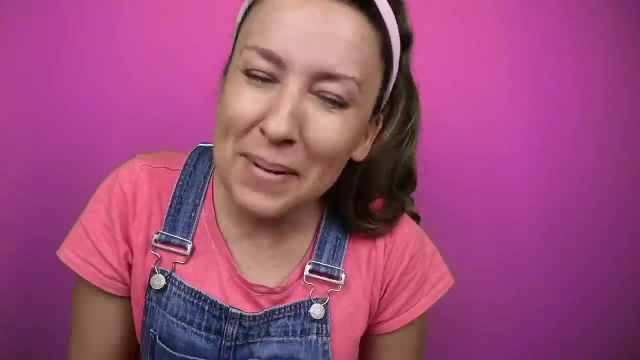 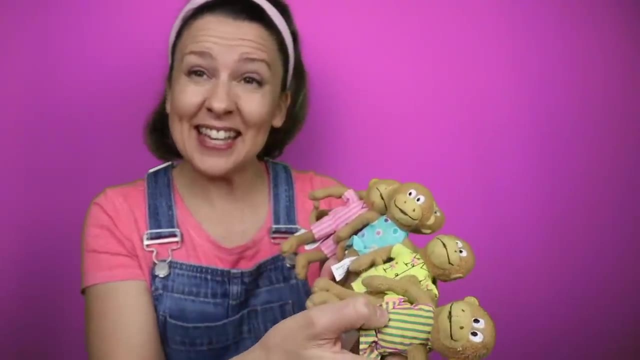 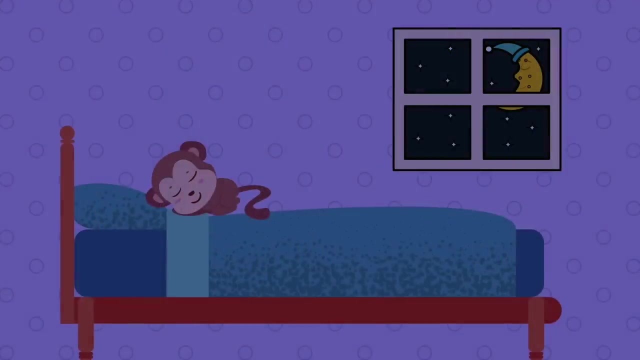 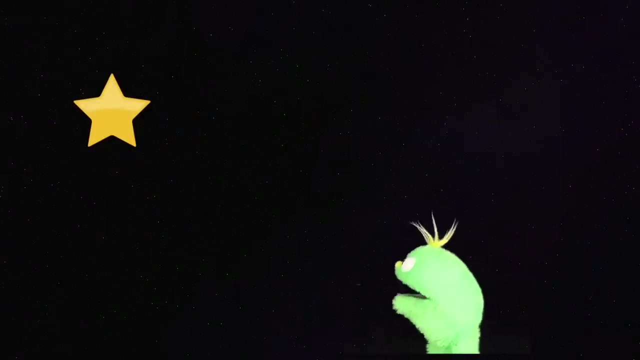 No more monkeys jumping on the bed. You did great Good job. Let's put the monkeys to sleep. Night night monkeys. No more jumping on the bed. Night night. night night monkeys, I love you. Night night Star, light star, bright first star I see tonight. 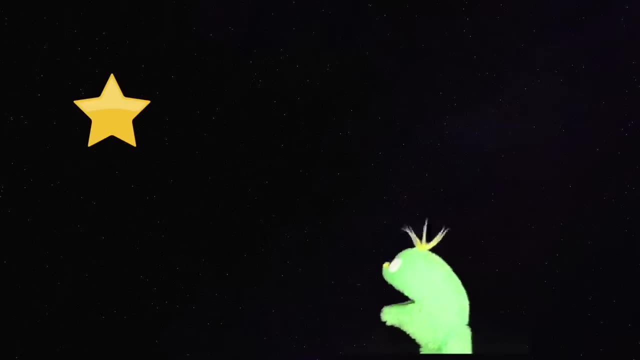 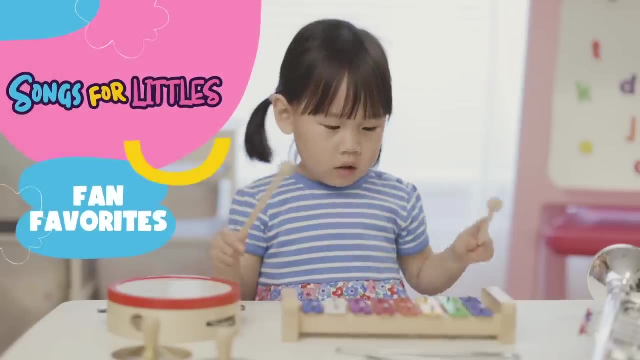 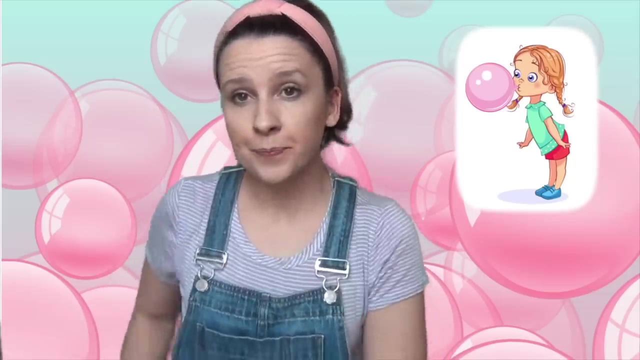 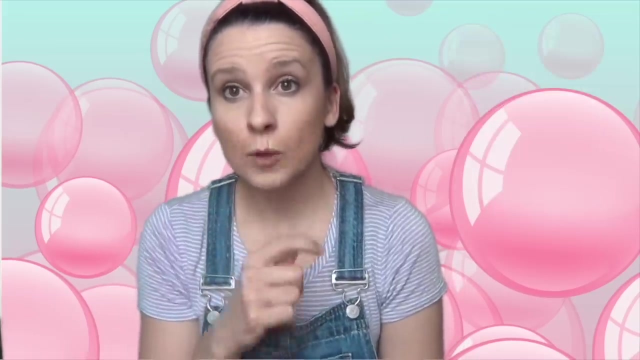 I wish I may, I wish I might have the wish I wish. tonight We're gonna get up some pretend bubble gum. Okay, so get up some pretend bubble gum. What color is yours? Mine's pink. Put it in your mouth and we're gonna chew it. 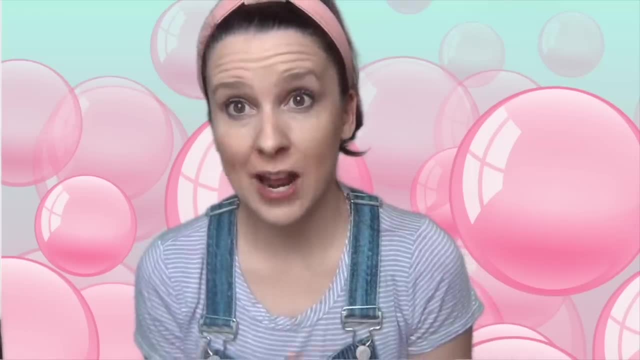 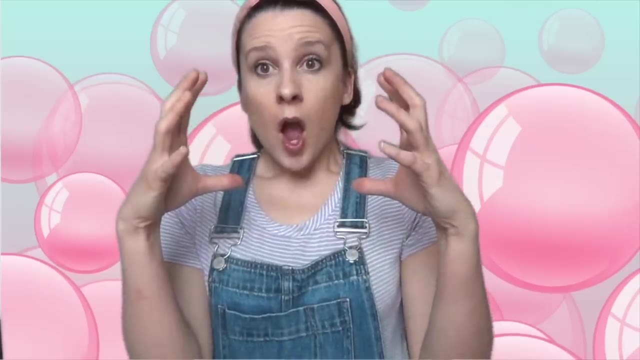 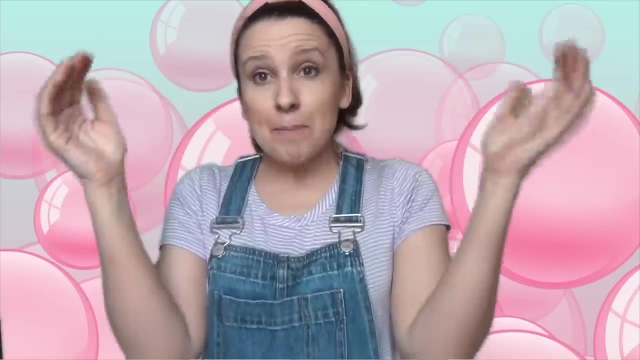 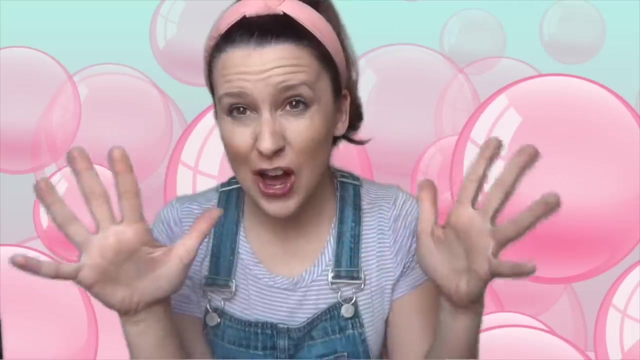 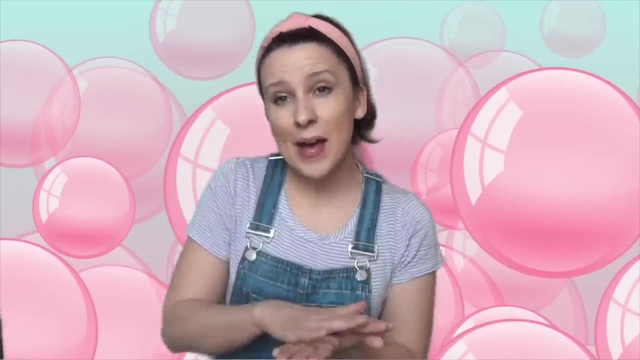 Are you chewing your gum? Okay, now we're gonna blow a really big bubble. Are you ready? Wow, Pop, Oh no, Our bubble popped And the sticky bubble gum is all over our hands. Icky, sticky, sticky, sticky bubble gum. 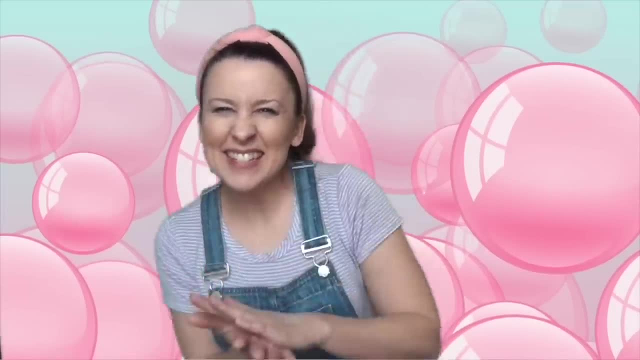 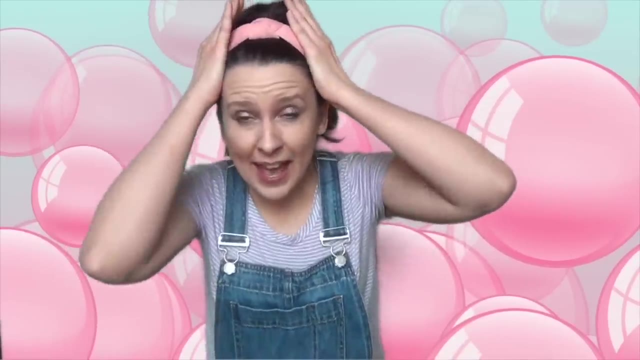 Bubble gum, bubble gum. Icky, sticky, sticky, sticky bubble gum makes your hands stick to your head And you pull them, and you pull them, and you pull them away. Icky, sticky, sticky, sticky bubble gum. 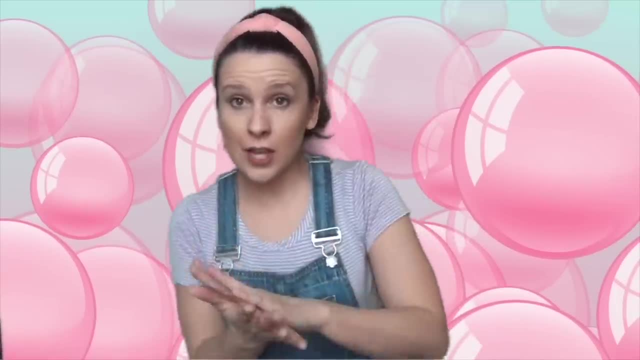 Bubble gum, bubble gum. Icky, sticky, sticky, sticky bubble gum makes your hands stick to your elbows And you pull them, and you pull them, and you pull them away. Icky, sticky, sticky, sticky bubble gum. 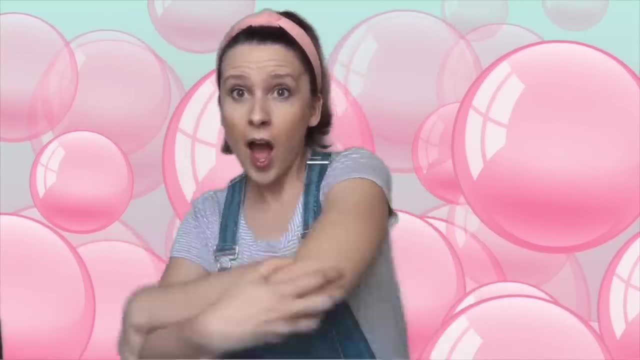 Bubble gum- bubble gum: Icky, sticky, sticky, sticky bubble gum makes your hands stick to your tummy. Bubble gum- bubble gum: Icky, sticky, sticky, sticky bubble gum makes your hands stick to your tummy. 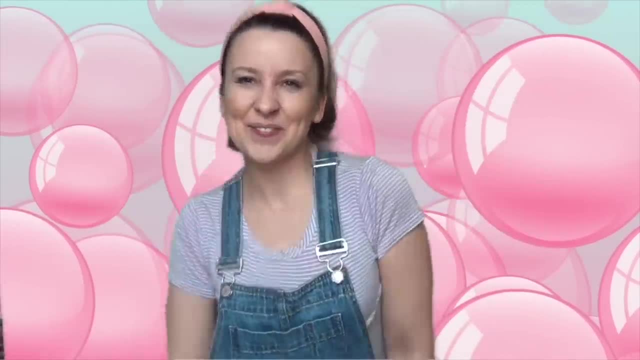 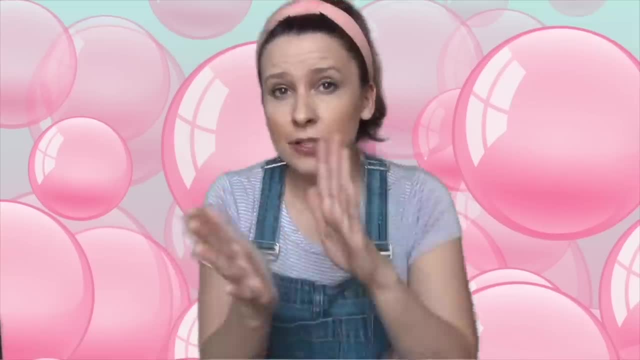 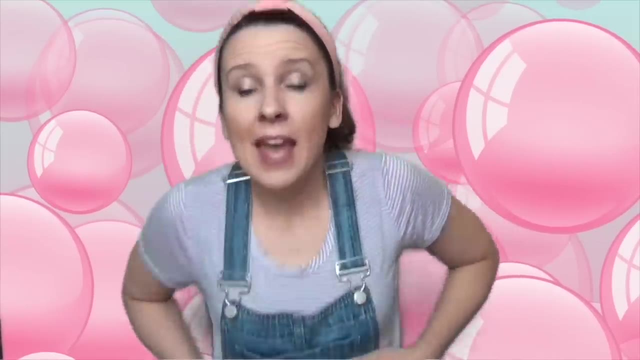 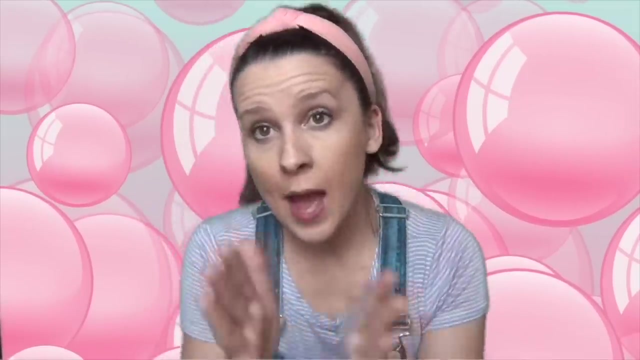 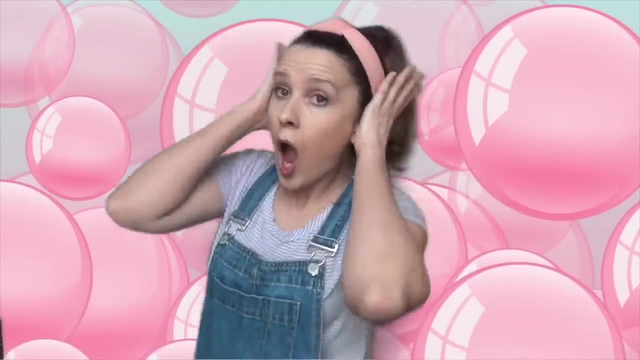 makes your hands stick to your tummy And you pull them, and you pull them, and you pull them away. Icky sticky sticky sticky bubble gum. Bubble gum. bubble gum. Icky sticky sticky sticky bubble gum. 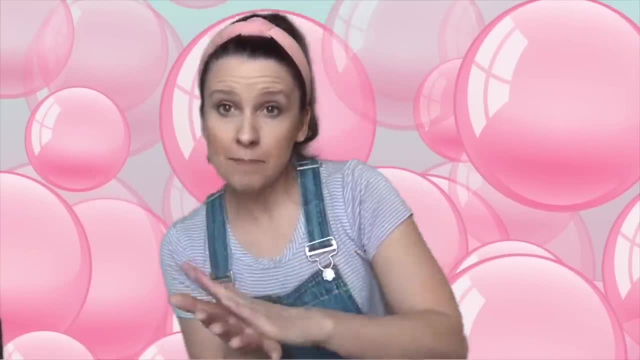 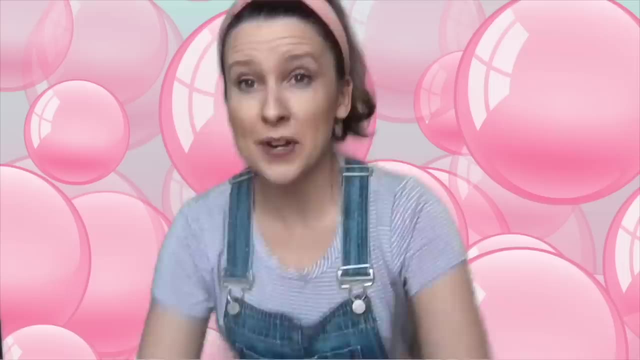 Icky, Icky, Icky, Icky Bubblegum, Bubblegum, Bubblegum. Icky, Icky, Icky, Icky Bubblegum Makes your hands stick to your knees. 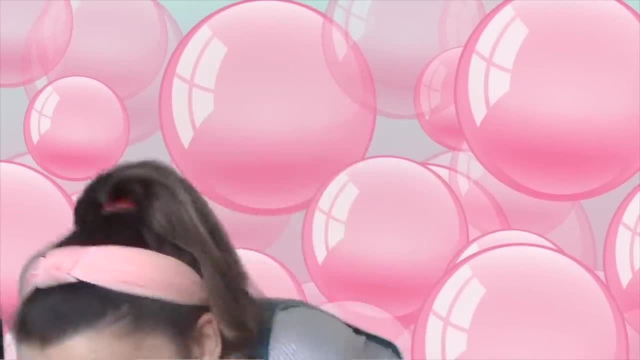 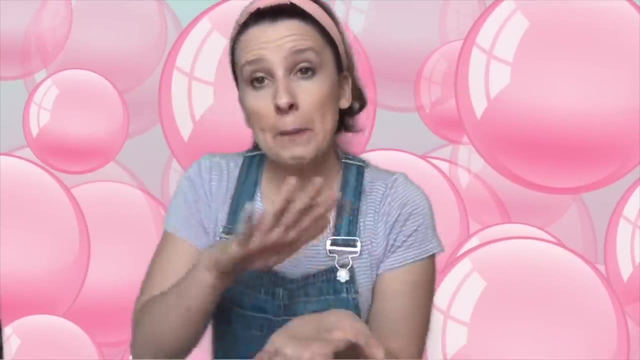 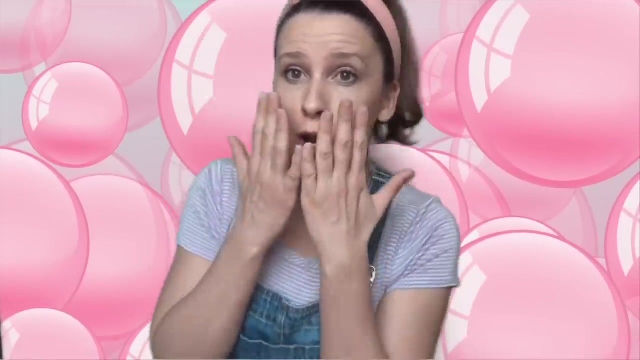 Are they on your knees? And you pull them, and you pull them, and you pull them away. Icky, Icky, Icky Icky Bubblegum, Bubblegum, Bubblegum. Icky, Icky, Icky, Icky Bubblegum. Makes your hands stick to your mouth. 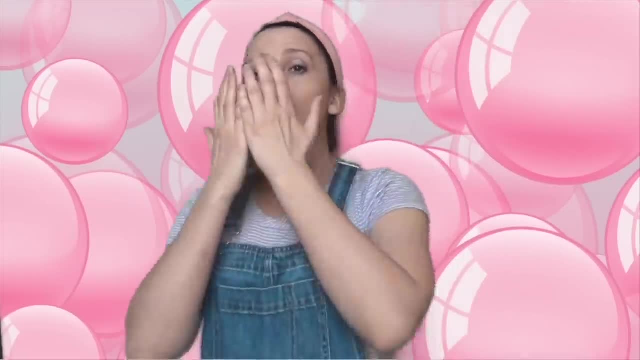 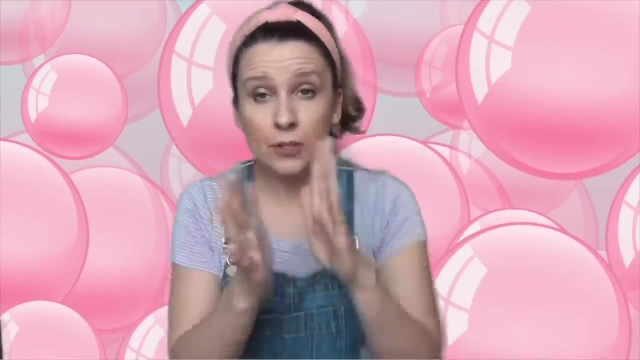 Icky, Icky, Icky, Icky Bubblegum, Bubblegum Bubblegum. Icky, Icky, Icky, Icky Bubblegum, Bubblegum Bubblegum. 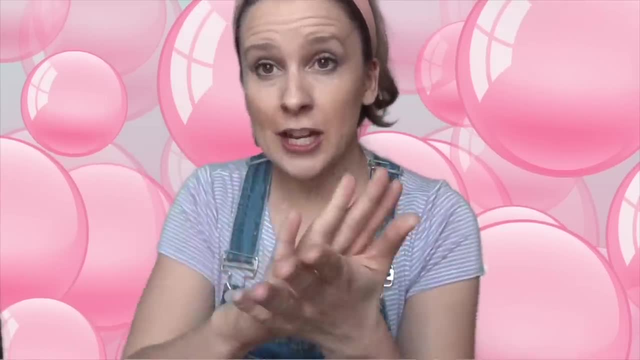 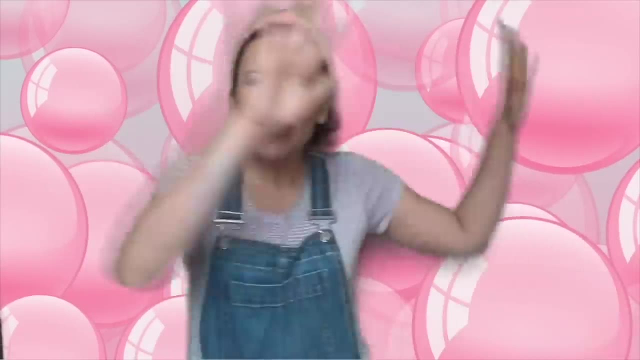 Icky, Icky, Icky Icky Bubblegum Makes your hands stick to your grown up. Put them on your grown up And you pull them, and you pull them, and you pull them away. That was so fun. One more time. 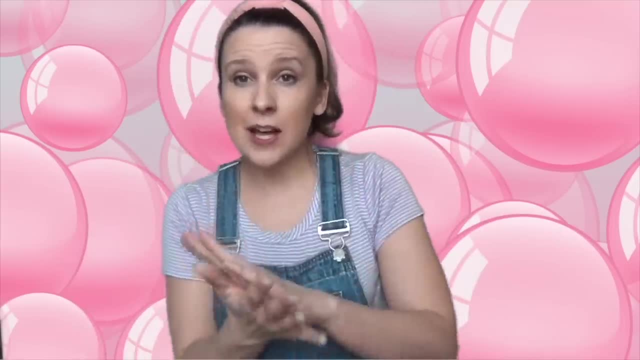 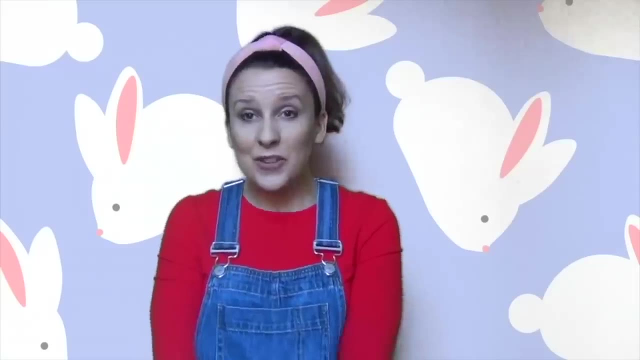 Icky, Icky, Icky, Icky, Icky Bubblegum Makes your hands stick to your Yay, That was so much fun. For this next song, we're going to sing part of it quiet. 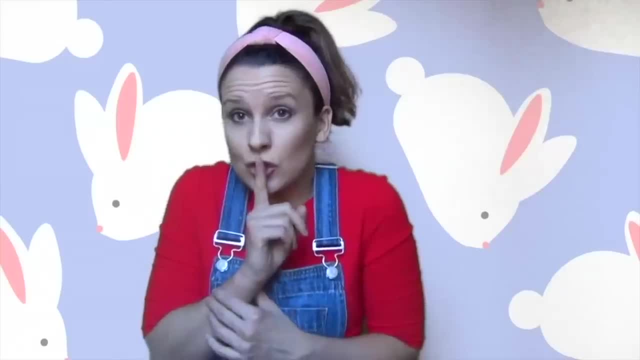 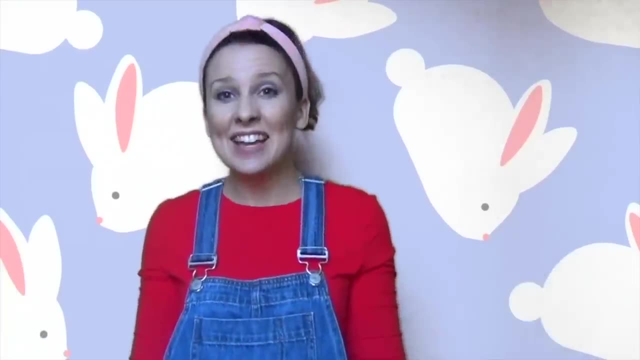 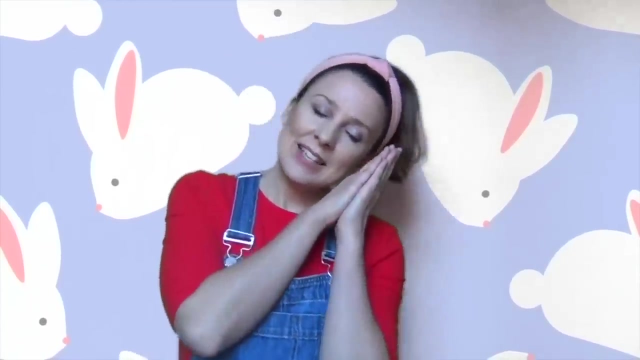 In music we call quiet piano. The next part: we're going to sing loud. In music we call that forte And we're going to pretend to be bunnies. It's going to be so much fun See the bunnies sleeping till it's nearly noon. 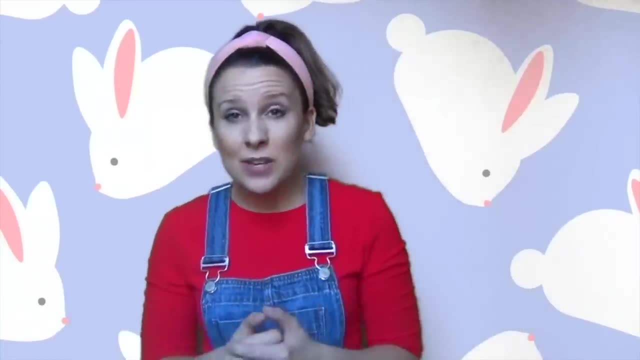 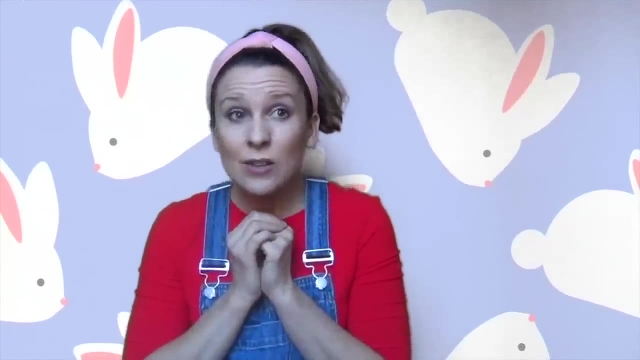 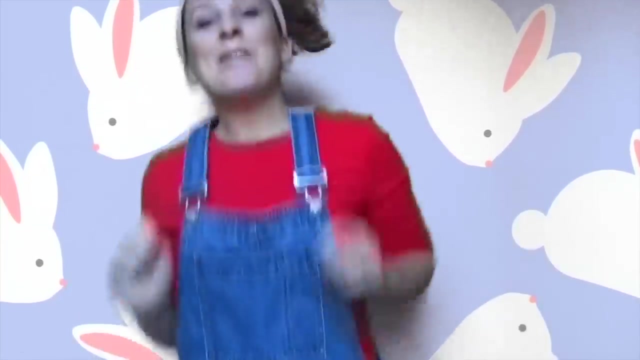 Shall we wake them with a merry tune. They're so, still are they ill. Wake up soon. This is the loud part. Wake up. little bunnies, Hop, little bunnies, hop, hop, hop, Hop, little bunnies, hop, hop, hop. 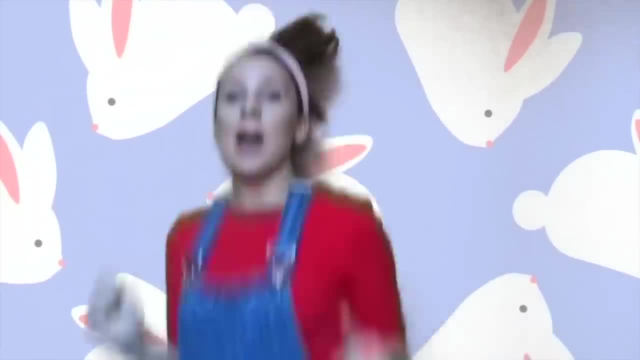 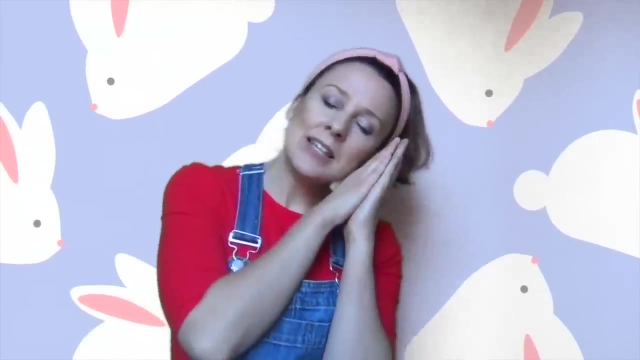 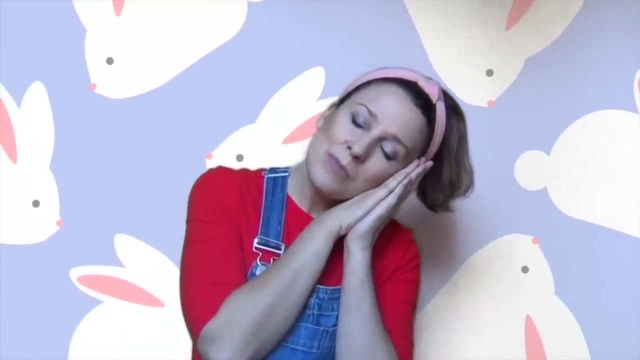 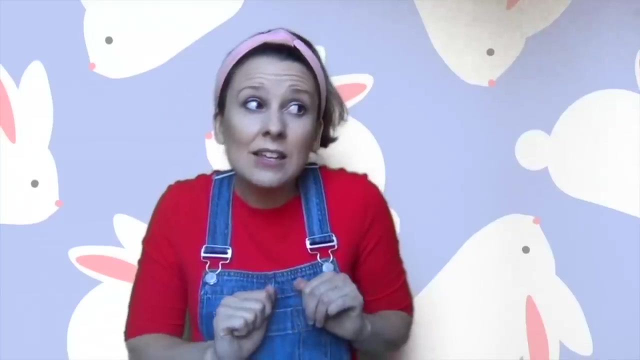 Hop, little bunnies, hop, hop, hop, Hop, hop, hop and stop. Now we're going to be quiet again. See the bunnies sleeping till it's nearly noon. Shall we wake them with a merry tune? They're so still, are they ill? 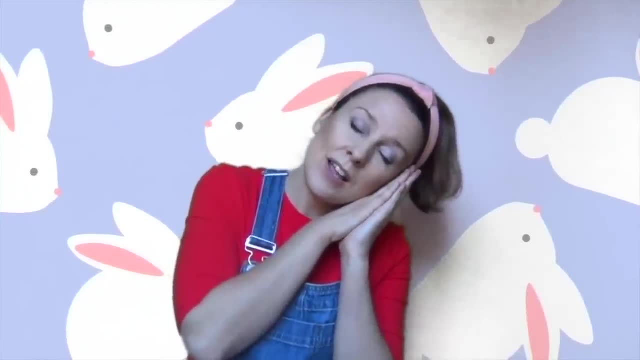 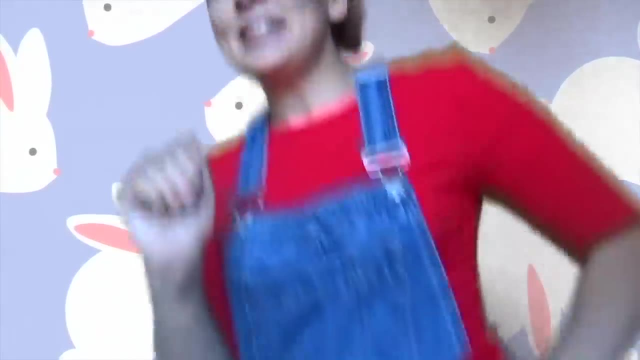 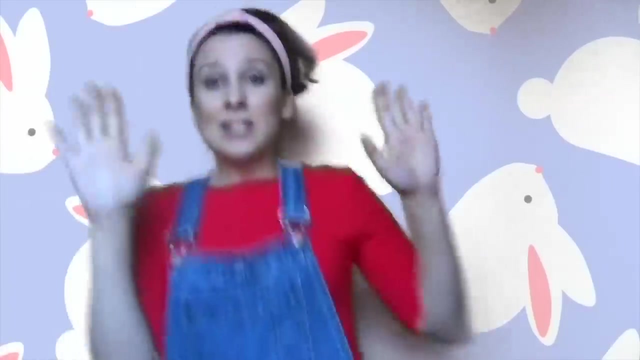 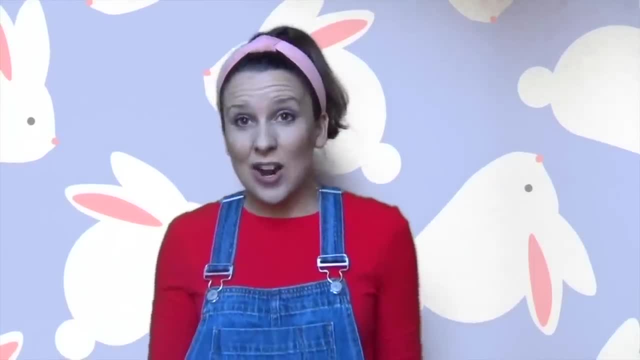 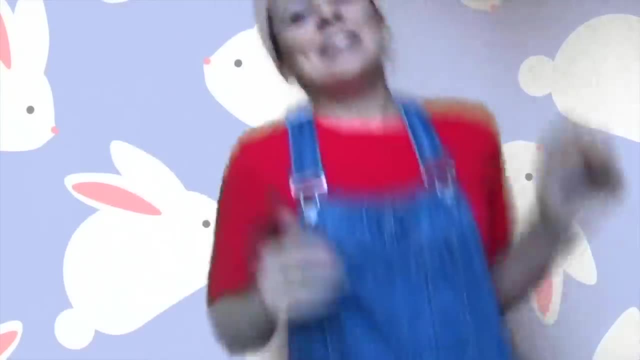 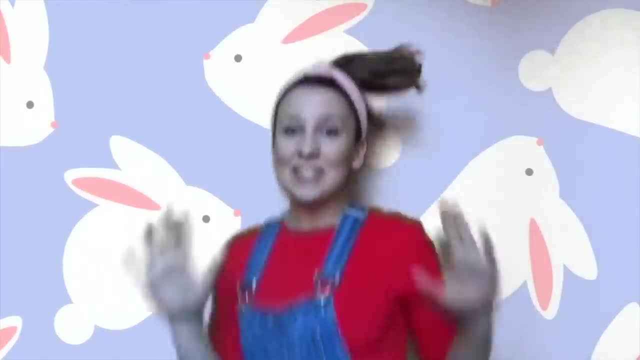 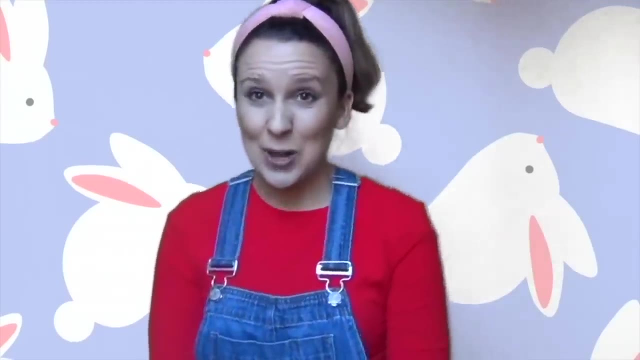 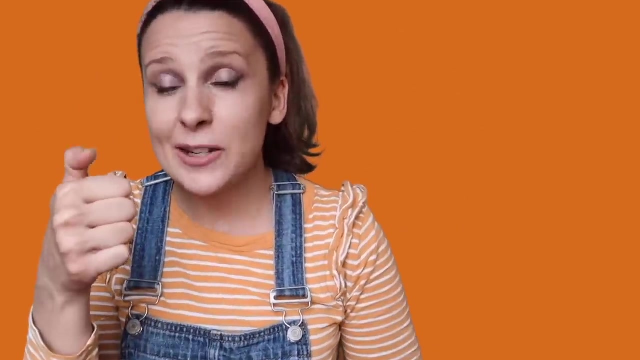 This is the loud part. Wake up soon. Hup, hup, hup and stop. Yay, Great job. Can you pretend your little thumb is a mouse? Then your other hand is going to be the house, A quiet little mouse in a quiet little house. 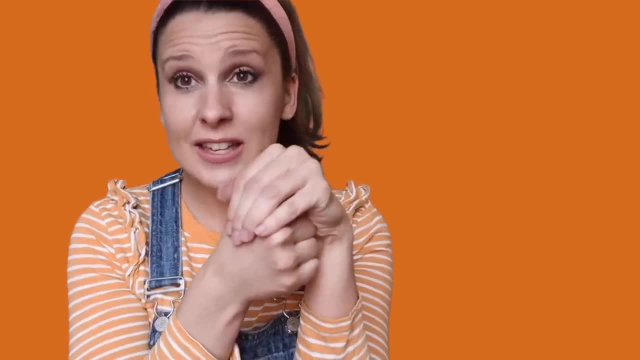 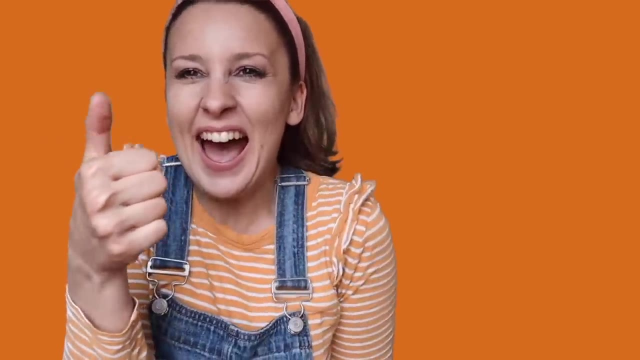 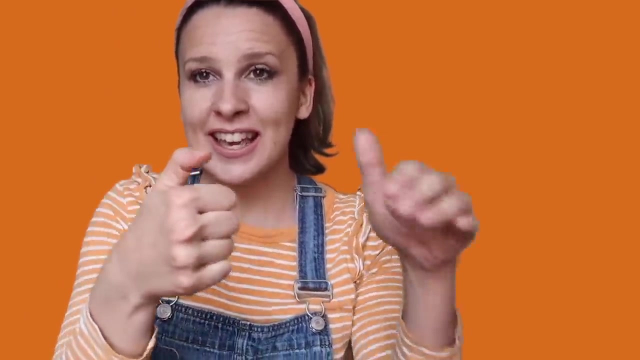 When all was quiet as quiet can be. Shh, shh, shh, Elf-bob-tee. What a silly mouse. Let's try that again. That was so silly. A quiet little mouse in a quiet little house. 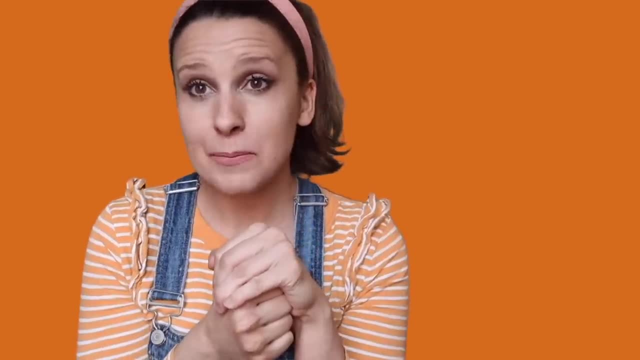 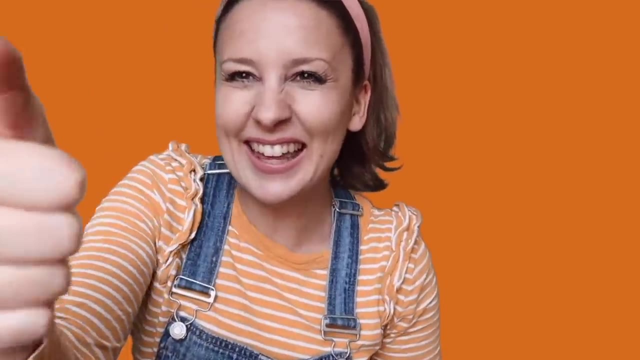 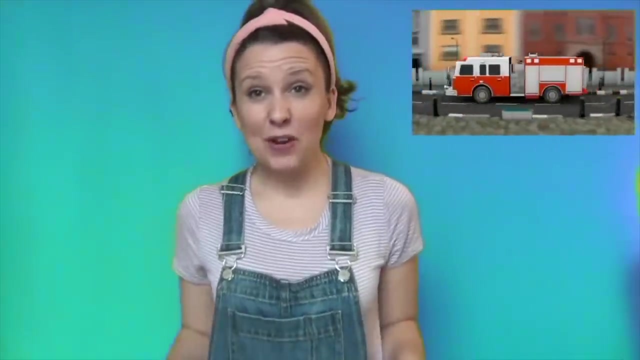 When all was quiet, as quiet can be. Shh, shh, shh, Elf-bob-tee. That was so silly. The little mouse surprised us. Good job. Okay, let's get into our firework. Are you ready? 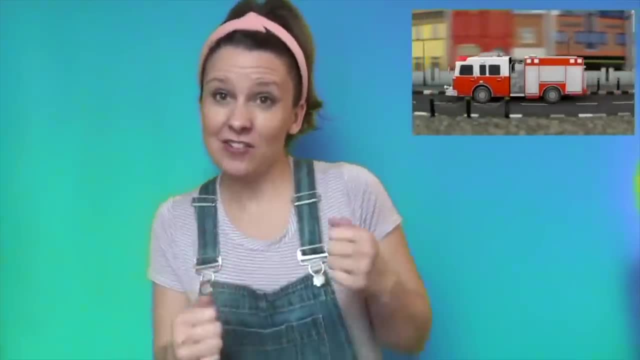 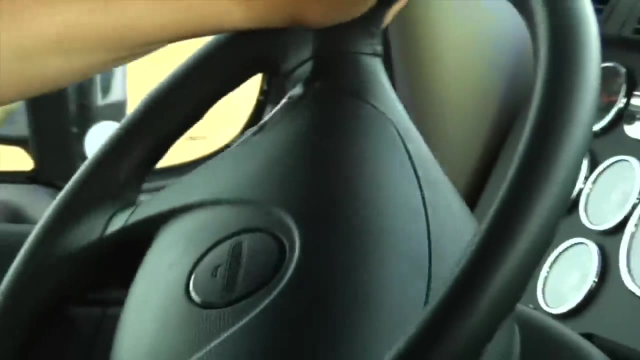 Hurry, hurry, drive the fire truck. Hurry, hurry, drive the fire truck. Hurry, hurry, drive the fire truck. Ding, ding, ding, ding ding. Now it's time to turn the corner. Hurry, hurry, turn the corner. 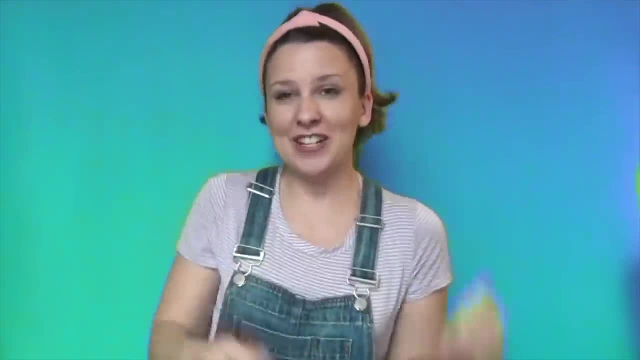 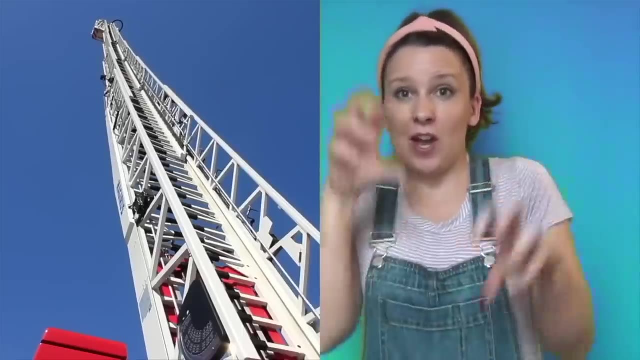 Hurry, hurry turn the corner. Hurry, hurry turn the corner. Ding ding, ding, ding ding. Now it's time to climb the ladder. Hurry, hurry climb the ladder. Hurry, hurry climb the ladder. 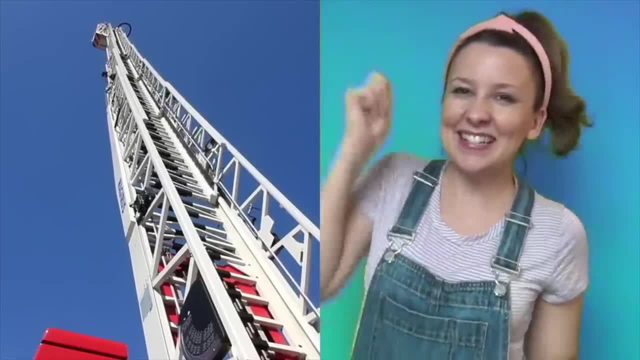 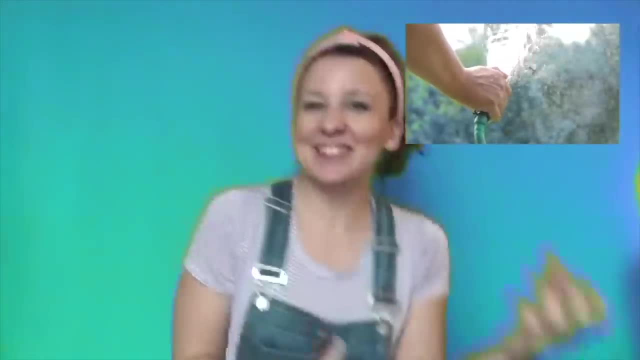 Ding ding, ding, ding ding. Get out the hose. We gotta squirt the water. Are you ready? Hurry, hurry squirt the water. Hurry, hurry squirt the water. Hurry, hurry squirt the water. 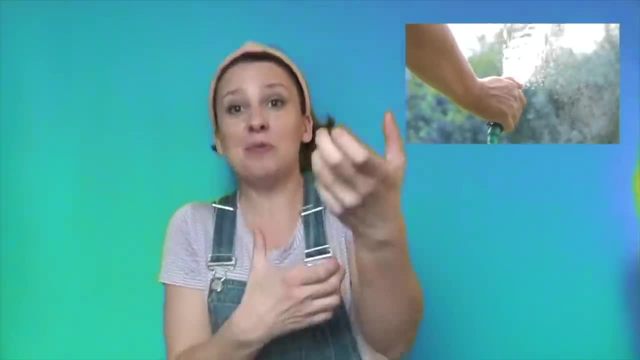 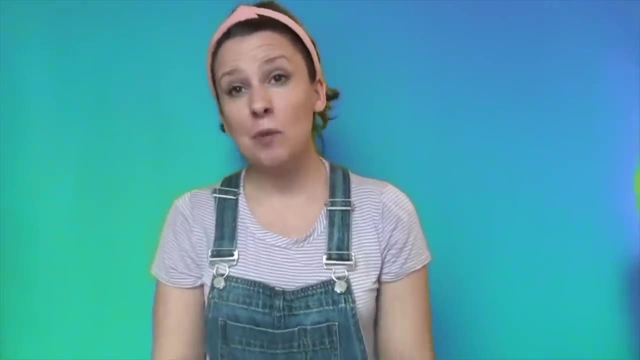 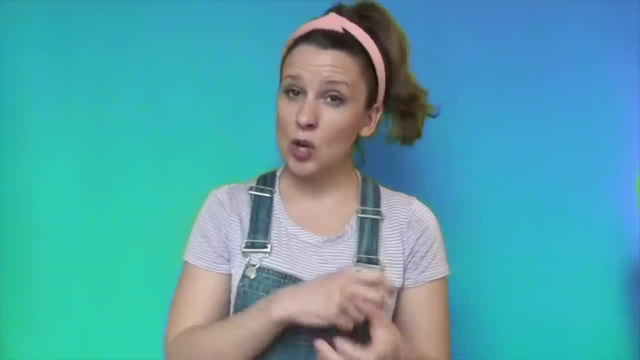 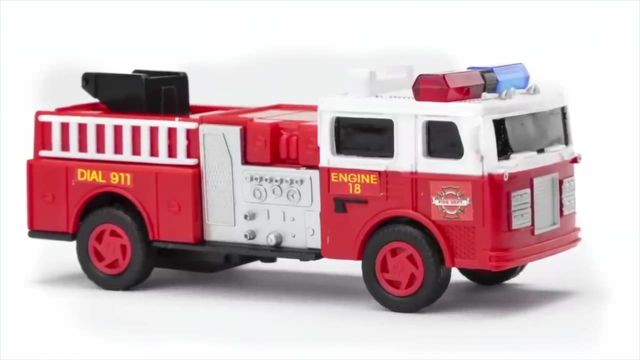 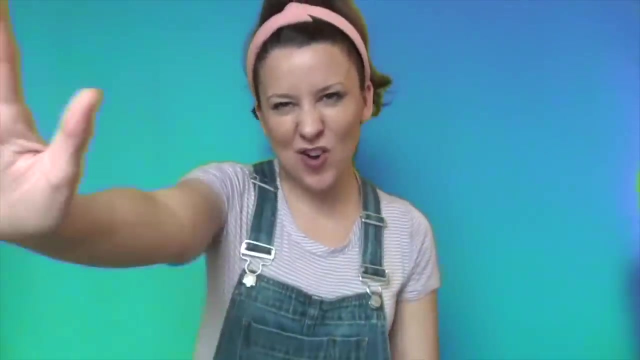 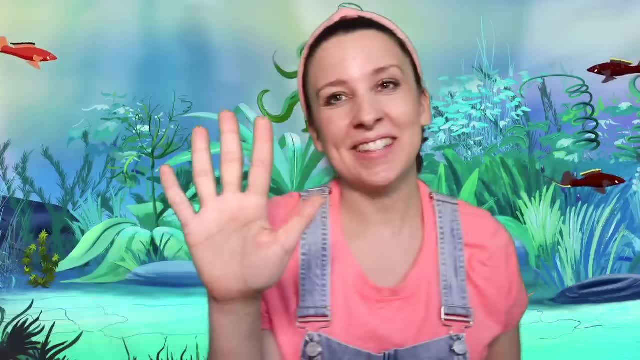 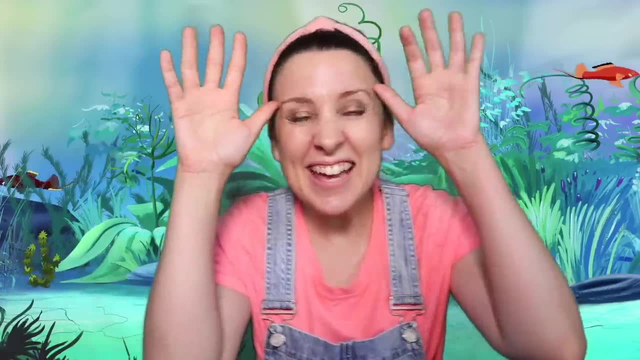 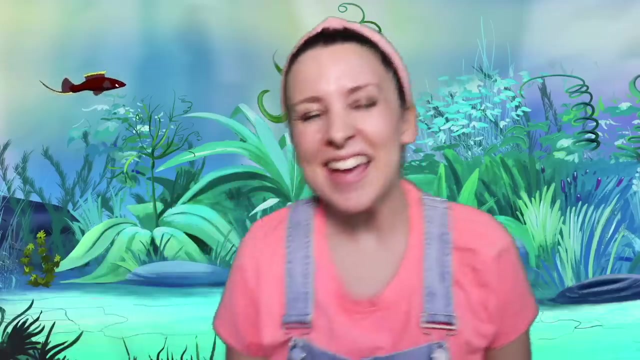 Good job. Five little fishies swimming in the sea, Teasing Mr Sharky can't catch me Along. comes Mr Sharky, quiet as can be, And snap that fishy right out of the sea. How many are left? 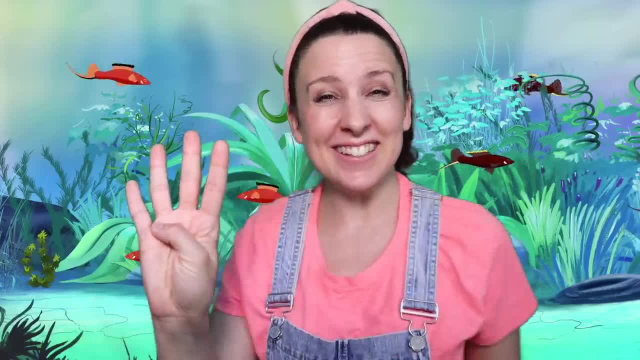 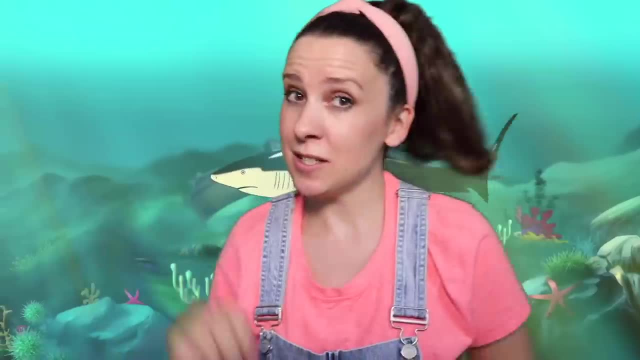 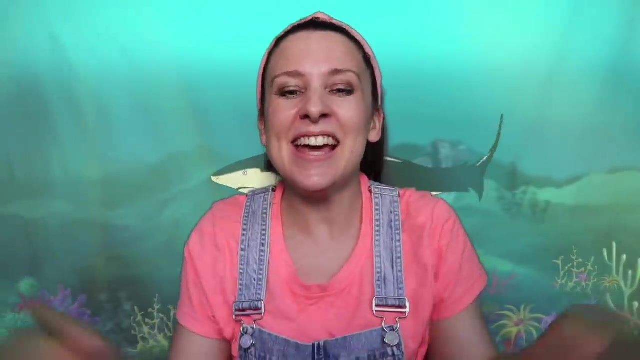 One, two, three, four, Good counting Four little fishies swimming in the sea Teasing Mr Sharky can't catch me. Along comes Mr Sharky, quiet as can be, And snaps that fishy right out of the sea. 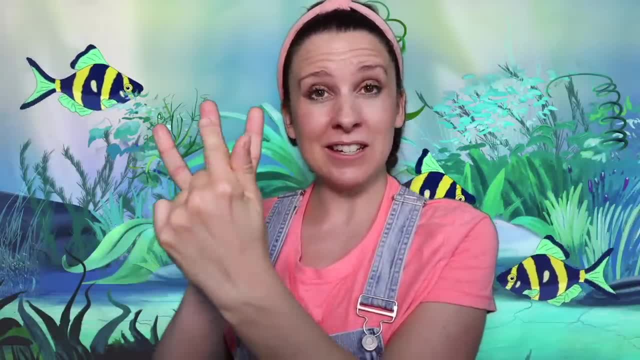 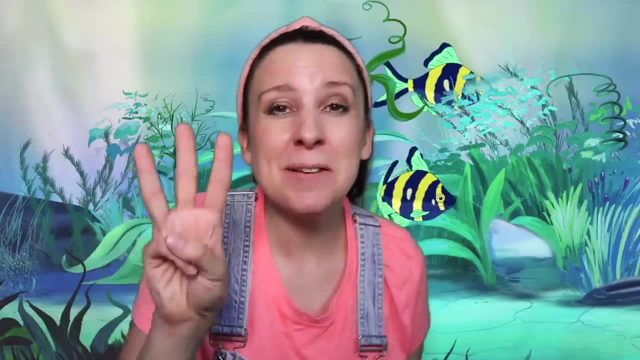 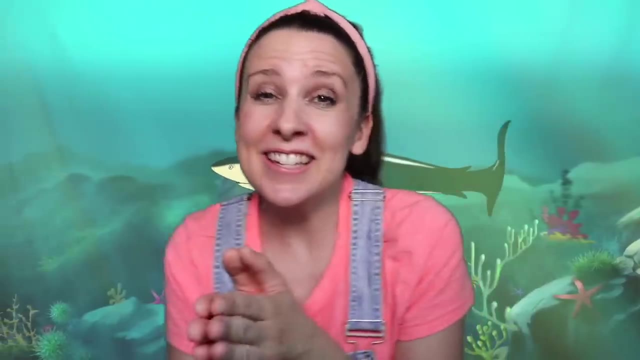 How many are left? Count with me One, two, three. Good job, Three little fishies swimming in the sea Teasing. Mr Sharky can't catch me. Along comes Mr Sharky. quiet as can be.